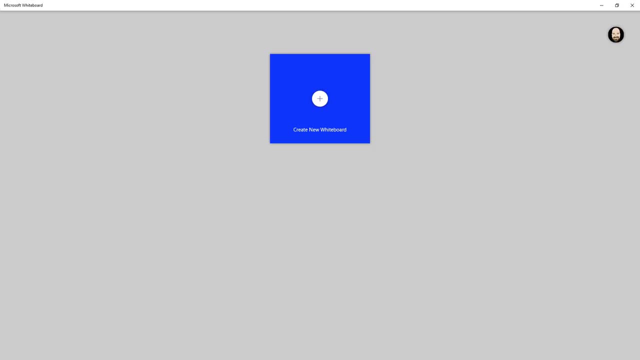 to talk about what is mediator, what is CQRS, and so on. So let's start off with CQRS. So CQRS stands for Command Query Responsibility, Segregation- all right, which is quite the mouthful Move that around, make it a little bigger. So that's CQRS: Command Query Responsibility. 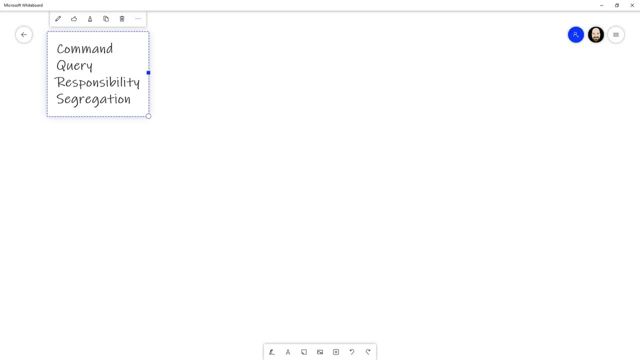 Segregation, And the idea is fairly simple. So we have normal CRUD commands. You may be familiar with the acronym CRUD, which stands for Create, Read, Update and Delete. This is how we deal with data. Well, instead of having all of our CRUD, 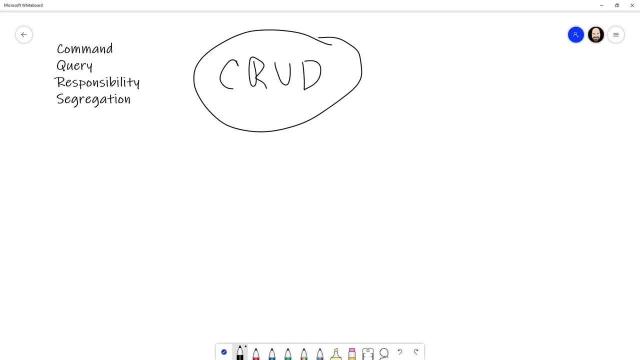 all of our CRUD kind of together. what we're going to do instead is we're going to segment it out into two different pieces And we're going to have our reads right here and our creates, updates and deletes right there. Now, what does that do for us? By creating this line here, we can 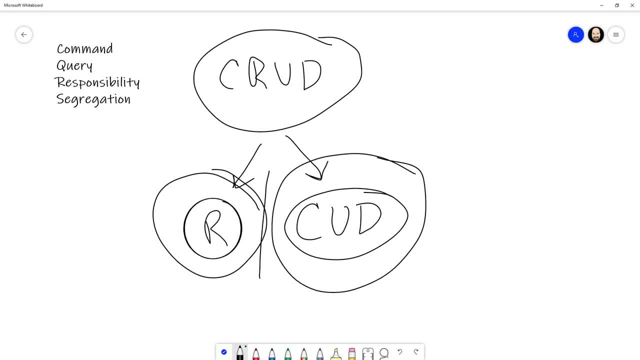 separately scale up this side or this side, So we can scale up this side, or this side, So we can do this side as necessary. So there are some benefits here, but there's also some added complexity. in doing that, We're essentially splitting our data access into two parts. 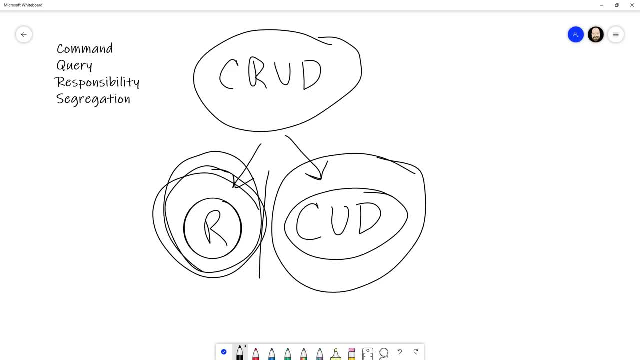 One part is all about getting data. That's this right here. The other part is all about updating data, And this is most often used in larger applications, And the rest of it is all about getting data. So we're going to have our reads right here and 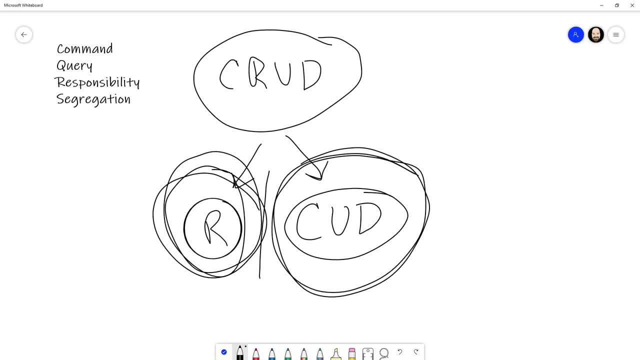 the rest of it is all about updating data, And this is most often used in larger applications. The reason why is because it adds complexity. However, it does give us some additional benefits. Like I said, we can change the read to scale up or move to a different server, or other things like. 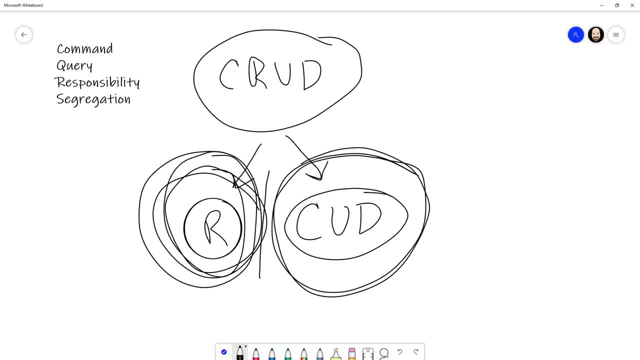 that We can scale that up separately from our creates, updates and deletes. There are two different systems for doing this. So there are some benefits to the command, query, responsibility, segregation principle or pattern. So let's now move on to. let's get rid of this. 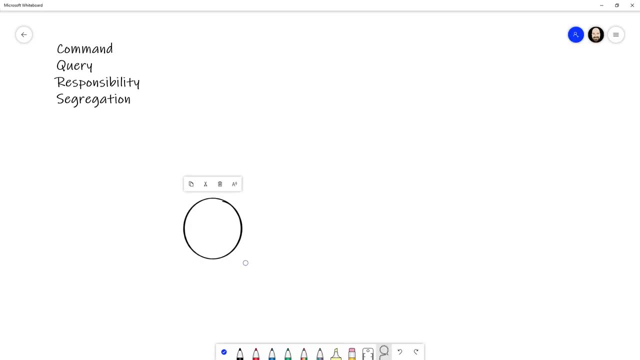 Get rid of all of it. You need to go away too. There we go. So now let's talk about our second pattern today. And whoops, there we go. That's the mediator pattern. Now notice how it's spelled. It's spelled mediator, like you normally spell it. 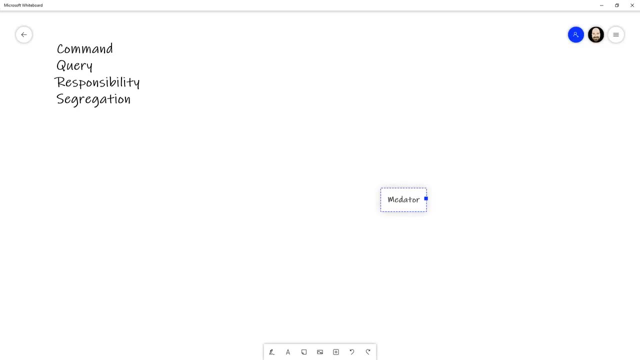 not like mediator. So now let's talk about our second pattern today. And whoops, there we go. So it's spelled mediator like you normally spell it like: mediator, the tool. So, yes, it's a little confusing, All right? So let's move that over here as well. We will make that a little bigger and 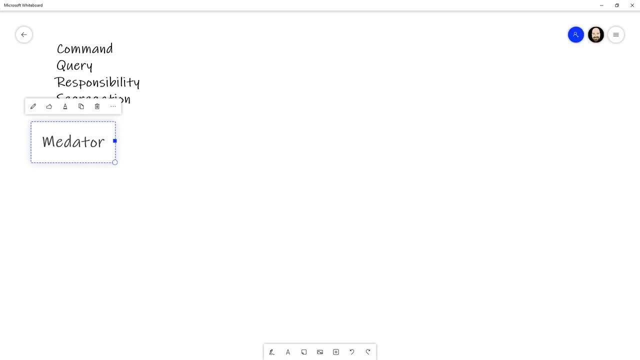 for all of those of you who love to see things crooked, we couldn't get crooked too. All right, So you have the mediator pattern as well, And the idea here is similar in nature as far as adding complexity, but also adding benefits to larger applications, And that is normally we. 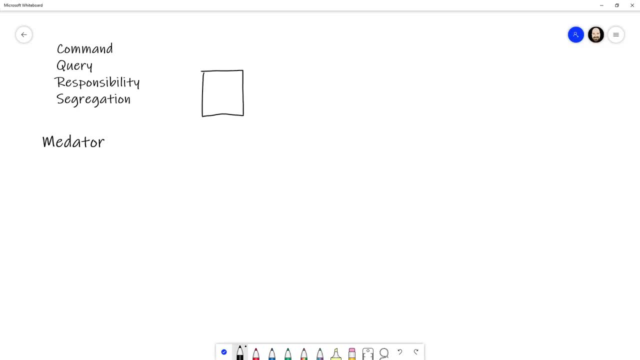 have this pattern where I have my, my front end, where it be my API or my razor application or blazer or WPF, whatever it is, and it's going to talk to my- let's keep this simple here and just say business logic, and then that's going to talk to my data access. okay, and from there we're talking. 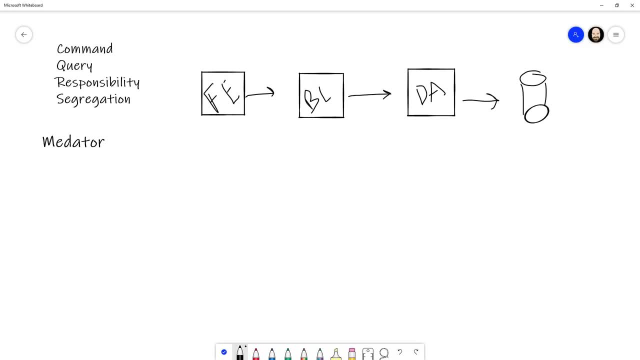 to the database. all right, that's the standard pattern for an application. if you've watched any of my applications being built, this is the pattern. you see. this is a very clean and simple way of building applications. you have some segmentation and separation but at the same time, there's not a lot of complexity. now what we have. 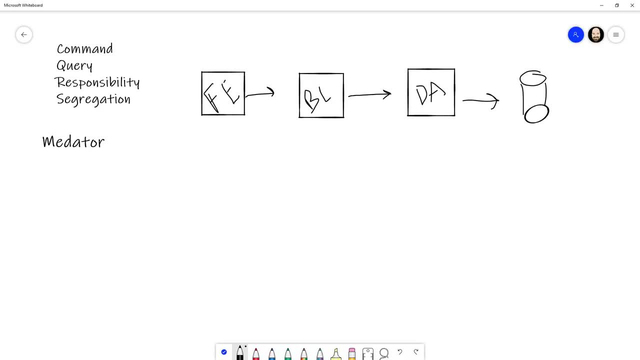 next with mediator is we have this idea that we kind of put some separations in here. you see, right now there's some coupling. now we do have the idea of dependency injection and having interfaces, but in general we've got coupling here where we have our front end talking to our business logic. we 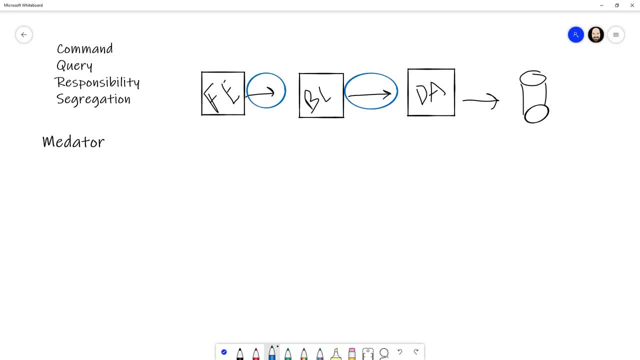 have, we have, we have coupling here. we have our business logic talking to our data access. so there is some coupling now with dependency injection. we reduce that or loosen that coupling by talking to interfaces. that allows us to more easily test things. however, what happens when your application scales well? 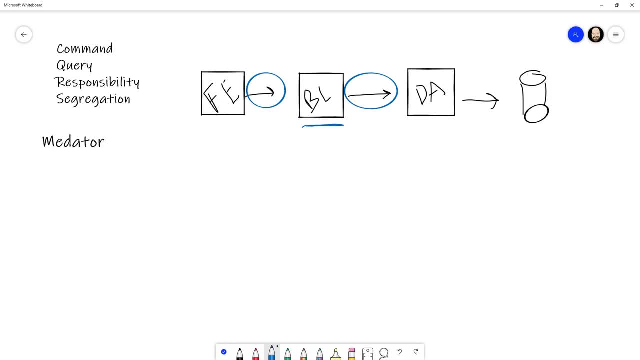 then what happens is, especially this layer right here, we have hundreds of different classes. in each one of those has to talk to a lot of other classes because we're doing things like dry, don't repeat yourself, and conforming to solid, and so on. so you've got lots of these little classes that 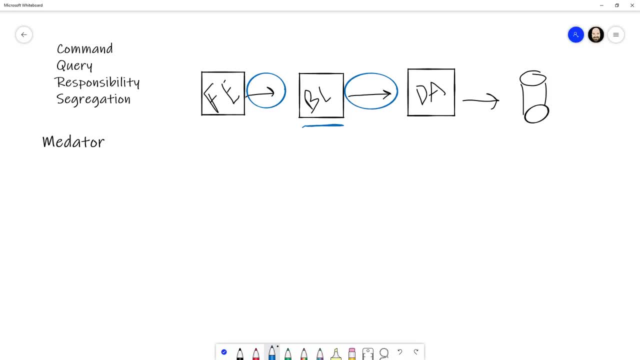 have to all depend on each other, and so what happens is we have the system where, let's just say, we have service a and that's going to need to depend on service b, and that's going to need to depend on service b, and that's going to need to depend on service b. 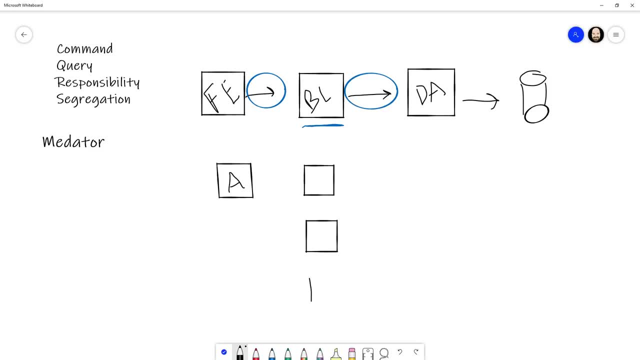 and that's going to need to depend on service a and service c and service d like so. so it depends on those three and in a, a simple world, that's fine. so what happened is, for each of these, you would bring us in via dependency injection. okay, so you would inject those into our a cool. now what happens is we're going to have a little bit of a. 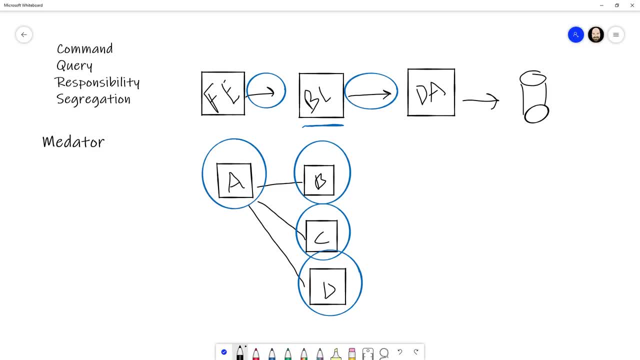 what happens is we're going to have a little bit of a. what happens is we're going to have a little bit of a. what happens if we have a more complex scenario? what happens if we have a more complex scenario? what happens if we have a more complex scenario? say we have 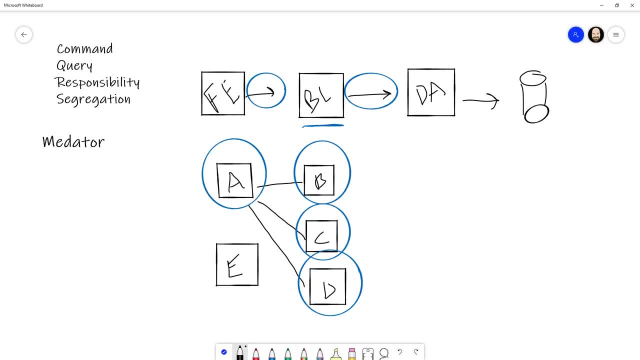 say we have, say we have another service. let's call this service e another service. let's call this service e another service. let's call this service e, or class e that needs, or class e that needs, or class e that needs c and it needs d. cool, that's fine. 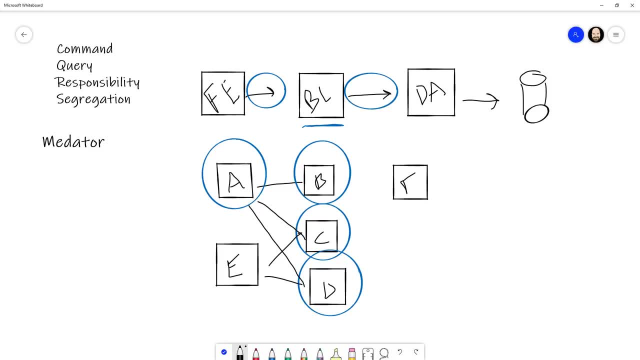 c and it needs d- cool, that's fine. c and it needs d- cool, that's fine. but now we have this f over here, but now we have this f over here, but now we have this f over here, and that depends on b and that depends on b. 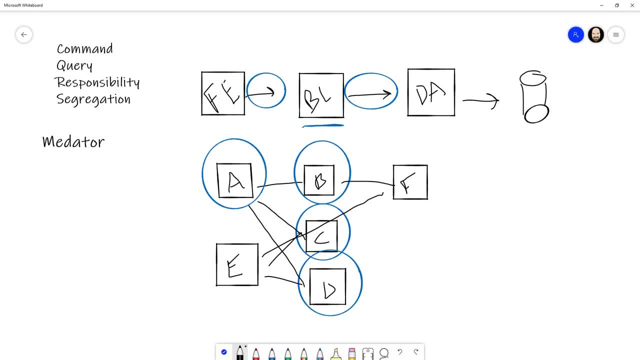 and that depends on b, and now e depends on f as well. so now, and now e depends on f as well. so now really, we've got this, this complexity graph going on, and maybe even we have this dependency from a to e and before we know it, what happens is in our constructor. you've probably seen this before. 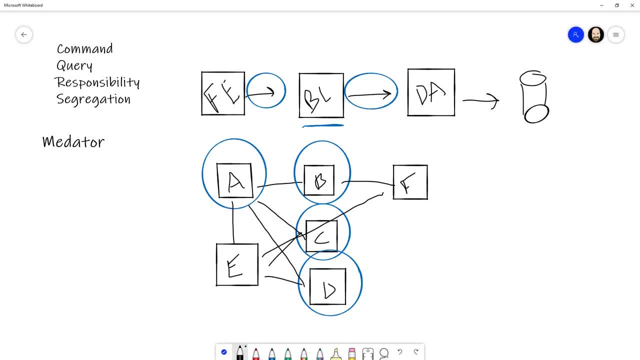 in our constructor where you bring in your dependencies, which is always good to see what your dependencies are right away. you have this list of six, seven, eight different dependencies that you're depending on and that can cause additional complexity. you're bringing all these, you've already got the, the logger you're bringing in. you're bringing i configuration talk to. 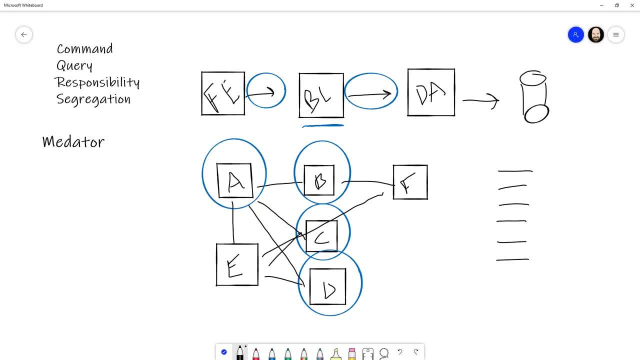 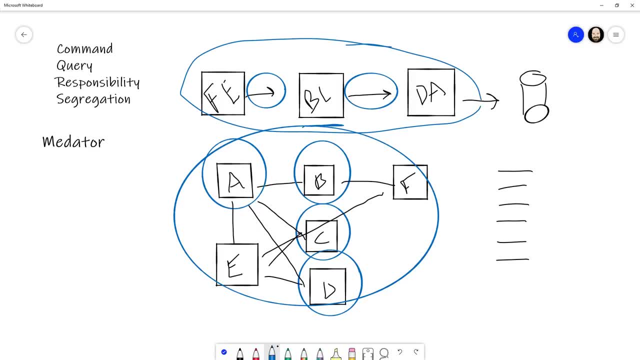 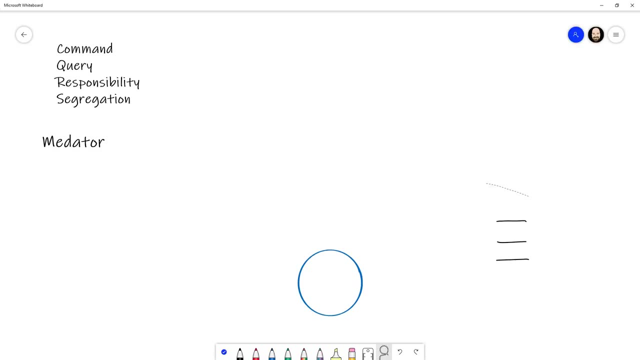 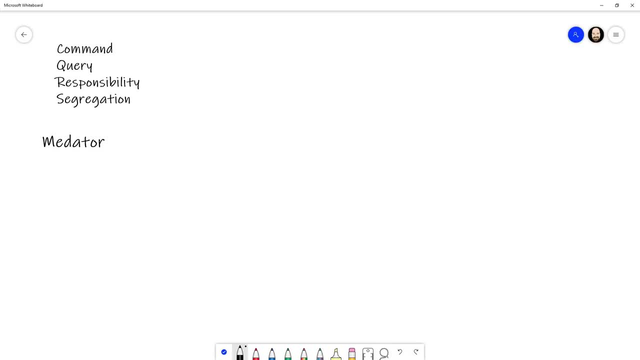 about the mediator pattern. What happens there? Well, let's just say you have a class And that's class A And it needs to talk to class B. Well, instead of going directly from A to B and having that direct dependency, what happens instead is we have this mediator And A says mediator. 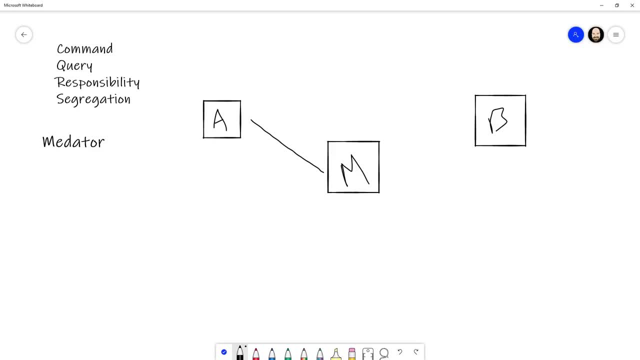 I need something And mediator says okay, I know how to get that, and goes to B. Now this may sound a little bit like dependency injection and in some ways it is, because what's happening is we are allowing something else to tell us what the implementation is of our dependency. but in other ways it's a. 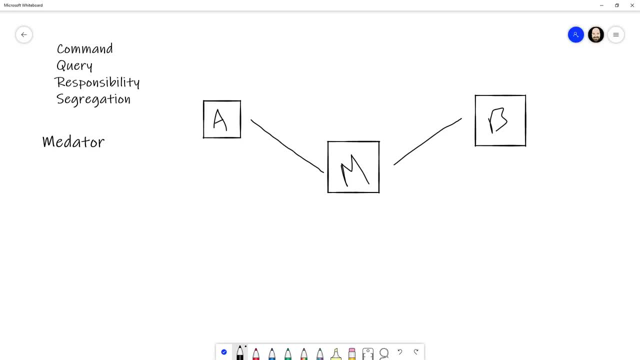 little bit different. Now I'm not going to go too deep into the mediator pattern, but essentially in this we're going to have is one call and one handler. The handler fulfills the call. so the call says this is what I need. the handler says I can do that. 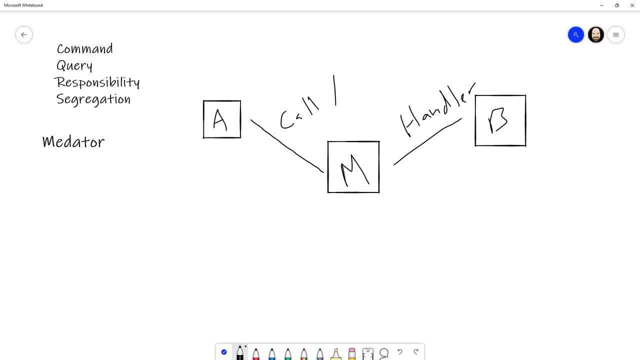 and it's going to do it. and this is a one-to-one relationship. There is not a one-to-many here. we can use a more of a broadcast kind of venting system with Mediator The, the, the tool. but for today we're going to talk about the one-to-one relationship. call to a handler. 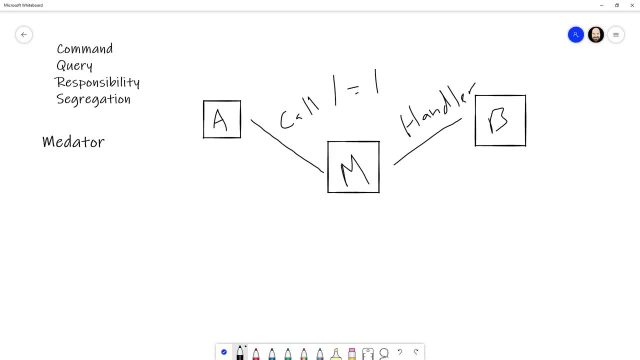 now you may wonder: well, how does that really solve our complexity? haven't we just moved our complexity somewhere else? and the answer is not really we. we have in some ways, but we've moved it out of the the caller, we've moved it out of this location and moved it into here. so if we 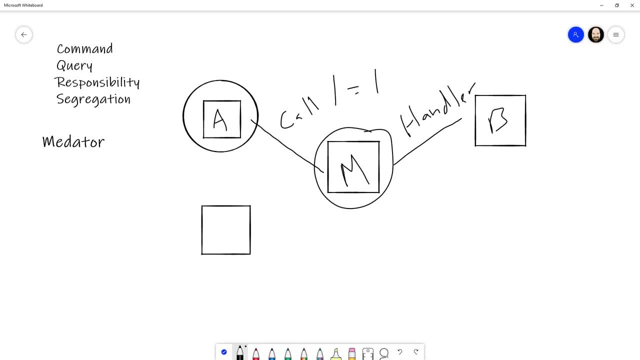 now have. let's just say we have over here c and that depends on b as well. it can call into the mediator and maybe it also depends on uh d. well, c calls in the media again, this time asking for d. this one is for b and it just gets the information, and d might depend on b but it's not going to go. 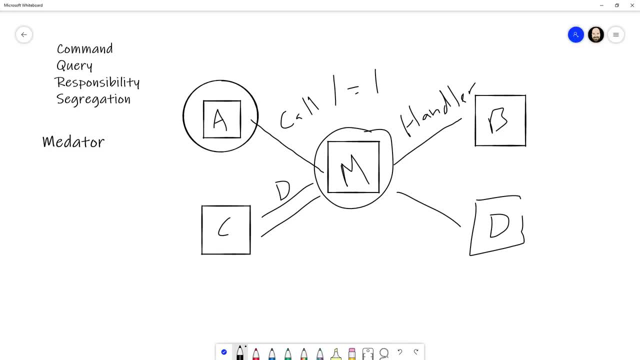 directly. it's not going to do that. instead, what's going going to do is it's going to go and talk to the mediator, which is going to get the, the b handler. so there's this central piece, now called the mediator, which is going to handle all of our. 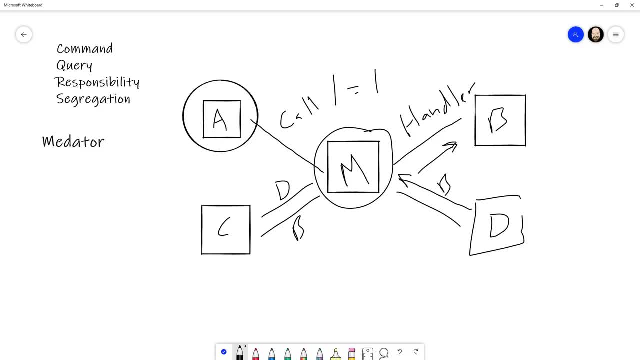 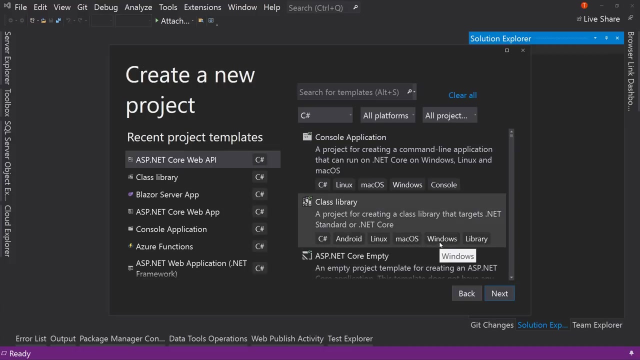 communication between our various systems. now this is all really theoretical. let's talk about, or let's see how to implement this in a real application using the mediator, nuget package. so let's go to visual studio and we'll create a new project. now what i'm going to do is i'm 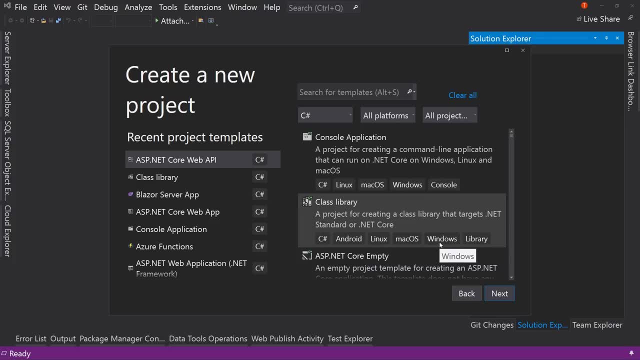 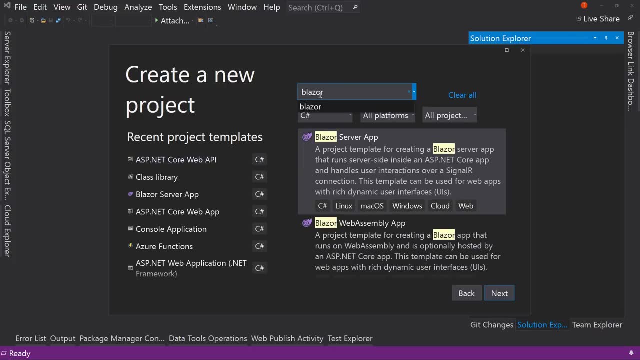 going to create a blazer server application first. so to do that we can search through here to find blazer server or we can type blazer. and they have changed again recently. i'm not a big fan of the new changes but now we find blazer server separate from blazer web. 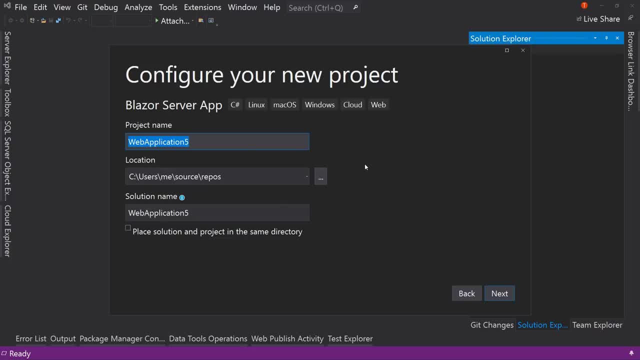 assembly. we can select that, hit next and from there, let's give it a name. let's call this blazer ui and the project name of mediator demo and hit next. we're going to use NET 5, which is the current version as of recording this video. we're going to configure for html. 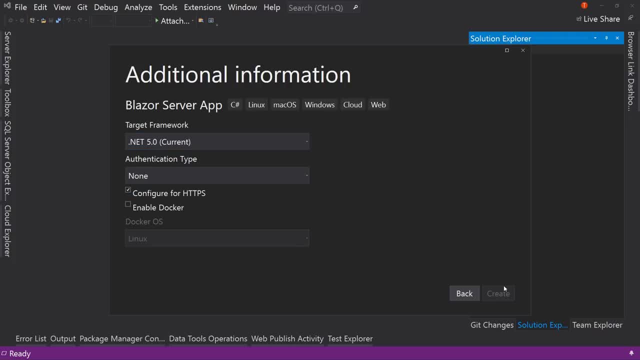 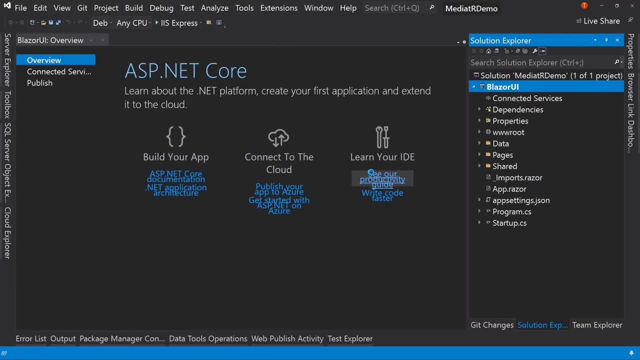 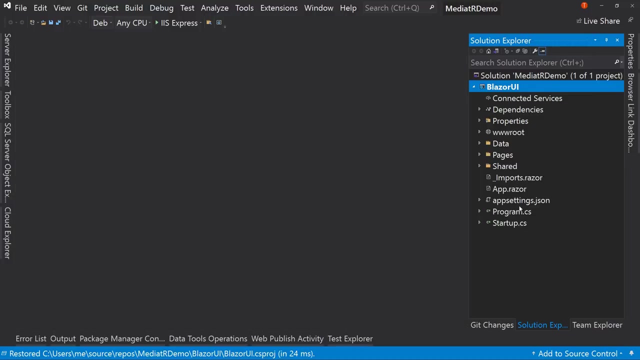 htcps but no authentication. we hit create and this will create for us our sample blazer application. we're not going to go into major modifications of this. we're just going to work with changing this, the index page, and making some tweaks here. that's all we're going to do in blazer. 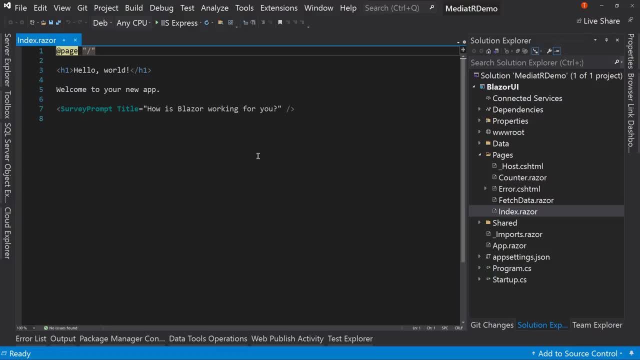 so if you're not familiar with blazer, no worries, we're just using this as a quick, ready to go template that we can then add things to. next up, we're going to add another product to our solution and that's going to be a class library project. 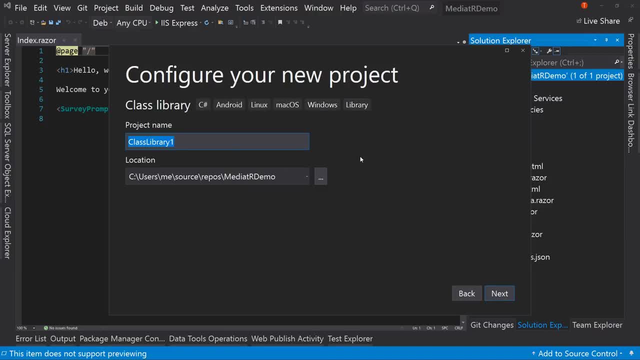 and we'll call this- our call it- demo library. it's fine. yes, NET 5 is what we use. we could use NET standard 2.0 or 2.1, but we're going to use NET 5, which is the current version. 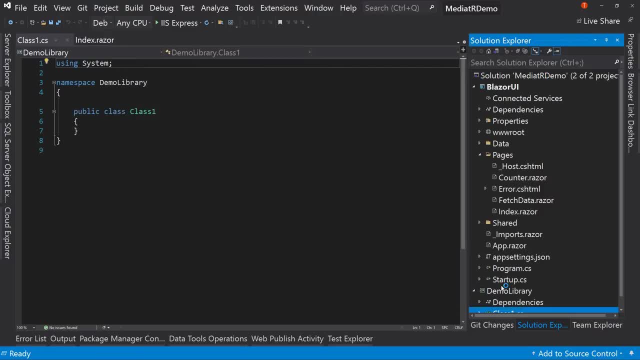 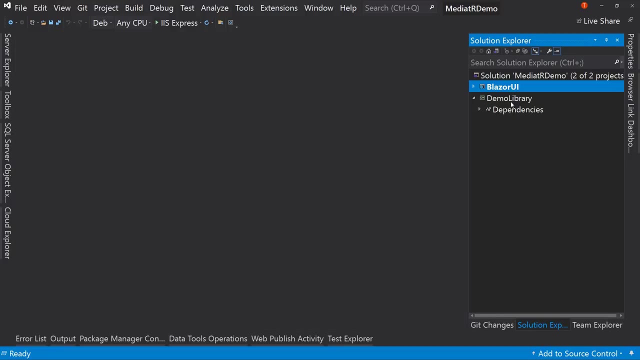 that means it will only work with other NET 5 projects. let's delete class one. and now we're going to do is i'm going to add some sample data access to this demo library. now. i debated putting actual data access in here, because oftentimes people get confused. 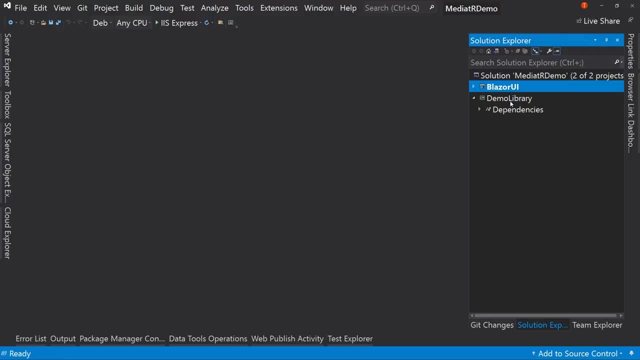 when they see sample data access and wonder: well, how would i do it with sql or with the my sql or with whatever the data access we're going to do here? if you want to replace it with an actual data access that talks to one of those things, you just put the code in the 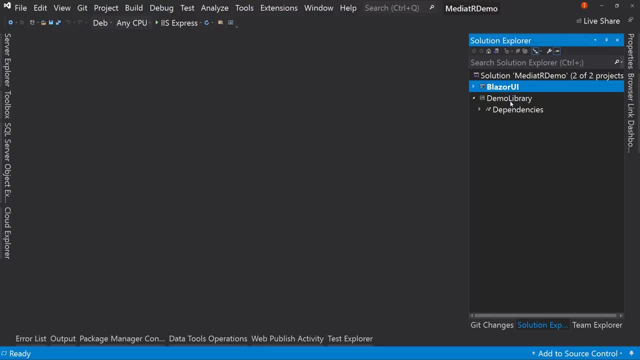 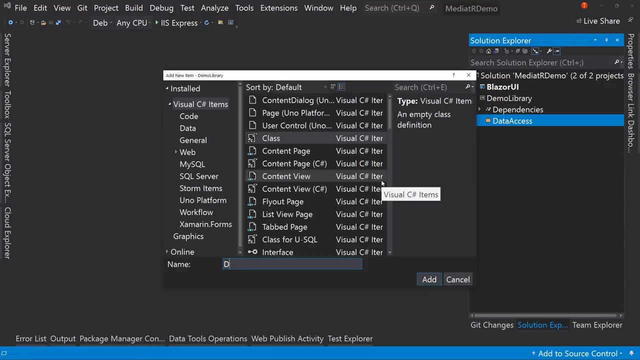 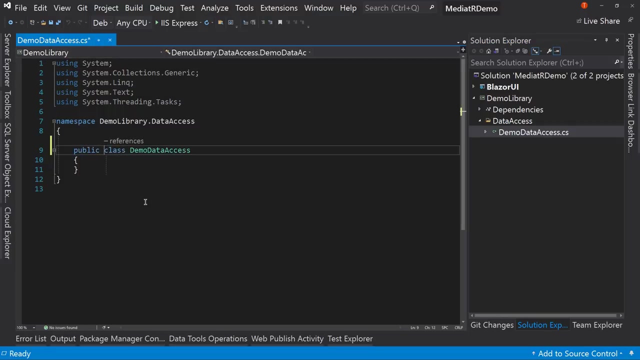 spots in the sample data access. okay, so i'll show you how we're going to do that. we're going to say: add new folder, call it data access, and in here let's add a new class and we're going to call this demo data access, this, Make it public. Now we're also going to need a models folder. I am compressing. 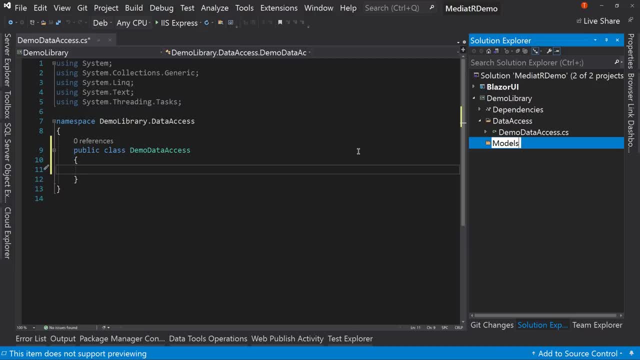 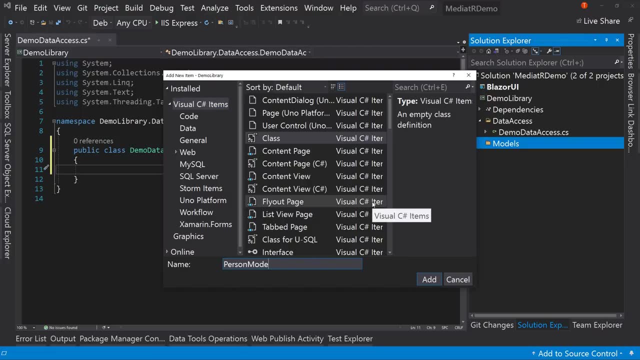 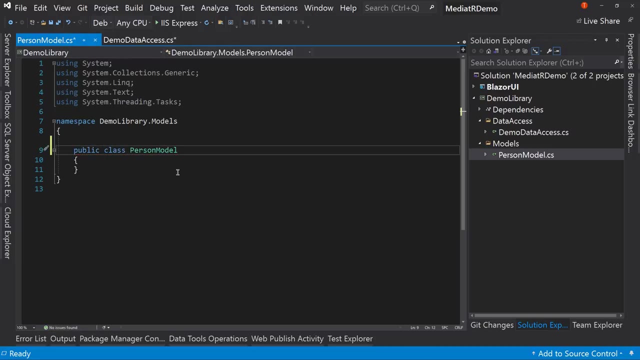 a couple of things in here. Let's call it models And let's create a class in here called person model- Person model, And this is the data that would come from the database. Now I am going to compress a little bit some of the things you could do. You could expand them out. 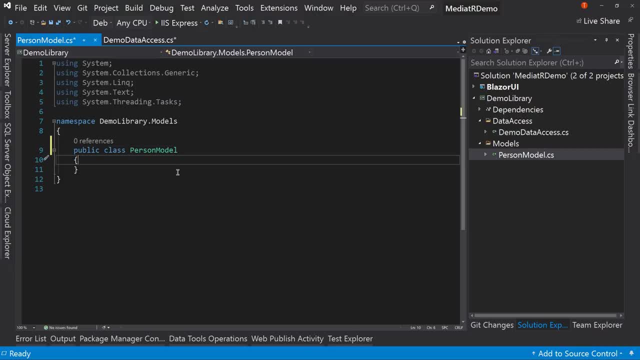 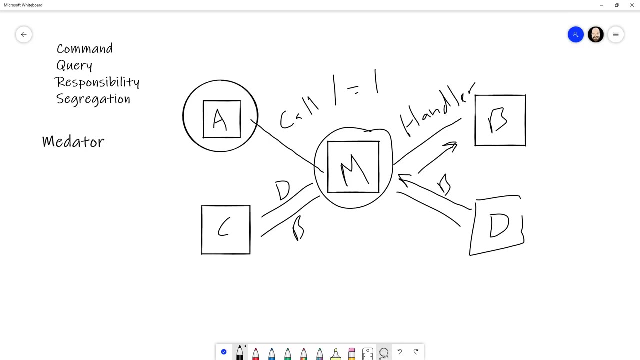 further as your application grows. The balance I'm trying to hit here is that mediator really should be for larger projects. It adds complexity. Let's bring up the whiteboard again real quick And let's start by getting rid of this And let's talk about the balance we have to hit. 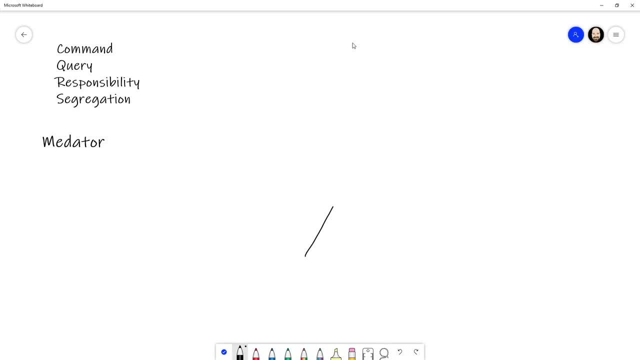 So if you've ever seen, there we go. if you've ever seen a teard, totter or a seesaw or something like that, you have this idea of a beam that's balanced in the middle And then whatever you put on the beam on one side is going to cause the beam to go down that side, which lifts the beam. 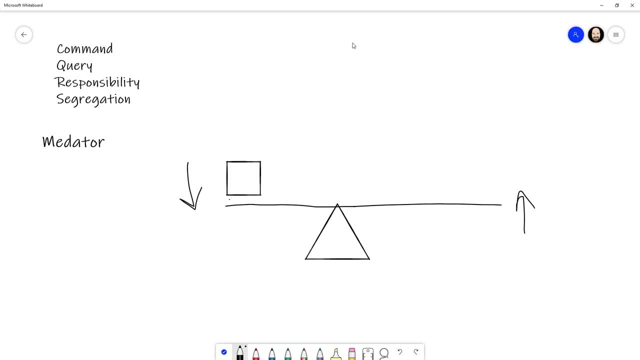 on the other side That's a fairly standard playground thing that kids do So. on one side we have the- the size or the complexity Okay. So how big or how complex is our application? If we have a hello world application, it's very tiny, which means there's just a little bit of 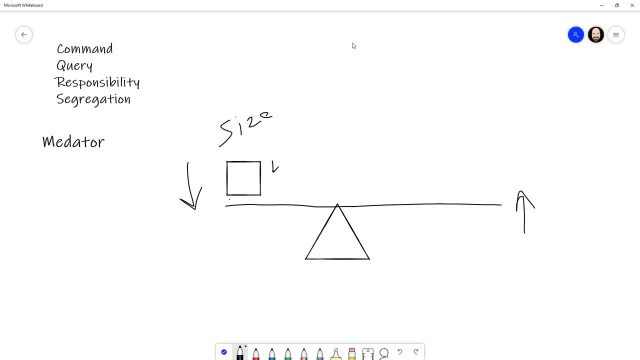 force pushing down on this side of the balance beam And because of that we have to have on the other side to balance it out. We have to have a little bit of- uh, best practice patterns, those kinds of things. Okay, so this would be the patterns. 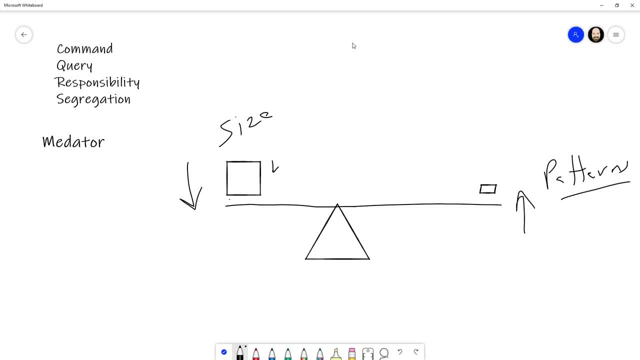 So the the smaller the size of your application- roughly the smaller size- and the less complex your application is, the smaller you want your uh, your patterns and things you applied your application, things like dependency, injection and even dry, Okay Okay. 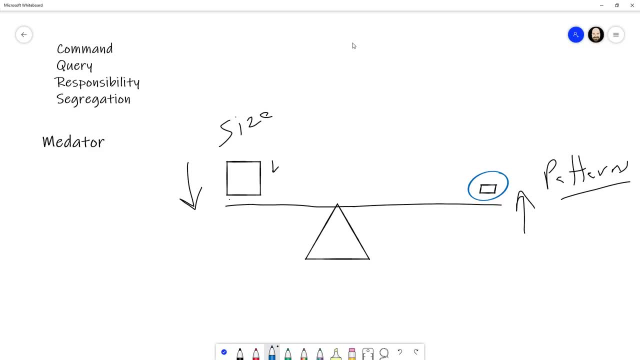 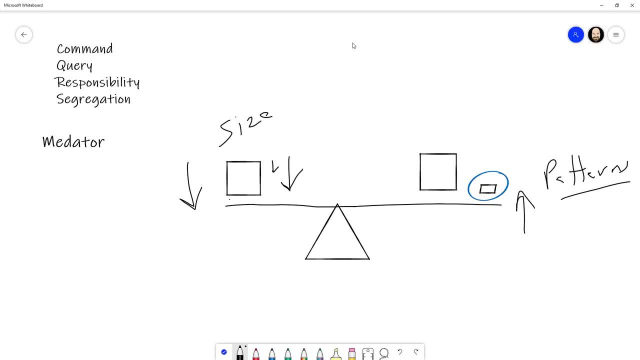 design principles, going into balancing out your application, because the ideal here is that we have this line right here: be equal. okay, so that they've got the same. you know we don't have a the, the balance beam. look like this where we have it. you know, unbalanced. we don't want an unbalanced. 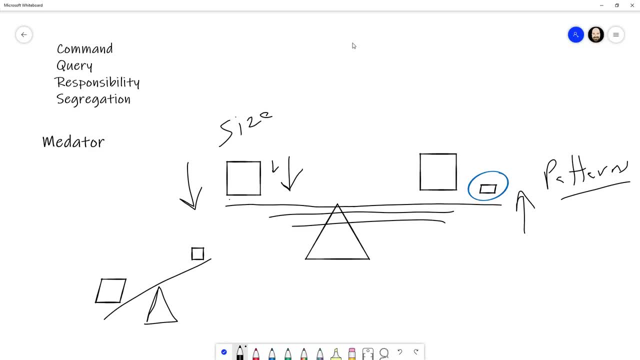 application. instead we want is this concept of the larger and more complex our application gets, the more we apply patterns and systems to make our application easy to maintain and easy to manage. but that ease is relative to the size. okay, if you apply, let's just say: take, for instance, if you have a small command line operation that said: 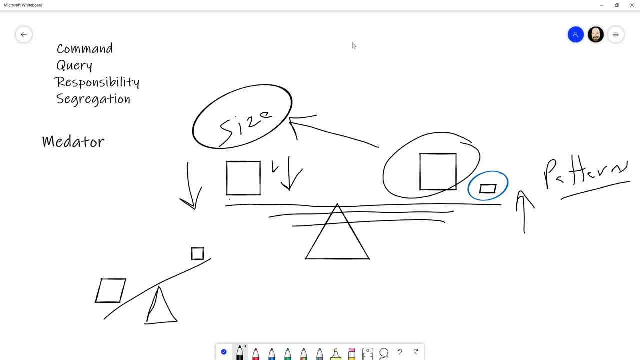 hello world if you follow conventional wisdom where you say, okay, dependency injection is good and solid is good, and making sure that we are, you know, dry and having interfaces, not implementations, and all this and unit testing, applying all that to a hello world console application, will give you 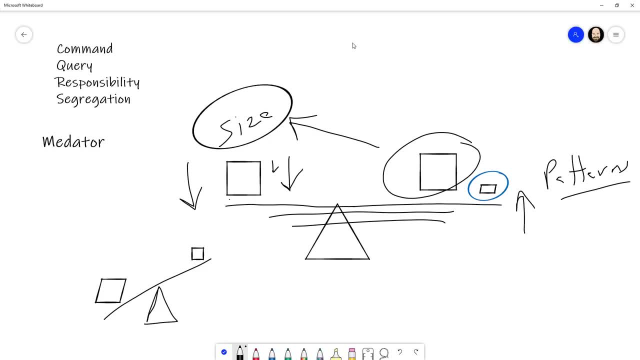 about 200 lines of c-sharp code for one line of actual work. that's ridiculous. that is unbalanced. so what you want to do is maintain the balance based upon the size and complexity of your application. all right, so that's what we're we're looking at doing here. that's why i say mediator and cqrs. 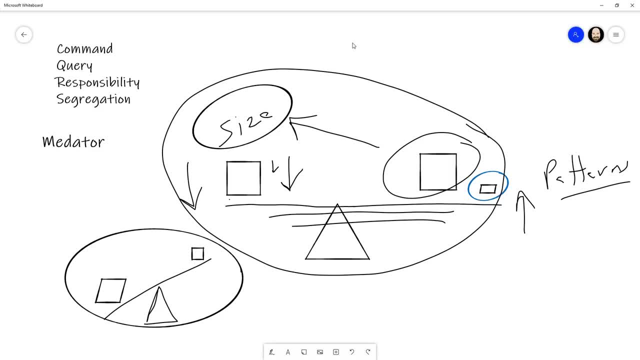 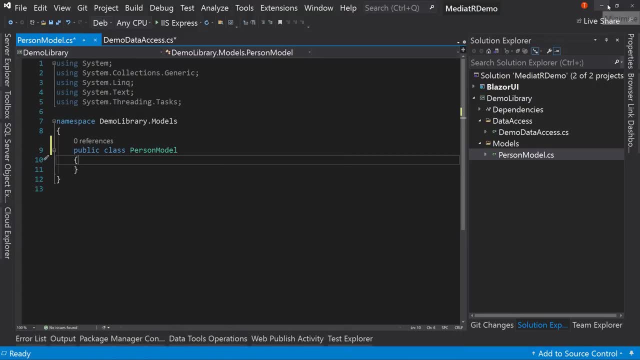 is not for every application. it's going to be for larger applications. so what does that mean for this application? well, i'm trying to build a small application in order to show you just the mediator tool, but that means it's really too small to work for higher implementations. very important: having mediator and cqrs implemented in it. 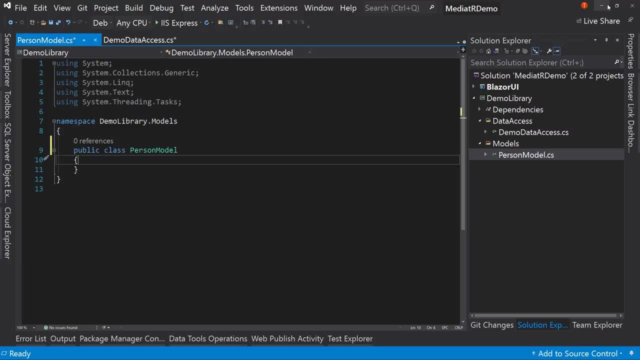 so there's gonna be a little bit of a go with me here. there's a little bit of a saying. this is what it's going to look like in its barest form, but in a larger application you will see how it would be beneficial. okay, so just note, we're gonna. 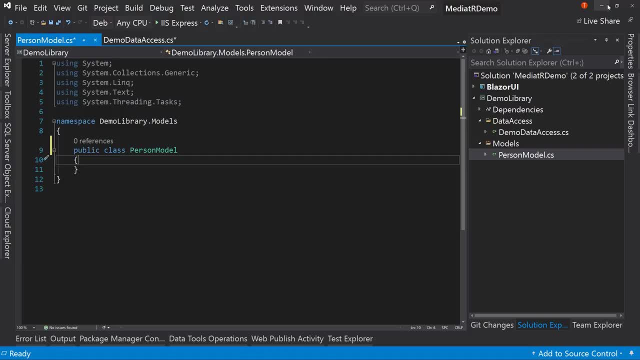 do just a little bit of of work here, just a little bit, to show you what the cqrs pattern looks like and what it goes anywhere. instead of this buildup, but instead of the cqrs standard, employment teams will feel like an equally reallyaaa great, Windowsな- humanistic workflow compared to any яанта. 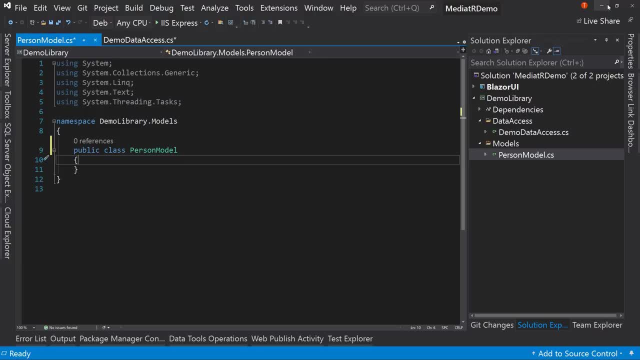 as how Mediator can make our lives easier, but it will grow over time in a real application. So back to our person model. we're going to put three properties in here: ID, first name, last name. Okay, Those are the three properties we're going to put into this person model Again. 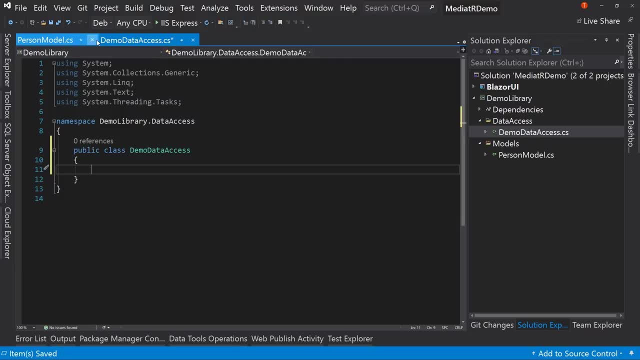 in our demo data access. we're not actually going to go to a database to get this. Instead, what we're going to do is we're going to actually have right in here private list of person model, which that adds a using statement, by the way, for person model. person model- people. 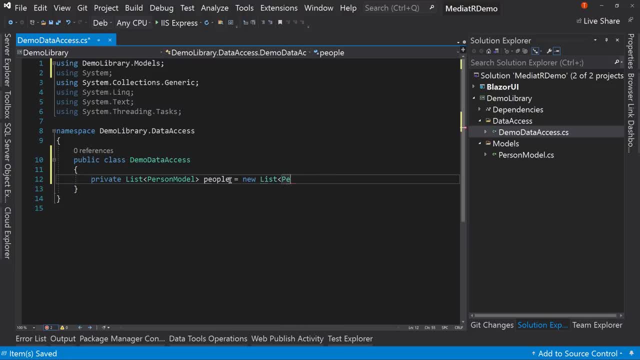 equals new list of person model. Actually, I can just say new. That's the new C sharp nine syntax, which allows us to not repeat saying this just to instantiate something. Now in our constructor I'm going to say: people dot add new person model. 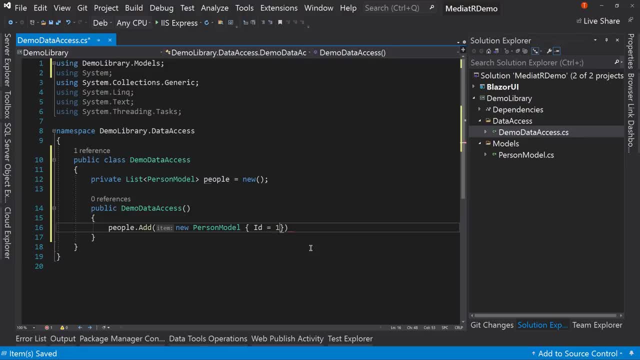 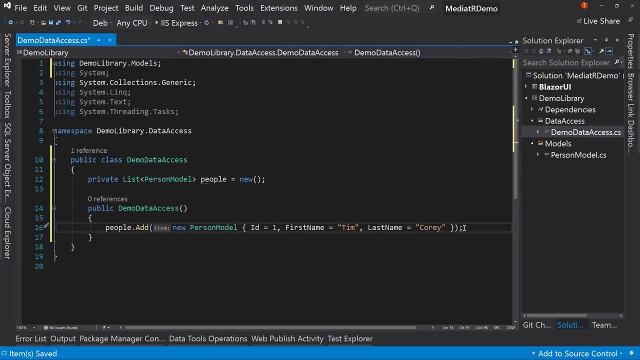 And we'll say: ID equals one, first name equals Tim, last name equals Corey, and put a cynical at the end. Let's try it out so you can see it. And we'll do this one more time And we'll have my ever present helper to store. Okay, And now we 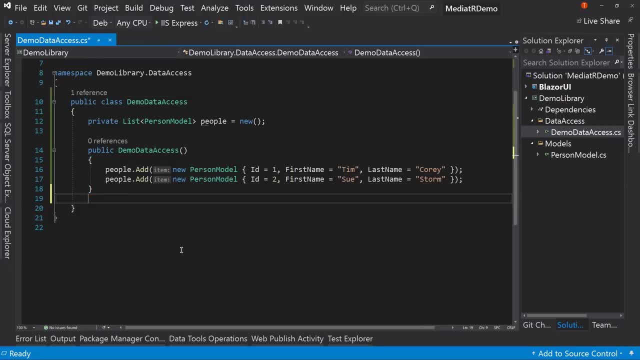 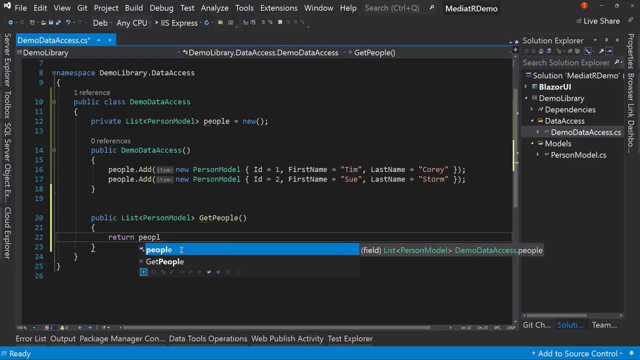 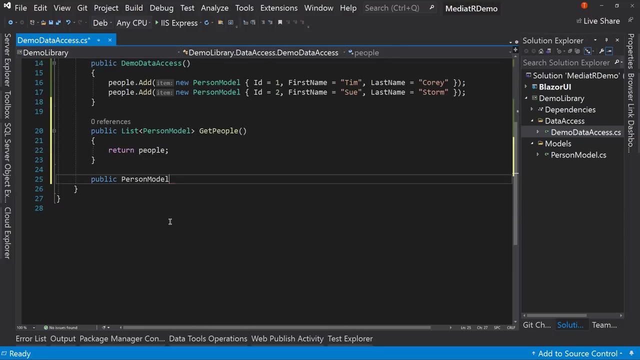 have our data access set up. We're going to have two methods in here: public list of person model, and that's going to be get people, That's going to return people, And then we'll have a insert method here: public person model. 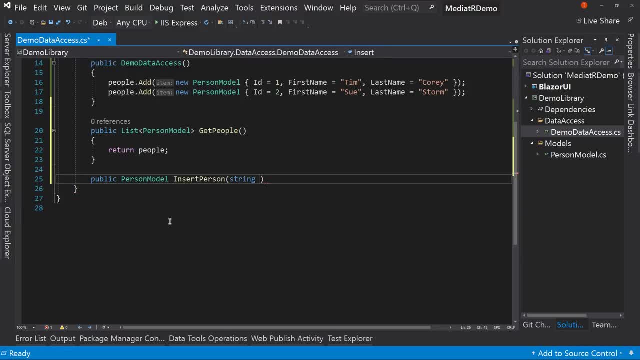 insert person string first name, string last name, And in here we'll say: person model P equals new autocomplete- It's going to do that for me about that- and then say first name equals first name, Last name equals last name. 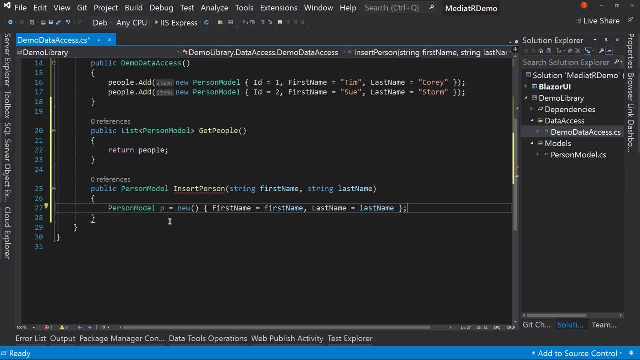 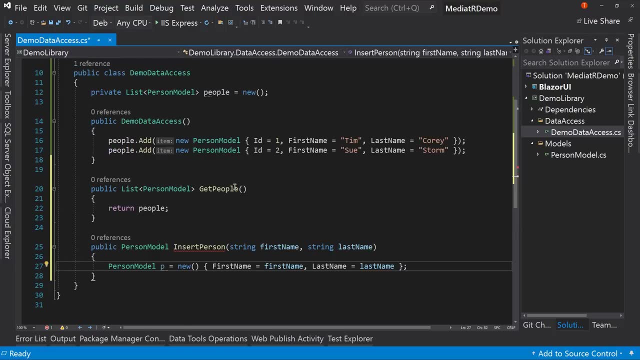 I'll explain this in just a minute. So what we're doing here is: remember I said that if you want real data access, you just need to replace the methods here. So this get people. we're just returning our list from up here. 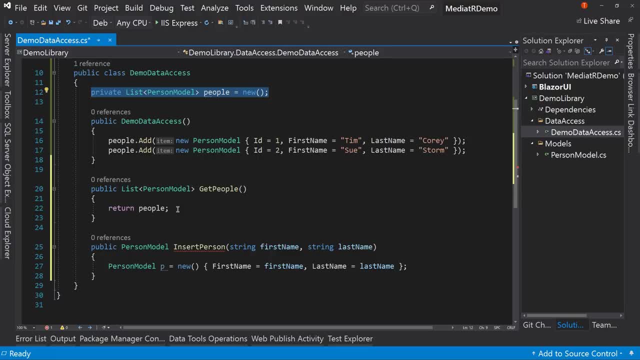 but instead we could do is you could say: well, actually go out to the database right here, Get that list of people, that list of people, convert it back and send it back as a list of person model. That's just a Dapper call. If you're using Dapper in SQL, that's just a Dapper call. You've seen that in others of. 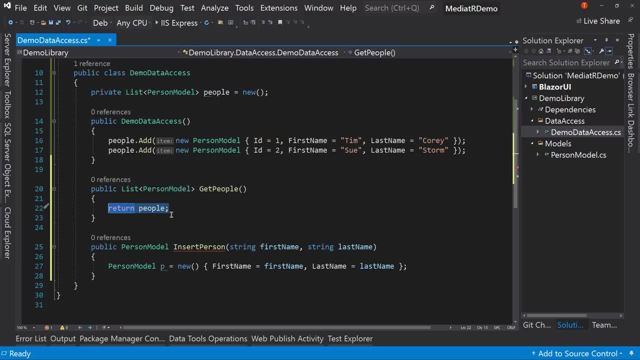 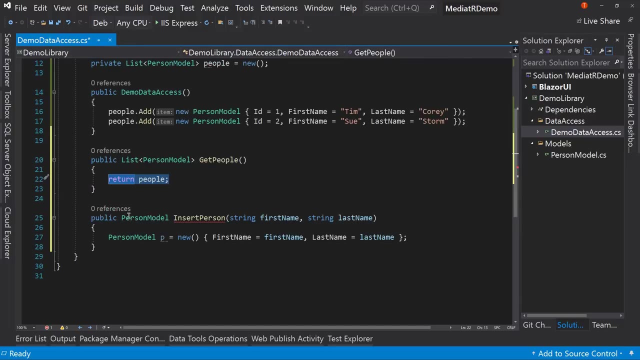 my videos. Look at the Timco Retail Manager, for example, to see an example of that, where you just replace this with a call out to Dapper to say, hey, load this store procedure or load this table and return the values. Same thing here: The insert. we'd actually insert this in the database. 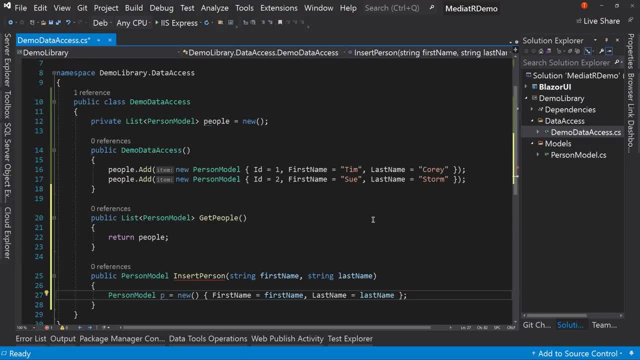 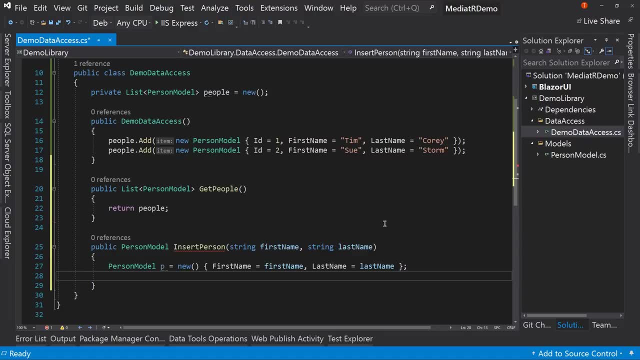 but instead what we're going to do is we're going to add it to this people list. Now, the only kind of tricky bit here is I need an ID, that I want to actually have a real unique ID. So pid is going to equal peoplemax and we'll say x, arrow, xid, That's going to get the max. 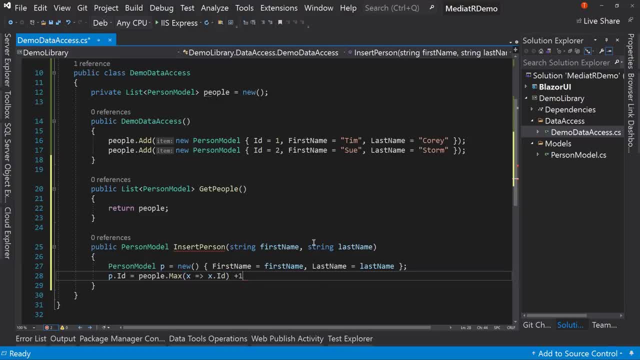 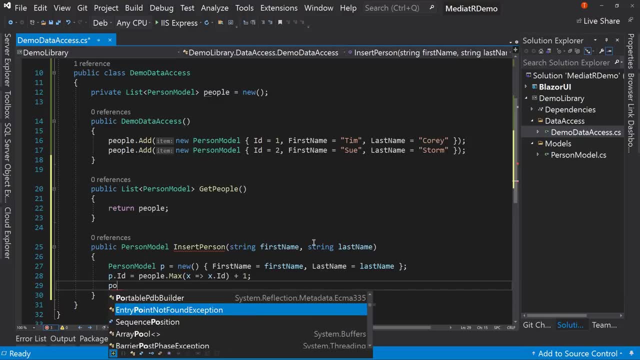 ID already in our list and we're going to add one to it. Really simple stuff here. And then we're going to say peopleadd p. That's going to add our new person to the list. That's our insert. But we have this return and the reason you have the return is because we want to see. 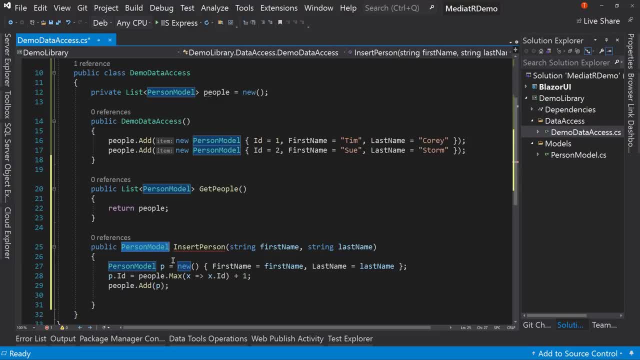 what the data is we inserted, including what the new ID is. So we'll just return p. That's it. So that's our insert method and that's our complete demo data access class. All we're doing is two things: getting people and inserting person. That's it What we'll do. 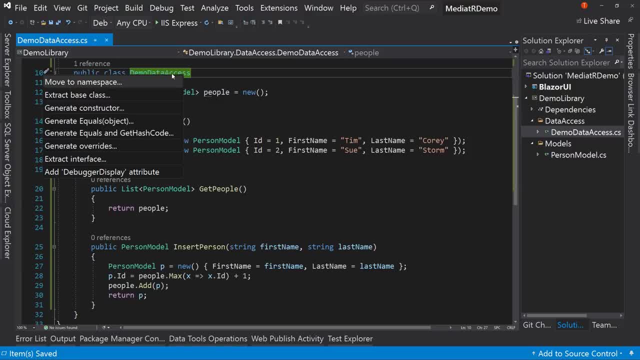 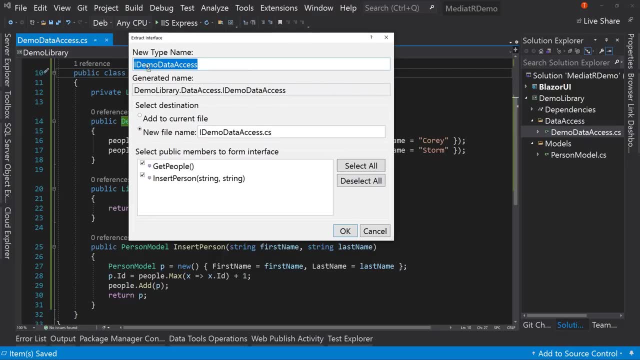 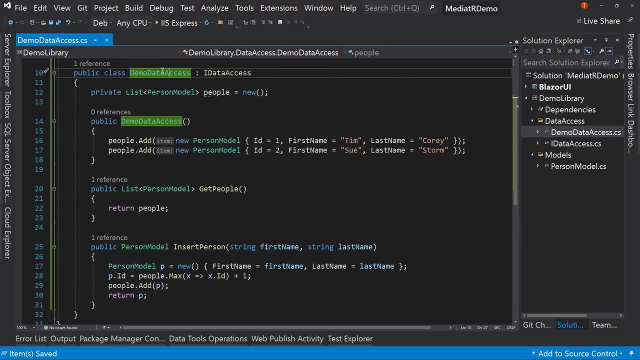 is we'll create an interface. So control, dot on my class name and say extract interface, And the only thing I'll do here is I'll change this from IDemoDataAccess to IDataAccess So that way, if you want, you can change and create a new IDataAccess that does the real job. 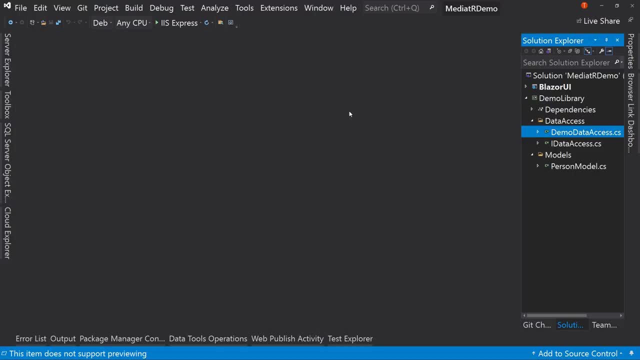 So we're all set with our setup stuff before we get to Mediator. So let's go back to our Blazor UI and let's talk about what we're going to do In the index page we're going to put right in here. 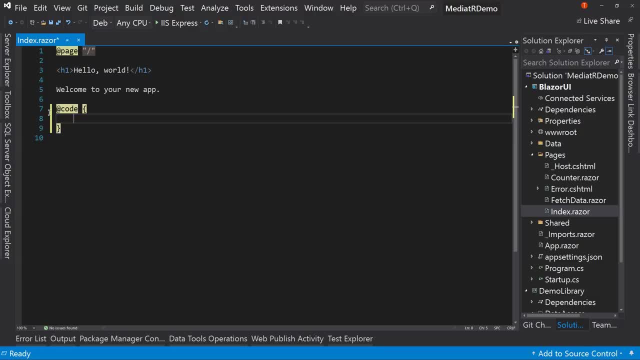 let's actually create a code, section Code, and in here we'll say protected override, And that's going to be the onInitializedAsync, which, of course, is going to mess up my formatting. No big deal, We'll just fix the formatting And in here we're going to do some type of work. 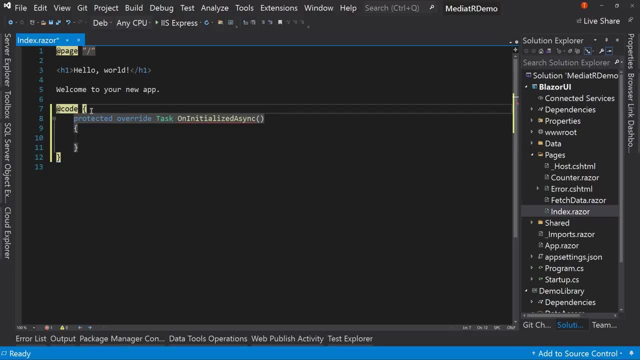 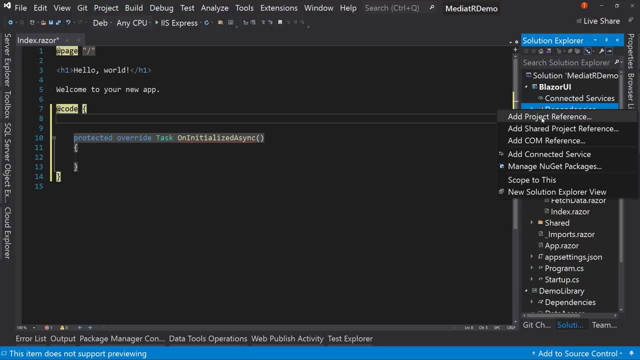 We're going to say: I want to get information. In fact, what information you want? let's define it already. So let's create a dependency, a project reference dependency to our demo library, And now we can say: I want to have access to, and we'll go to this Models folder here and say PersonModel. 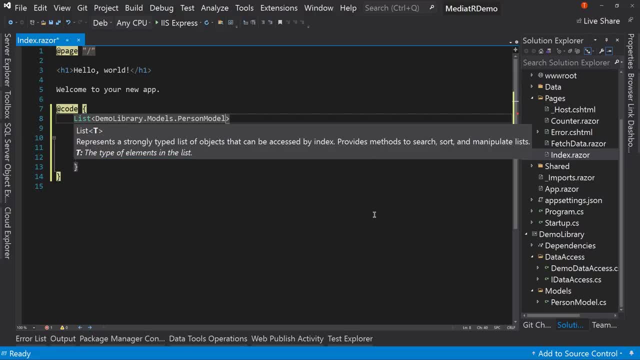 I want a list of PersonModel, which of course spells the whole thing out, List of PersonModel called People, And we will initialize that in this onInitializedAsync. but we don't know how to get this yet, So first let's cut this out. 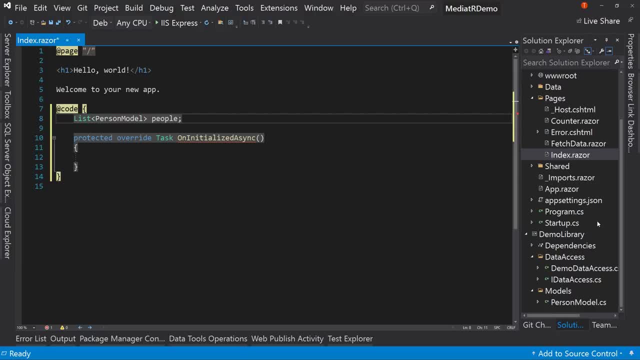 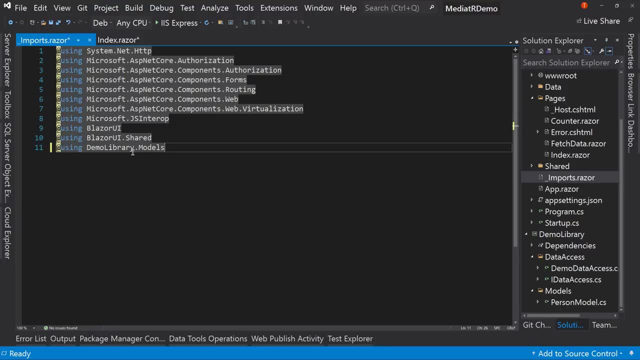 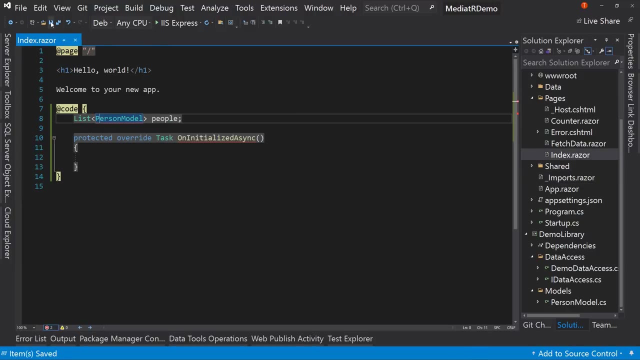 And we'll put it in the importsrazor. We'll paste that in. Now, if I'm losing a little bit with this Blazor stuff, I do have videos introing Blazor itself. The keys here are: I just add a using statement there. 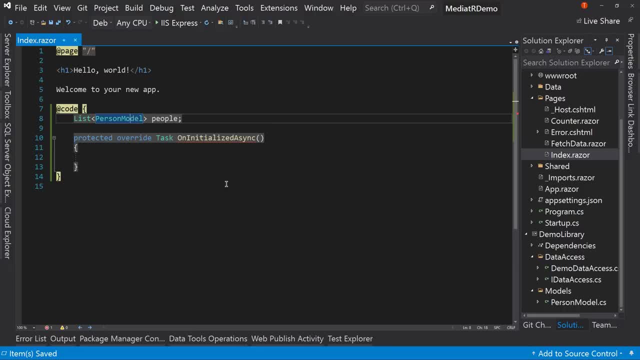 And this is going to get called essentially at the beginning of when the page loads. There's some more nuance there- You can watch my Blazor videos For more on that- But essentially that's what it's going to do, So we're going to load somehow. 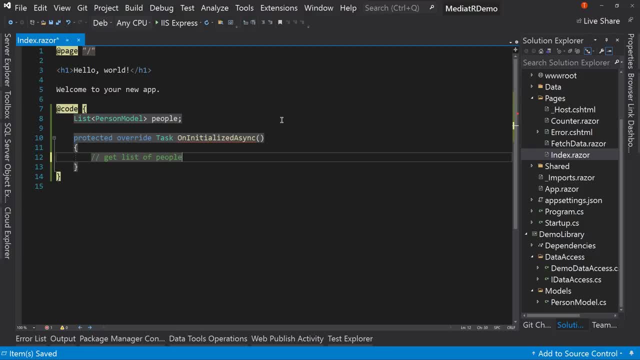 Get list of people. Okay there. Now let's just get that to go away. That writes quickly. So now in here we're going to create an unordered list. Now, if you're not familiar with HTML, that's essentially a bullet point list and we'll say at for each and we'll say var p in people and we'll have a list item where we'll say at p dot first name, space, at p dot- last name, and we'll have a list of all of our people. we've loaded. 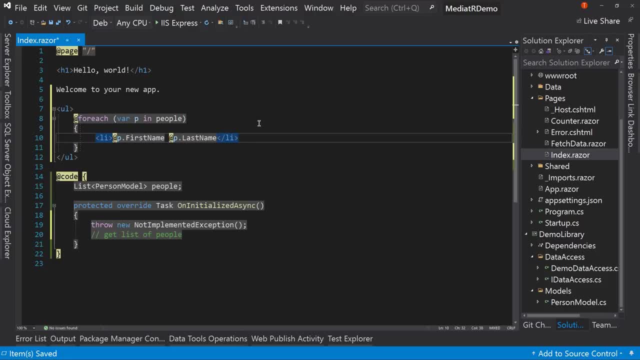 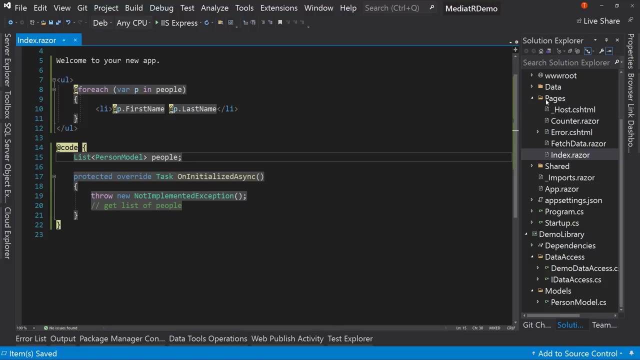 This is going to show us right now Tim Corey and Sue Storm. Okay, that's a theory, but we haven't yet loaded This list of people. So how do we load this list of people? Well, let's start by setting up our demo library to use mediator. 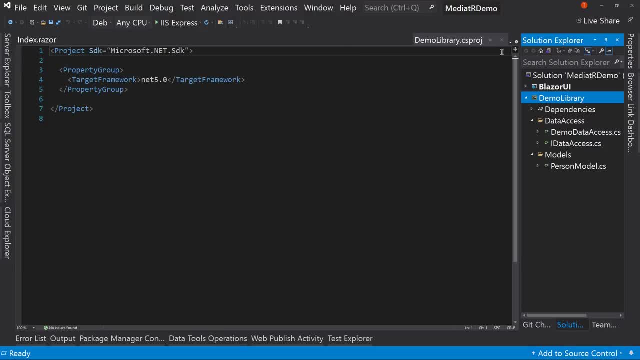 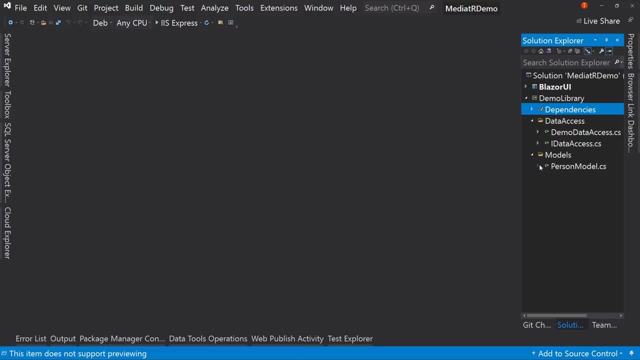 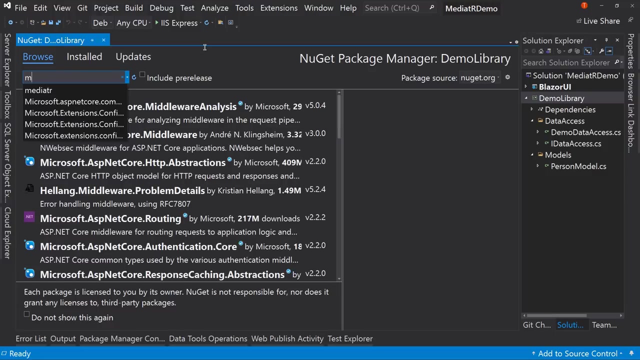 So in our demo library we're going to: let's close these out. We're going to right click on our dependencies and say: managed NuGet package. It will search for mediator. I spell it right, Okay, notice: there's no O in it. 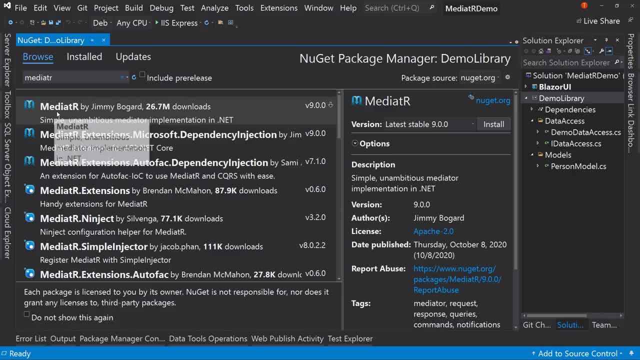 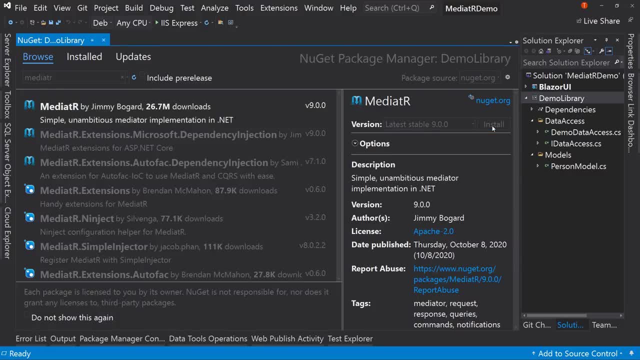 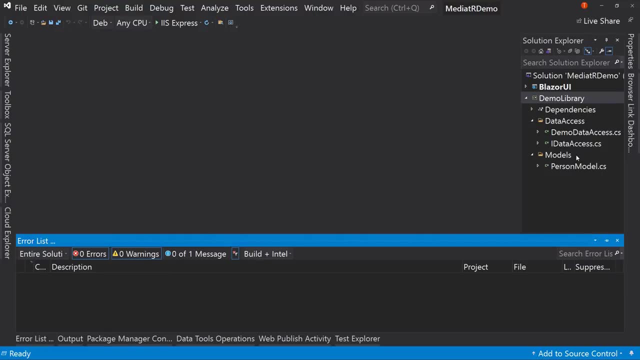 That's not misspelling. That's how it was designed: mediator. So we just want the bear mediator, which currently is at 9.0.. We install that And now you set up our NuGet package. Now let's actually build out a mediator setup. Now remember that I said that the CQRF is not going to be able to build a mediator. Now remember that I said that the CQRF is not going to be able to build a mediator. Now remember that I said that the CQRF is not going to be able to build a mediator. 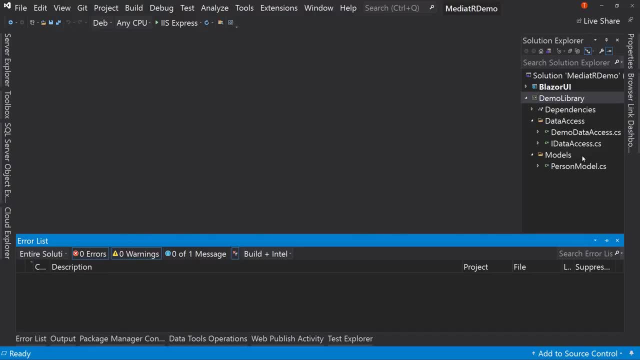 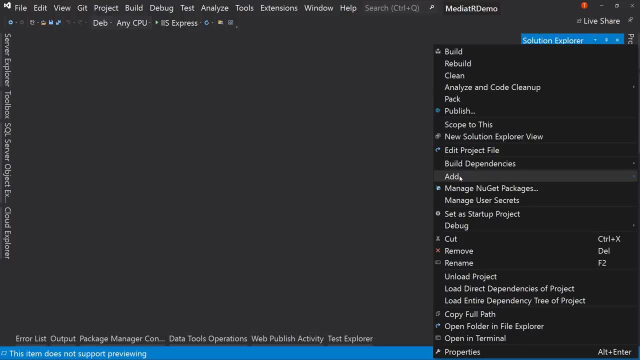 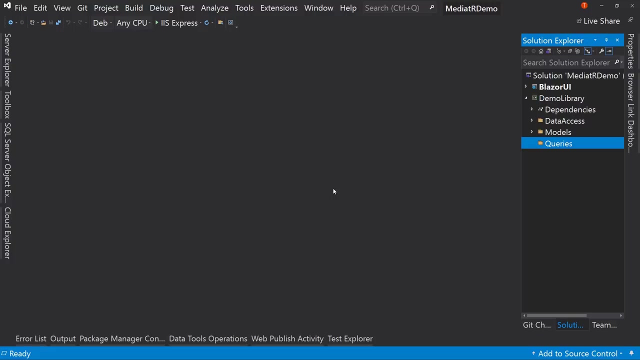 The CQRS pattern is supported by, encouraged by mediator And in fact it's fully compliant with it. So let's create folders for those items. We have first our queries. These are the things we're reading. These are our read commands. 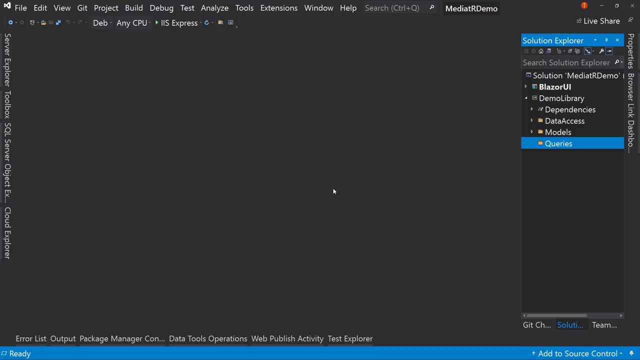 Remember that CQRS splits up, reads and writes. So the other side of it is a folder we'll create called commands, That is, the, The, the rights, the things that we're going to insert into the database. And then we have, finally, we have- our handlers. 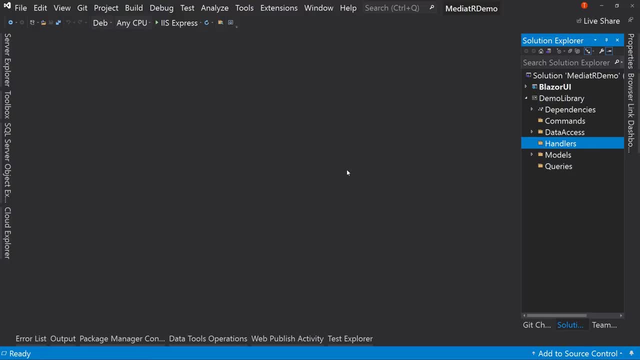 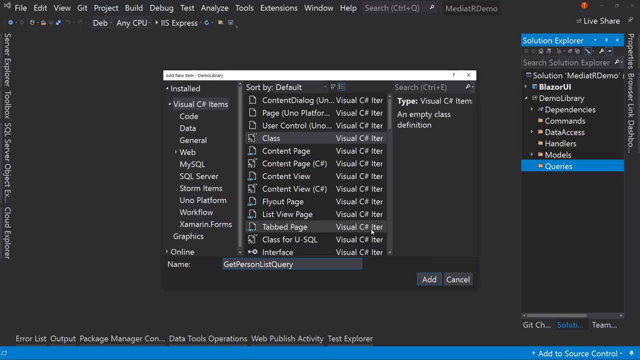 So what's gonna happen is we're gonna say I have a query, I want run And in fact let's create one. So we're gonna say: add new class and we'll call this our get person list query. Okay, I'm calling it query at the end. 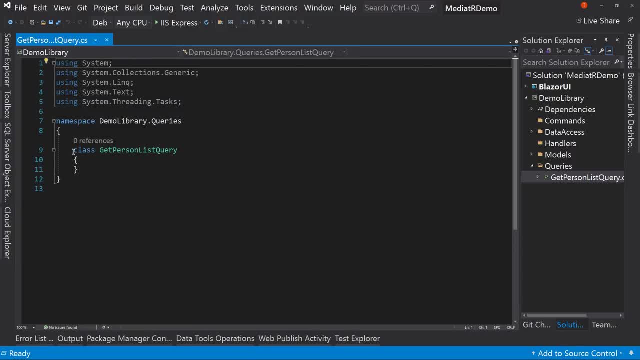 It's a naming convention, just to let me know that, yes, this is what it's for is a query or a command That's more specific to the CQRS. Now I'm gonna change this. Instead of being a class, I'm actually gonna take it off. 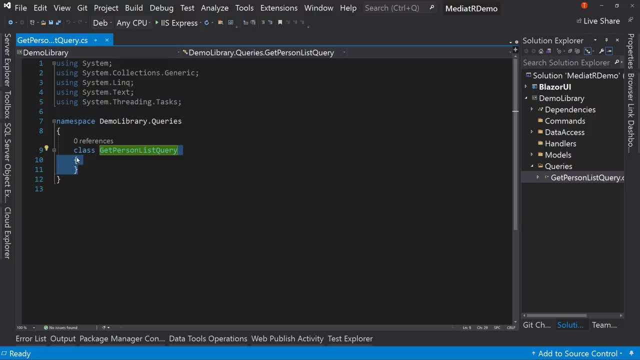 and change it to a record. Now, if you're not familiar with records, I did cover that in a previous video. I have a video all about records and what they're used for. So records are just like classes. In fact, they are classes. 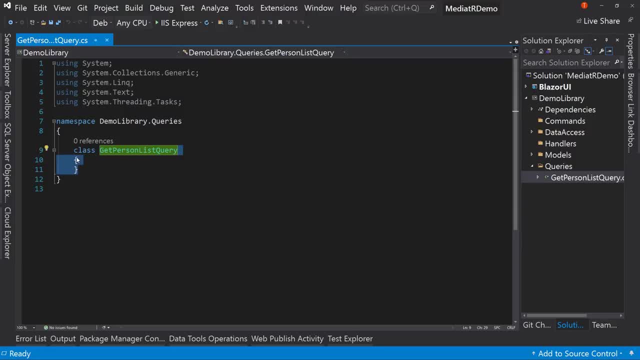 except that they've got some additional syntax goodness, And part of that is you create them once And then in theory they are unchangeable, meaning they're almost read-only. Now, I say almost, because there are things you can do to force the read-write, but you shouldn't. 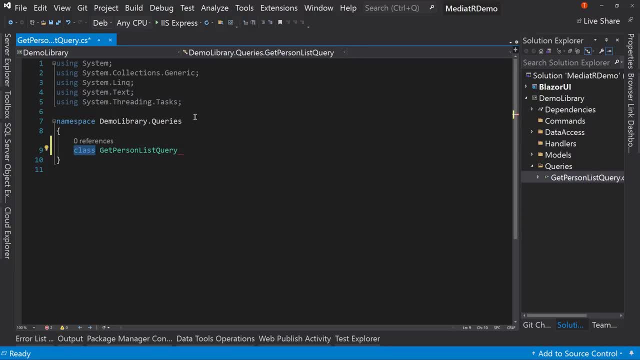 So let's get rid of this and we'll say public record. Now a record gets declared in a couple of different ways. We could specify every property with an init for our set, but instead we can just use our open- close parens and say: these are the values inside here. 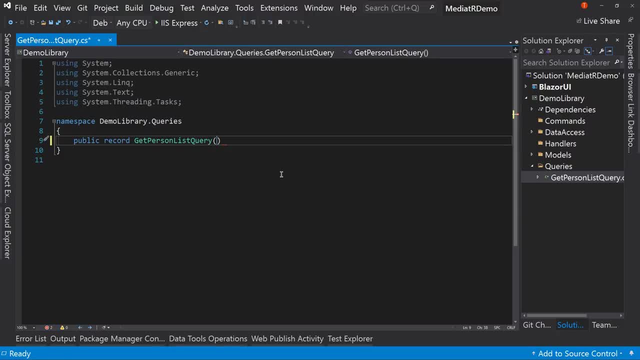 that are gonna be my properties. But in our case, since we're asking for all the people, there is no data we have to pass in. So I just gotta give an empty record meaning it has no properties. It just has essentially a name. 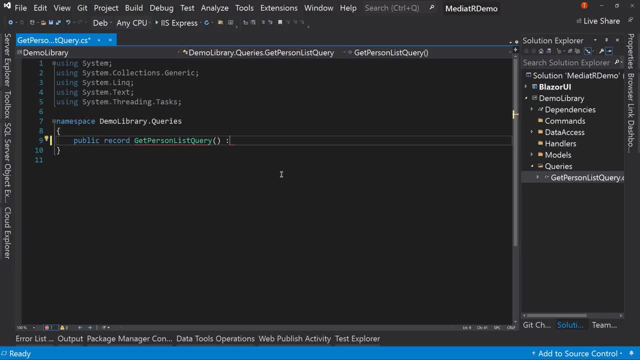 And then I'm gonna say this inherits from- I'm sorry, implements. I request Control dot there to add using mediator, And then this is gonna be what it returns. This is our out or our response. So I'm gonna say, well, 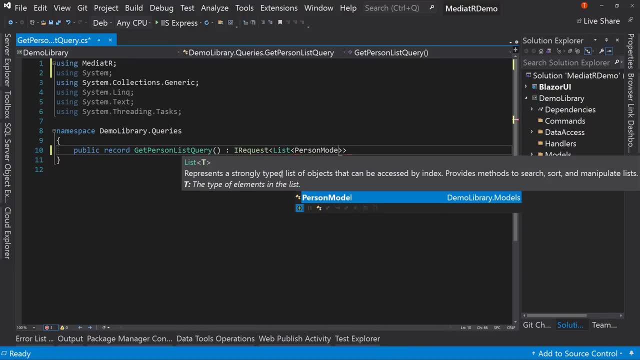 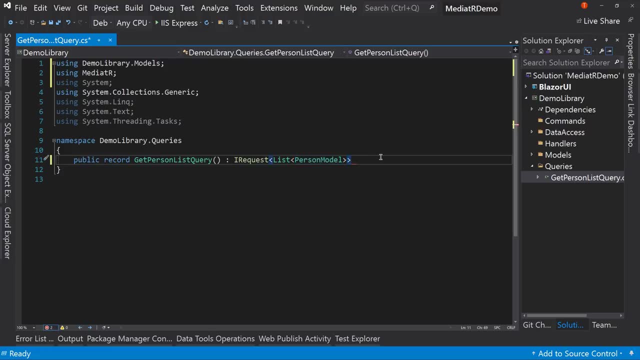 it's gonna return a list of person model Control dot again to add that using statement as well, And the very end we need a semi-colon. So this is our record and this is what it implements, this interface which just says: here's what I'll return. 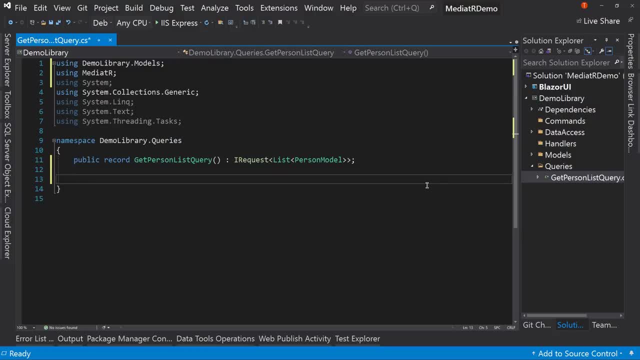 Now, if you wanna do a class instead of a record, not a problem, let's type it out here: public class. Let's call this: get person list- query class, Just so you can see it. Oops, Oops, There we go. 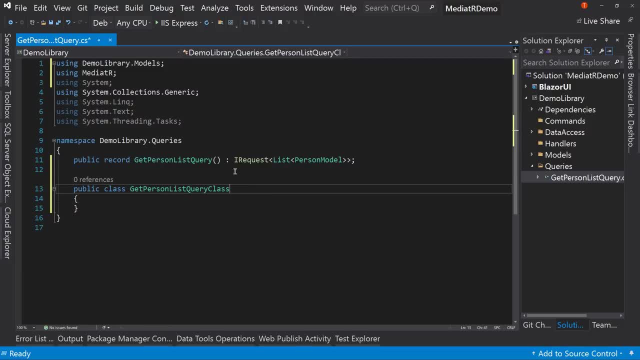 And then in here we'd have no methods, But I would still do the same interface like: so. So this and this are equivalent, except the fact that a record has the additional syntax and goodness that records provide, such as being immutable by default, and so on. 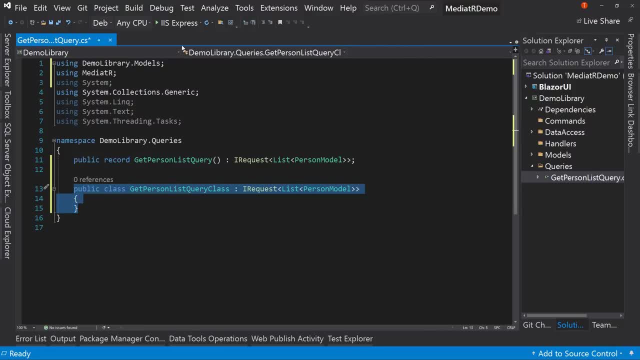 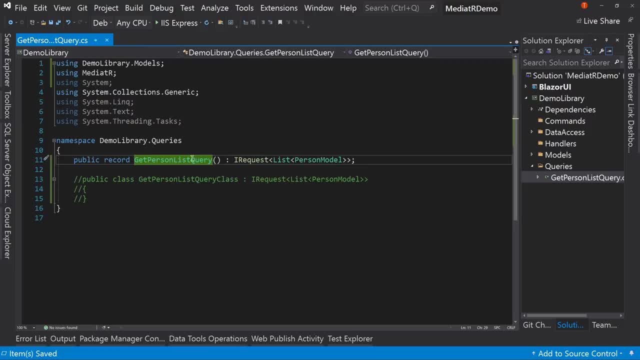 what's going on. all right, so that's our get person list query. this is the data we're passing in. it's also how we'll identify what the the handler is and that's where we start talking about the handler. so it will wire this up in a minute so you can see it called through, but every 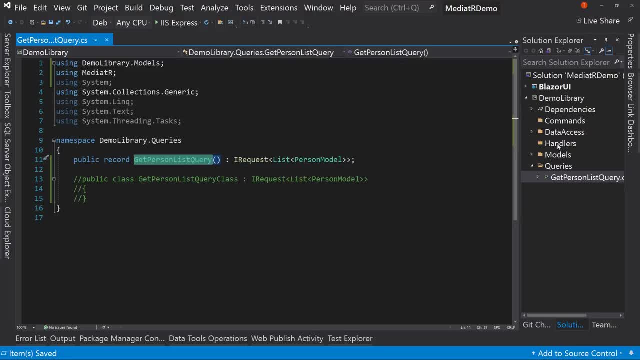 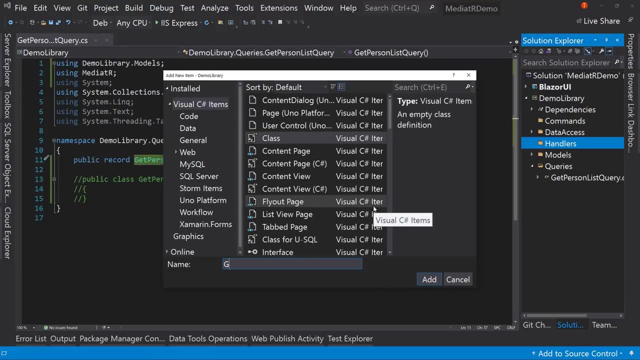 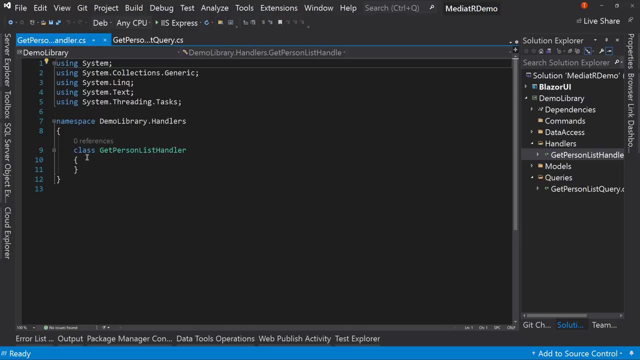 query will have one handler, not more than one, just one. so under handlers, let's create a class and let's call this the get person list handler, and in here we'll make this still a class. we're gonna change the record: public class: get person list handler. 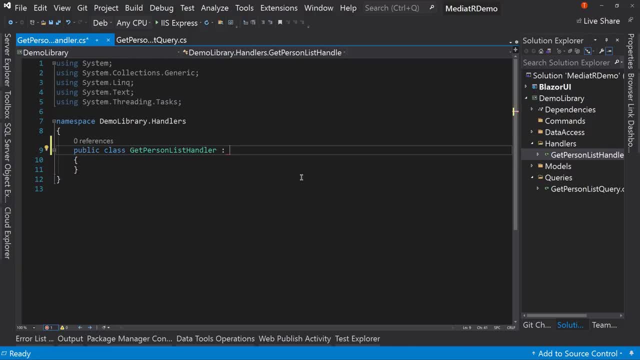 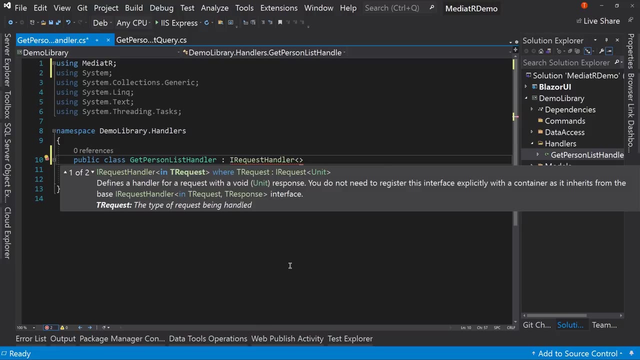 inherit or implement. sorry, not inherit and implement. i request handler that's going to add the using up here for mediator and then we have to pass in two generics. well, potentially two, you can pass in just one, but in our case we have a return value, so we have the get person list query, the pass in. this is what you're going to handle. 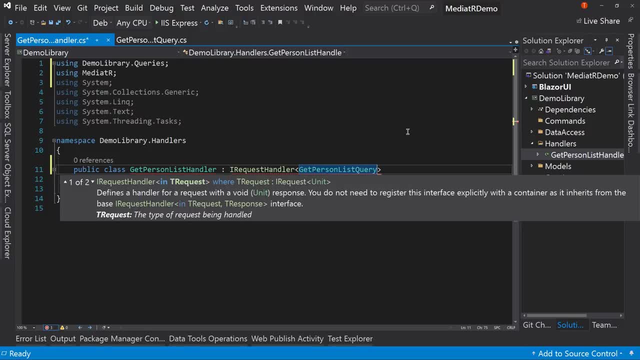 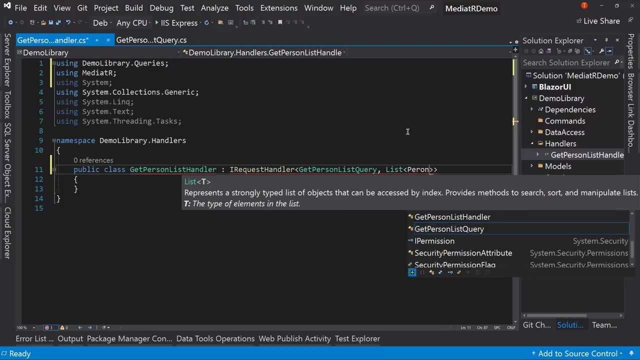 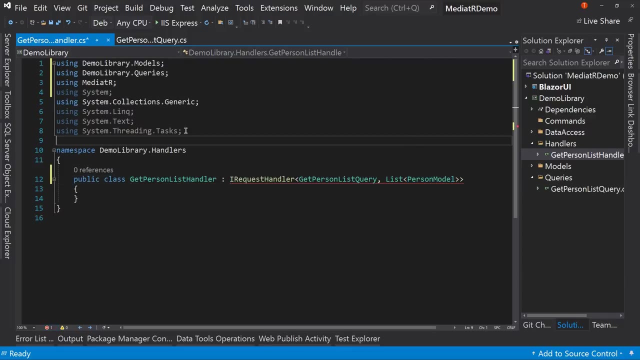 well, you're going to handle the get person list query but if you have an output, you're going to output that value. so, list of person model. that's going to add a using statement for that as well. so notice up here, my usings are probably a little different than yours, if you didn't. 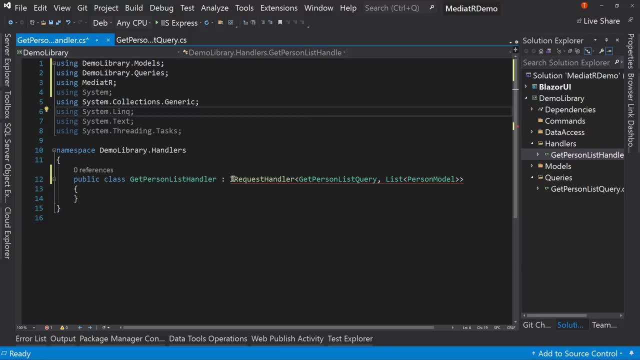 have that auto ad, all right. so this i request handler, which is different than i request, the i request handlerThe I request handler is for the userwhich is not an ID нельзя to use which is different than i request. the i request is is for i requestAnd my IDI further show that the html is a valid id. the HTML files having Handler here, nerve side of that, and we're going to need to add this in of the key for terminal. 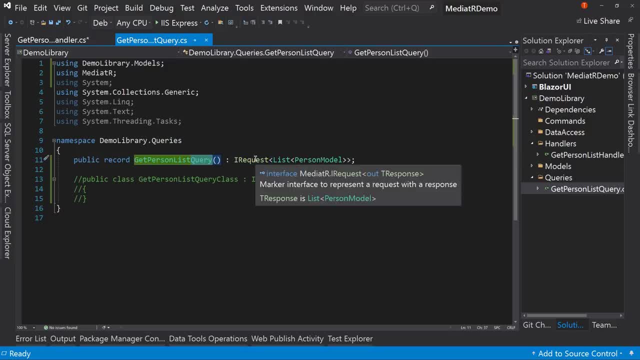 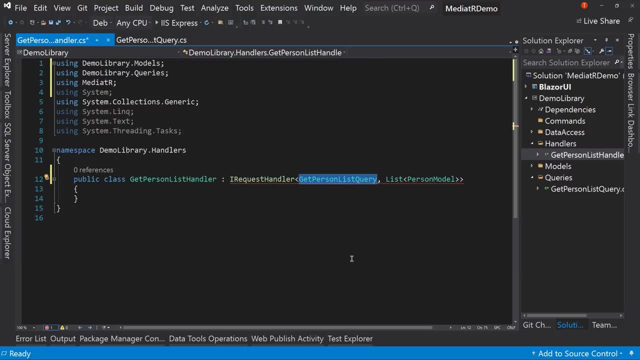 request is for your queries and your commands, But then on the other end, we're going to handle that query or that command. You pass in first which one you're handling and then, optionally, you pass in. you say what the output is going to be. In our case, the output is going to be a list. 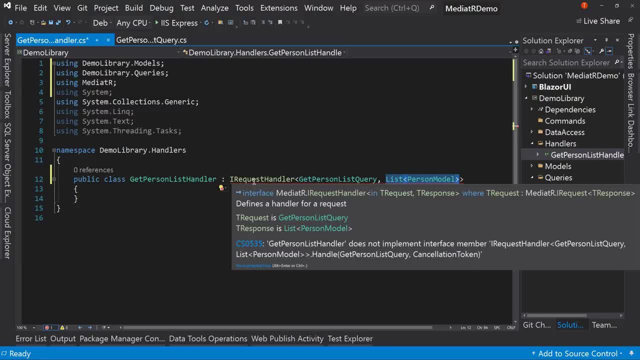 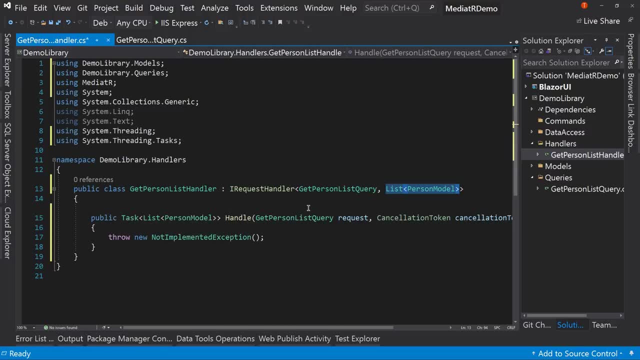 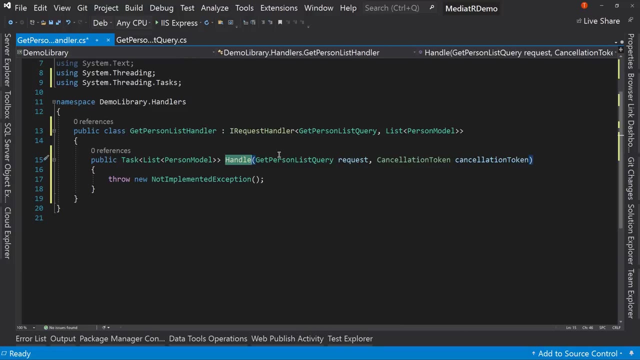 of person model. So that's our I request handler. Notice it's yelling at us because we have not yet implemented it. Well, if we implement this interface, it's going to add one thing: a handle method. That's it. And now note- let's unpin this- that the handle method you pass in your request. 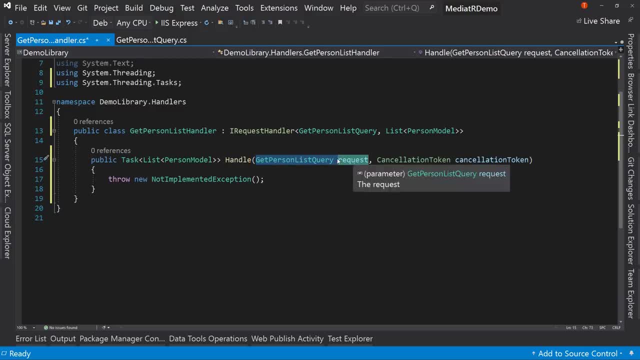 which is a get person list query. That's any data you need for the request. We also have this cancellation token because everything is asynchronous in mediator, So that's really nice because it just makes life easier. but you can pass in optionally that cancellation token And then the return is. 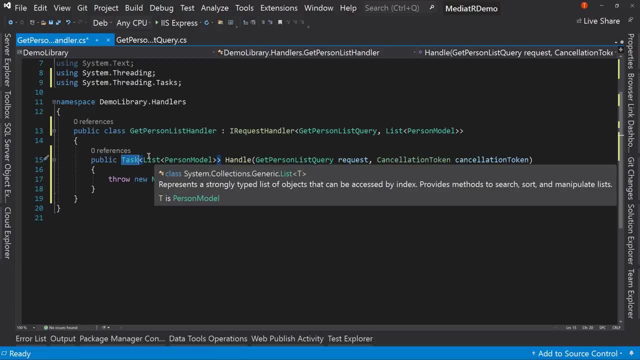 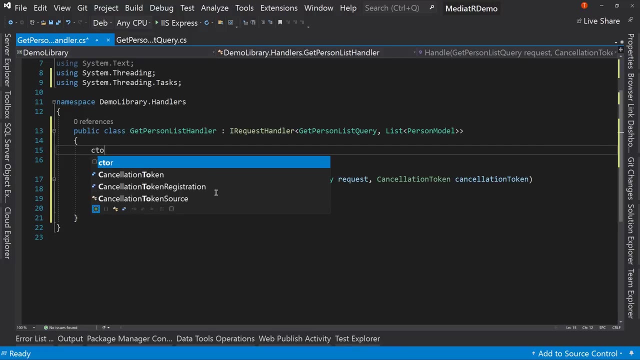 going to be a task is because it is asynchronous of type. list of person model. That's our output we expect. All right, So that's all we have to implement. for this, I request handler. So let's implement this. We first need to have a constructor CTOR where we need to pass in our I. request handler. So let's implement this. We first need to have a constructor CTOR where we need to pass in our I request handler, So let's implement this. We first need to have a constructor CTOR where we need to pass in our I request handler, So let's implement this. We first need to have a constructor CTOR where we need to. 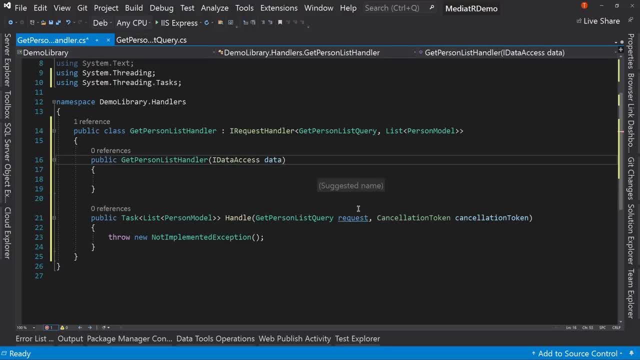 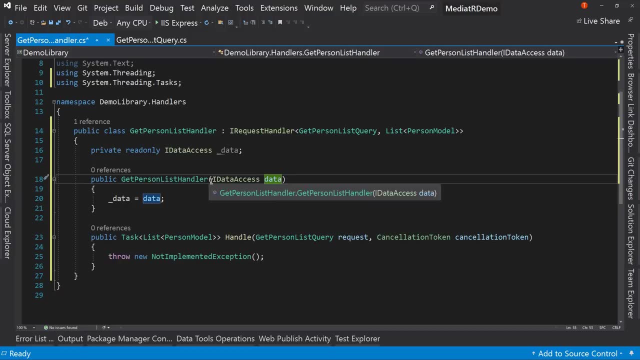 data access And we'll call this data And we'll do a control dot to create and initialize a field, underscore data. And you may say: well, Tim, where is that coming from? Well, this is dependency injection. So we're going to have dependency injection inject into this, an IDataAccess. 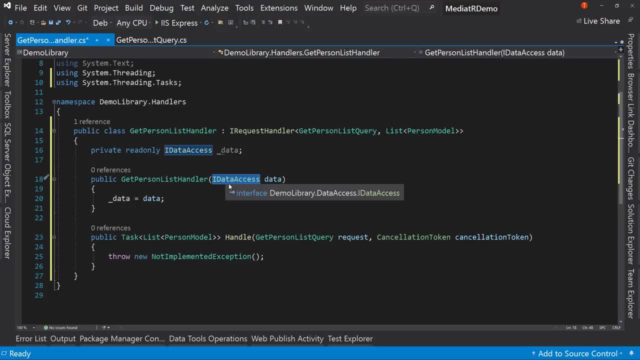 Mediator does not replace dependency injection, It just adds to it or improves it. So we can still use dependency injection to get the final details. we need In this case in our handler. we need to know about our data access layer So we can. 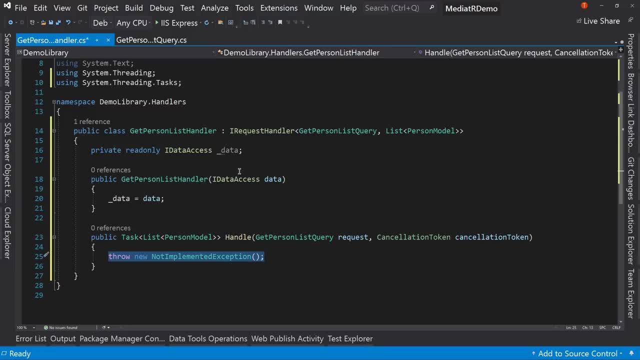 say in here: now return task dot from result. Now, this is kind of a- I don't want to call it a cheat, because it's not a cheat necessarily- But what we're doing is we have a synchronous call, not an asynchronous call, And yet we need to return an async value, something we can await. 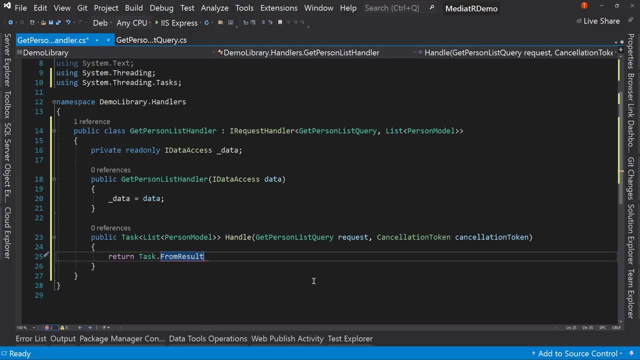 And so you say: task dot from result to pass in your synchronous result And that will turn it into an asynchronous call. It's not actually putting on a different thread. It's not doing anything like that. It's just saying it's wrapping our result in a task. That's all it's doing And it's a. 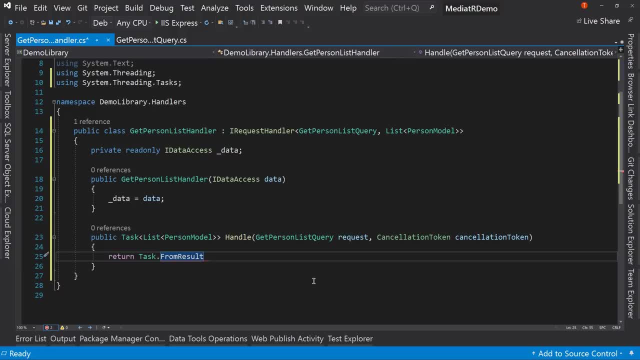 completed task, So it's complete right away. It's just a little bit of syntax sugar here to help us properly return a task. So in here we say underscore data dot get people And that get people method is going to get that list of. 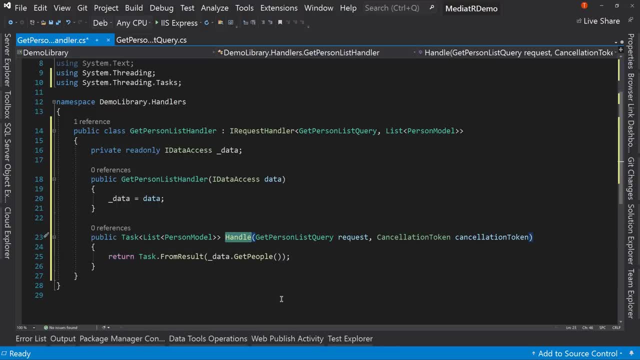 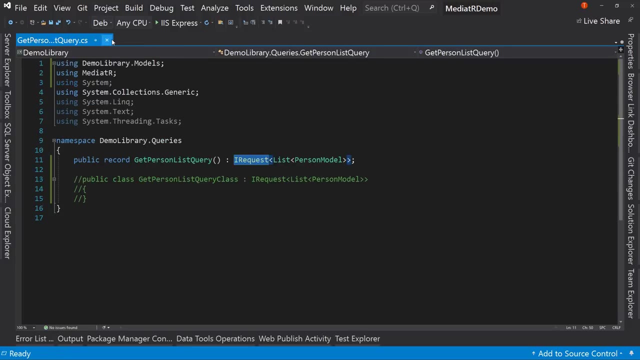 people. We'll return that in our handler. So now our handler knows about our data access, But that'll be the only place that knows about data access is our handlers. All right, So we have our handler, We have our query. Let's go back to Solution Explorer. 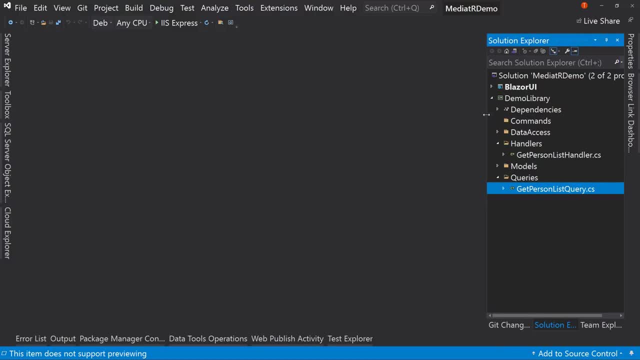 We'll pin this back on And we're pretty much done in our demo library for our first take at our first use of Mediator. Let's go back over to our Blazor UI And the first thing I do is configure startup You need to bring in. 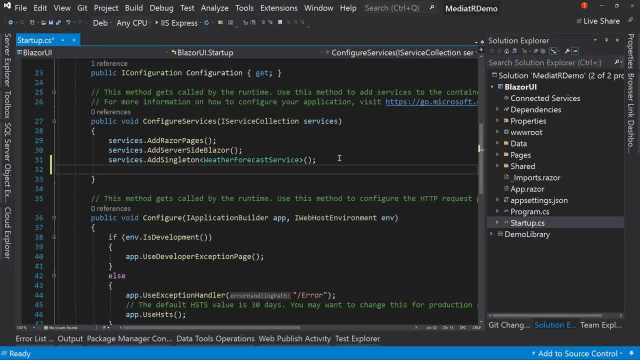 that data access. So services dot add singleton Now. normally, when we have data being stored, we're going to have to use a singleton, Because a singleton means that everyone has access to that data. It's not going to be refreshed throughout the life of our application. That can be really bad for a web application, because when I load it it'll be the same as 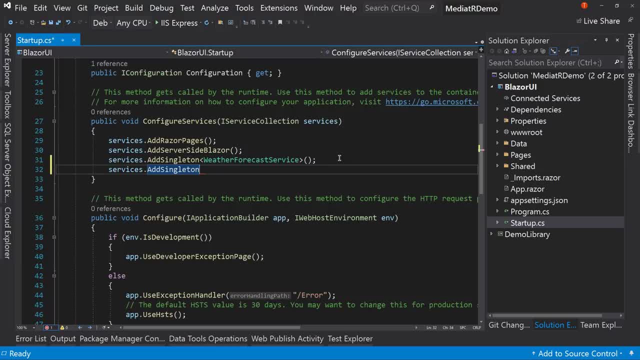 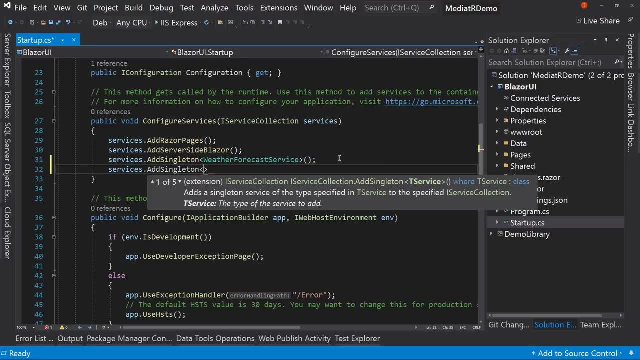 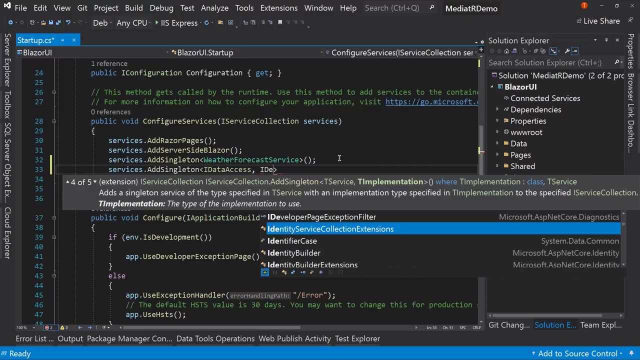 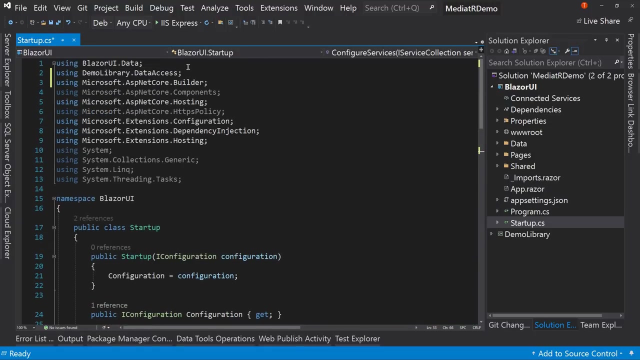 when you load it. But in the case of a demo like this, it's perfect because I can actually have my data persist. So add singleton for IDataAccess, Add the using statement And I- I'm sorry, not I- demo data access. That's going to map those two. And notice up, here we have our 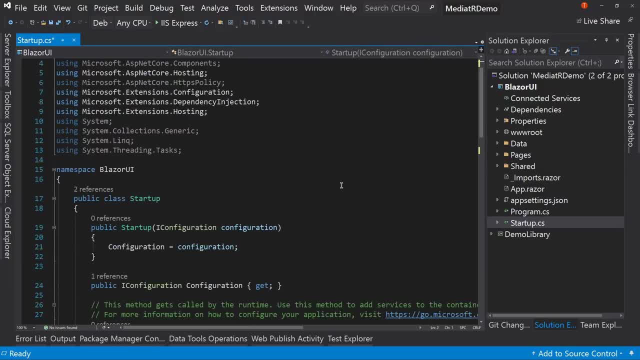 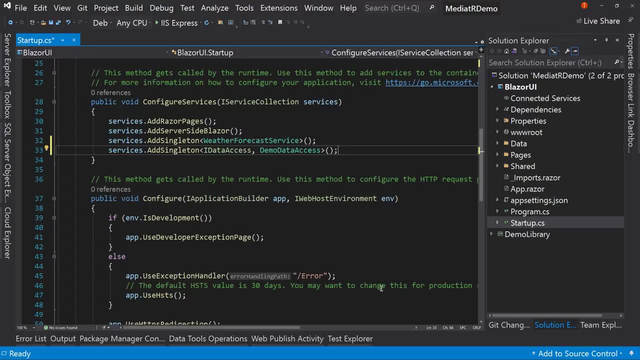 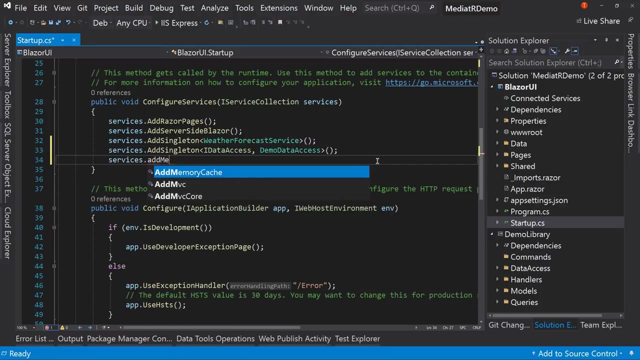 added using statement for demo library dot data access. So that adds our our data access to our dependency injection, but we still need to add Mediator and all the things in demo library. Now this is where things get a little interesting. is for Mediator. you can say services dot add Mediator, which I have not installed Media yet. So that's why it's not even coming up. 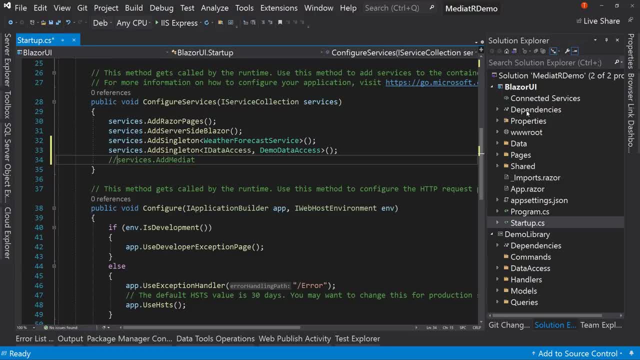 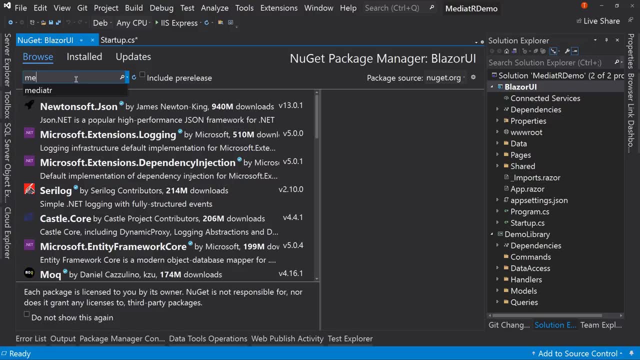 Well, let's do that. Right click on dependencies for our UI and say manage NuGet package, And we're gonna search for Mediator Events instead of this main one. I want to include this one here, So we're going to call this pretty. 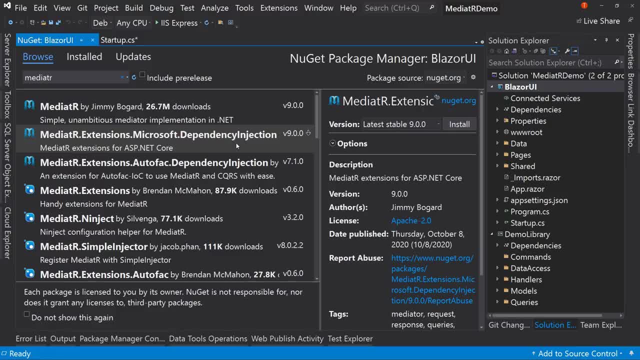 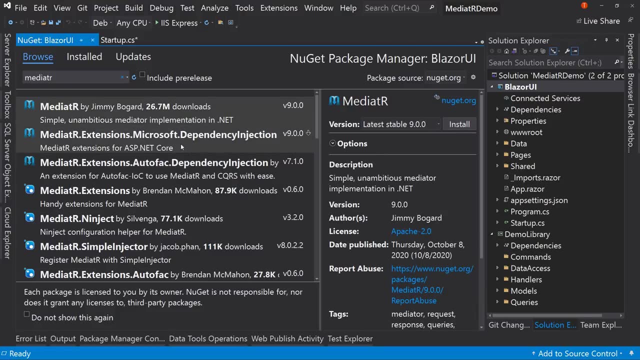 This one instead: mediatorextensionsmicrosoftdependencyinjection. This will allow mediator to work in our NET core dependency injection system easily. Now this is going to install the base mediator package as well, So let's install that. accept the terms. 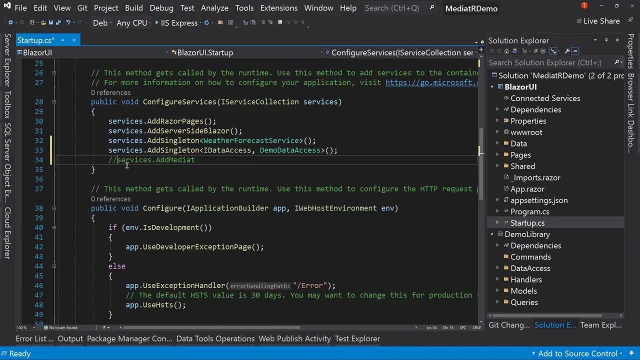 Once that installs, then we can come back over here: Add mediator. Now for adding mediator, we're going to say type of to get an assembly, But this can be a little confusing. You have to grab a class in here. For example, I could grab the get person list handler, or I could grab the model here, or I could grab even data access. 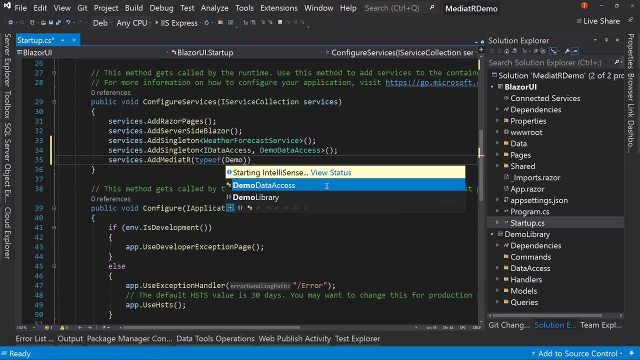 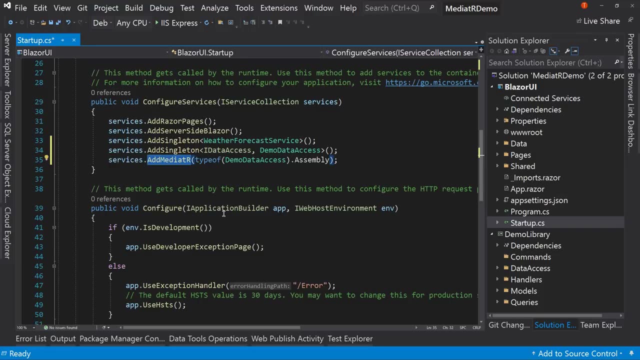 So I could say demo Data access and then say assembly, Okay, that's not going to load, just demo data access. That's going to load the entire assembly, and look for anything to do with mediator, which is going to be anything that is a handler, a query or a command. 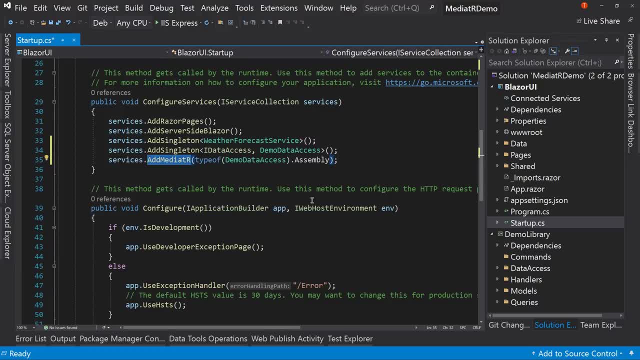 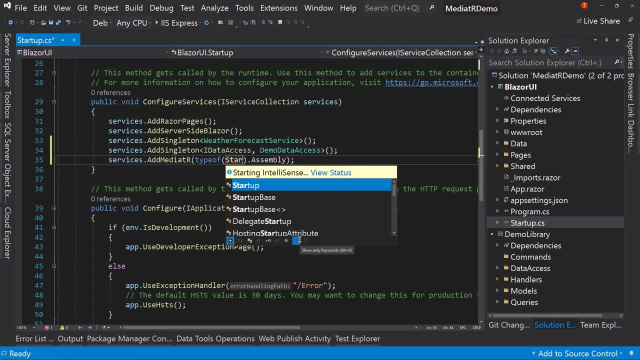 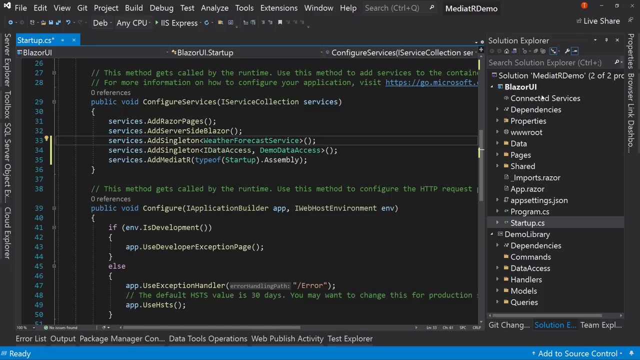 At least in our example. there are other things that mediator will look for. Now, if they were in the same project you are. typically what people do is, they say, start up, which is the class you're in. but that would be this Blazor UI and that's not where our mediator stuff is. 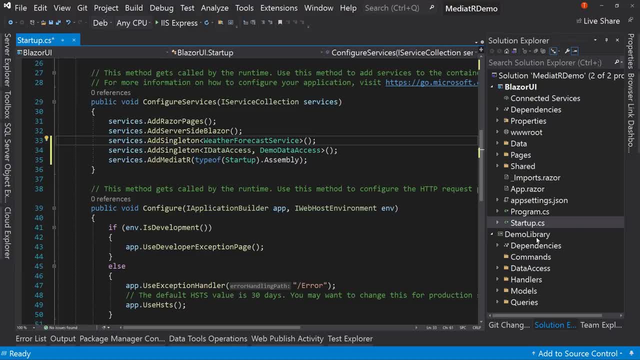 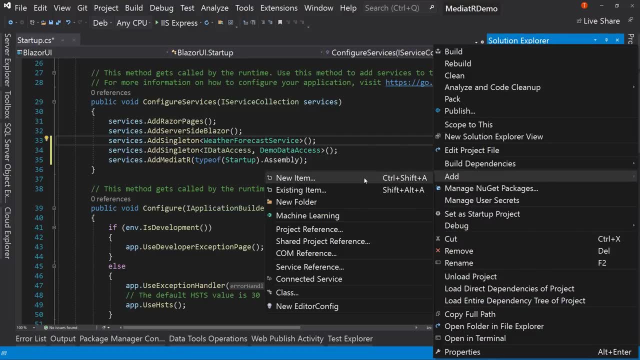 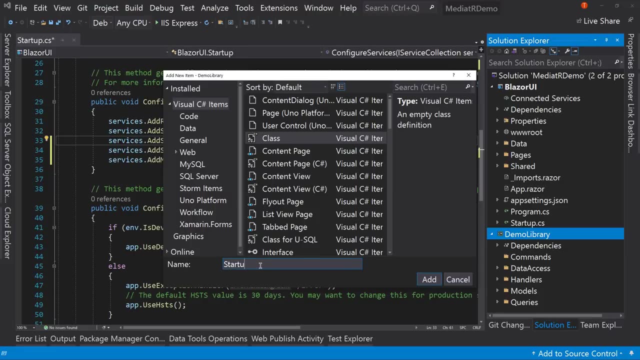 We have it in the demo library, So what you can do. this is questionable if it's a best practice or not, but it is. it makes it easier to read If you can create in the root of your demo library a class and call it start up, or you can call it something else. 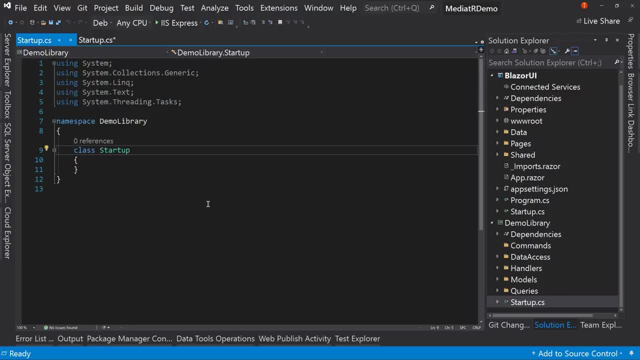 You could call it um mediator entry point or demo library mediator entry point. It's up to you. In fact, let's do that. Let's call it demo library mediator entry point. That is really clear what it is. We'll hit control dot to rename the file. 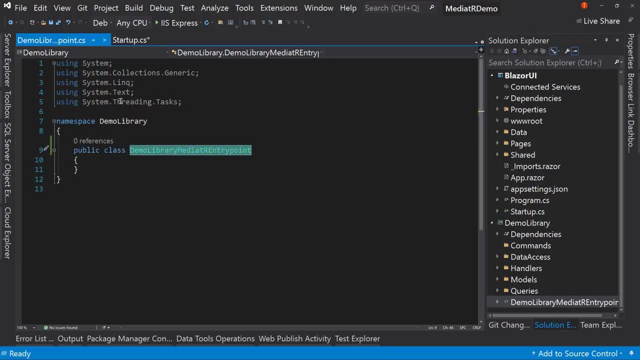 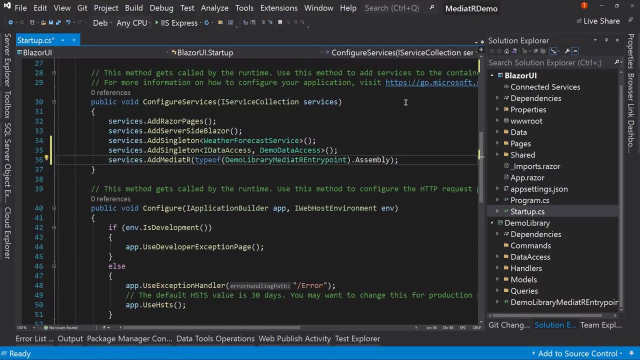 And now we have this file in there. We can grab this, copy it and go back here And we'll paste that in. We have to do a control dot to add a using statement. but now we know this: demo library mediator. entry point is for the demo library. 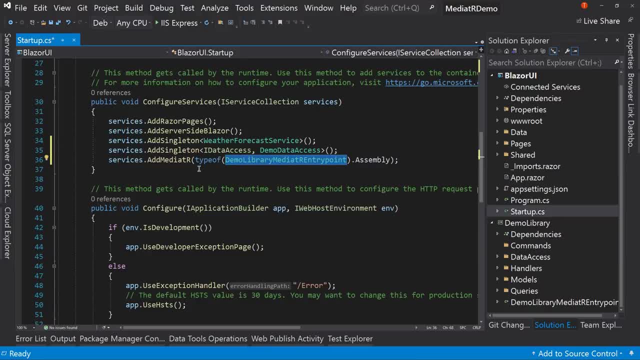 So it's very clear what we're adding to our mediator. All right, But again, that's not adding that class, It's adding the entire assembly. So now mediator has been added to our dependency injection system, along with ID to access, because that's necessary. 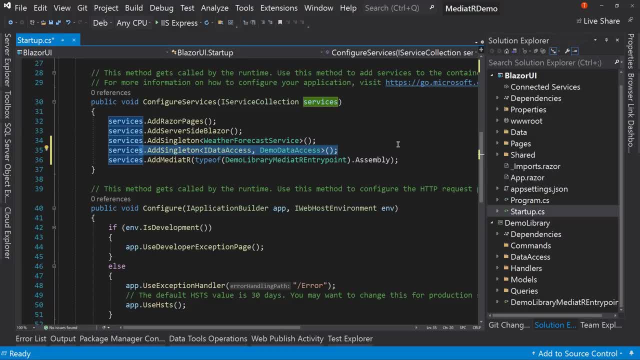 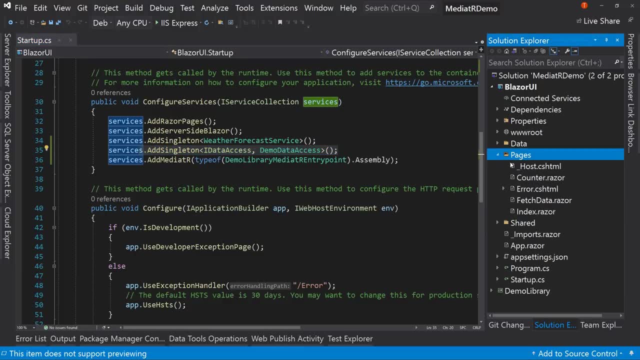 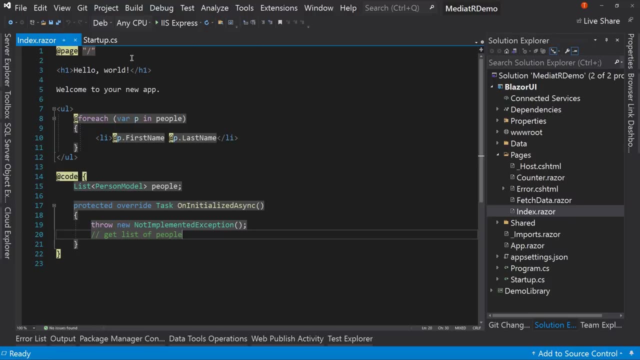 For the um, the handler. Now we can go over, we can save this, We can go over to our page, our index page, where we're already set up to call our mediator. So you first have to inject something. Now 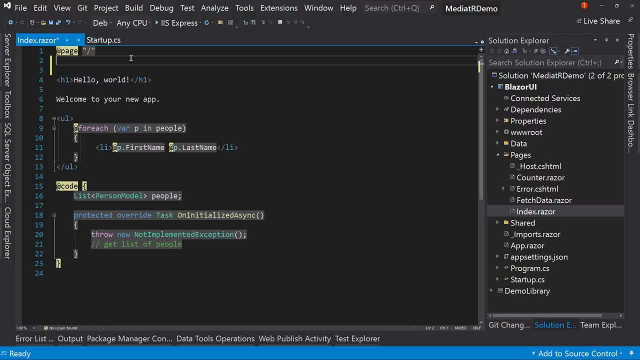 remember I said that as your complexities grow, your list of dependencies you inject into any given item or class is going to grow. Well, with mediator that shrinks right back down to one inject mediator dot I mediator like, so it will call this. 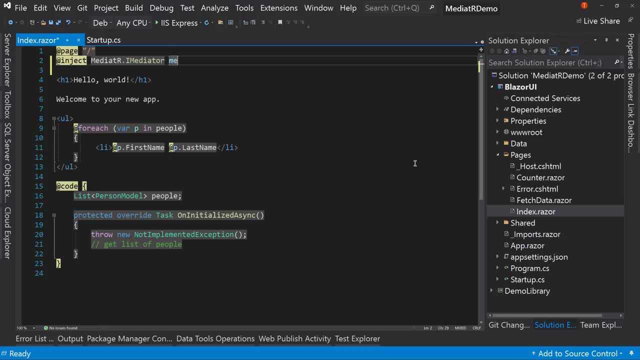 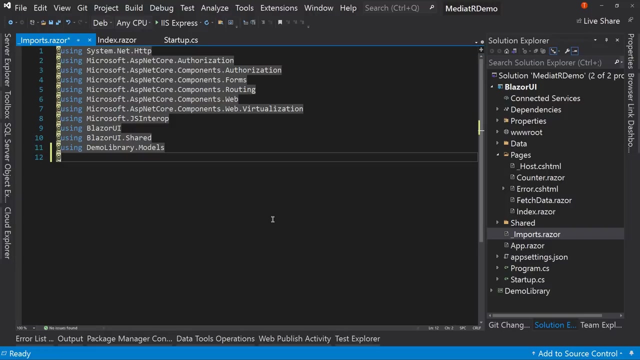 um, let's call this a mediator. I left it at underscore like so, and now we can use this mediator to find what we need. Now we also should go to our import statement and add some usings. here We have the models already: demo library dot. handlers. demo library dot. 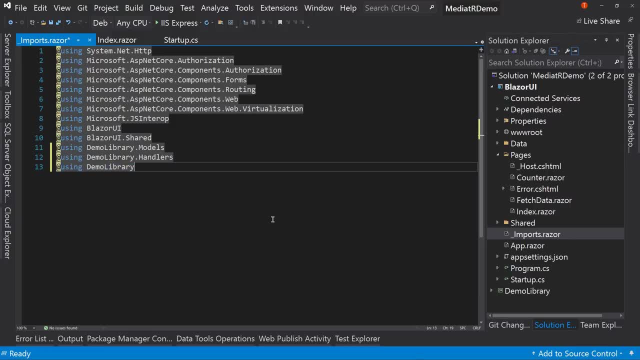 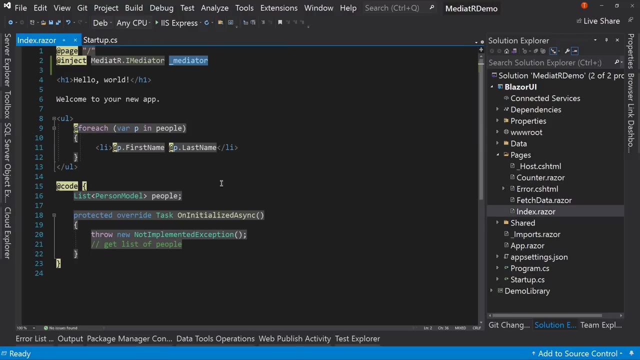 Let's just copy that So it's a little bit faster. dots, uh, queries, And that's all we have actually for now. Um, we're going to have commands soon, But we don't have them yet. All right, So that's gonna make our life a little easier when it comes to. 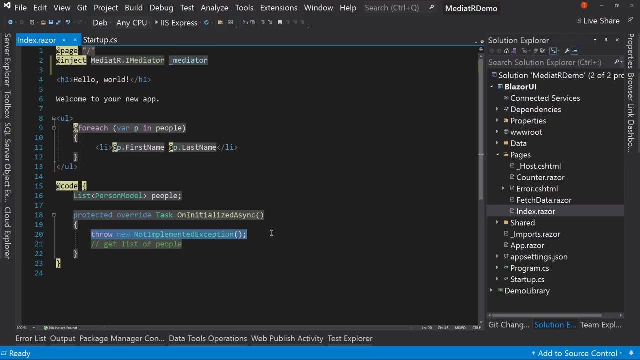 um, doing these calls here. Let's get rid of this. throw exception in the comments and let's put our code in there. to talk to mediator. We'll say: people, that's where I assign it to. equals a weight mediator. Whoops, We have to say. 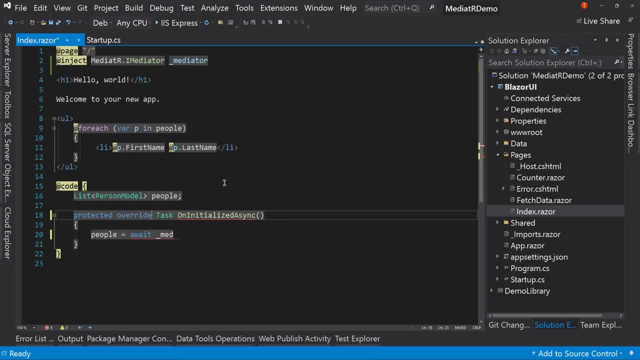 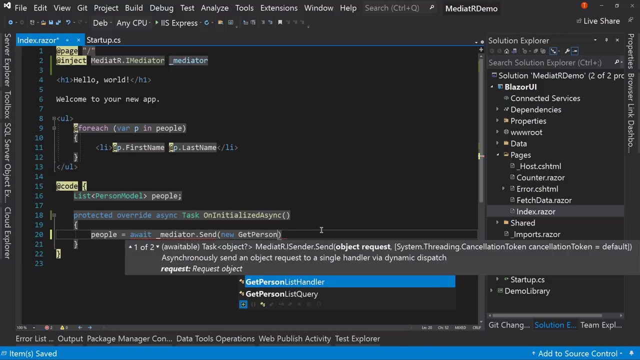 uh, override Async mediator dot send. Now the send command is the only command you really need, using this pattern of having a command or a query and a handler. Just say send new get person list query. Okay, So I've said: 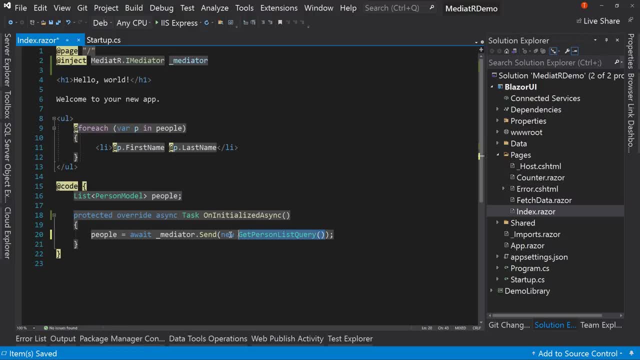 Hey, this is the query I'm going to do, which has all the data in it, which is nothing. I want you to send. that That's it, And the result is going to be: if you look here, it's gonna be a list of personal, actually a task of list of personal model. 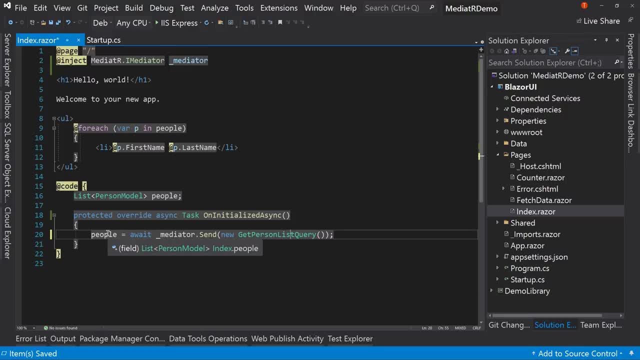 which we're waiting it. We await it. Therefore, people will get populated with a list of person model. Now I'm gonna run this, We're going to see it And then we're going to talk about it. So let's do that in that order. 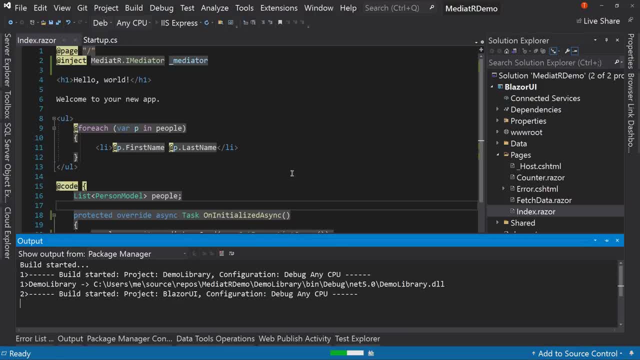 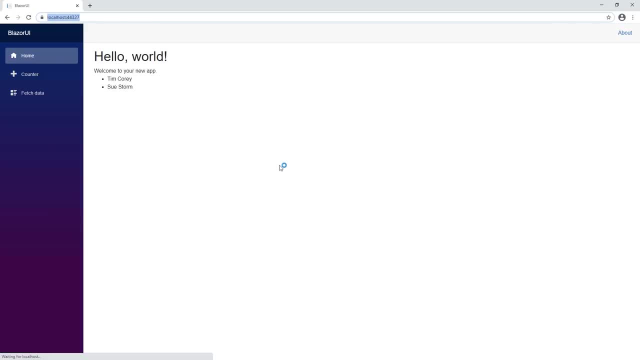 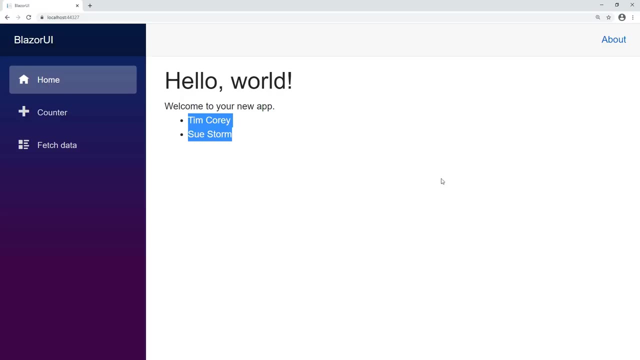 Let's run this, get this to go. Hopefully nothing breaks. There's our index page And, as you can see, hello, your new app. Tim Corey and Sue storm are on the list. Well, how did that work? Because really that's a pretty simple command. 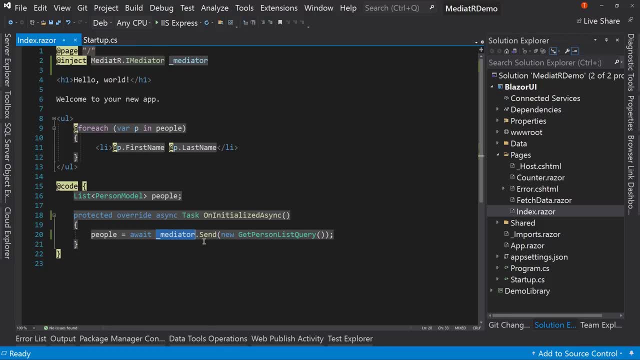 Well, mediator said I've got a new send request. You're sending out a request and the request is of type or the data is of type- get person list query. So it says who handles that. And if you go to the handlers here, 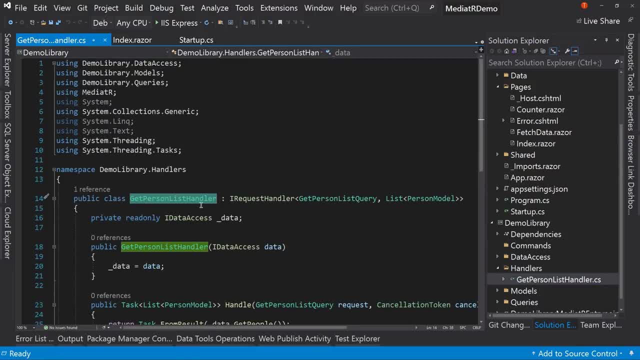 you'll see that the get person list handler, which I've conveniently named to correspond, but the this handler handles get get person list query. So it says: okay, you've asked for a get person list query, I've got the handler for that. 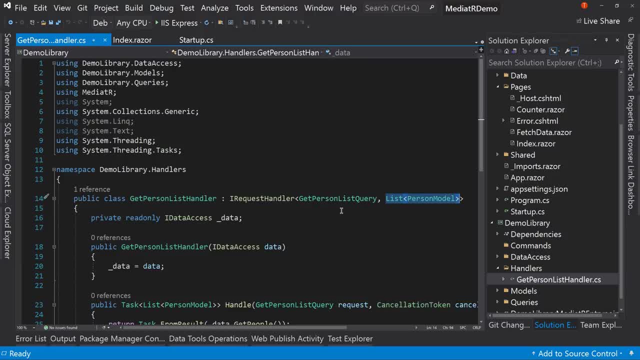 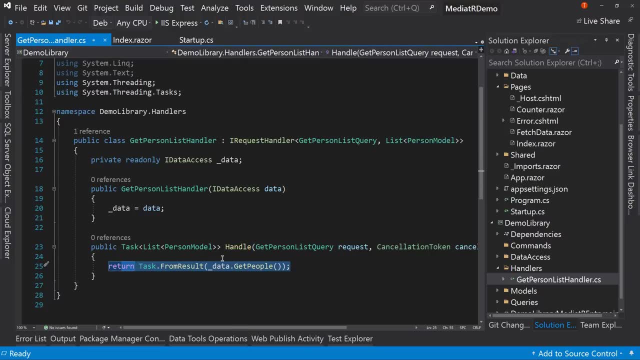 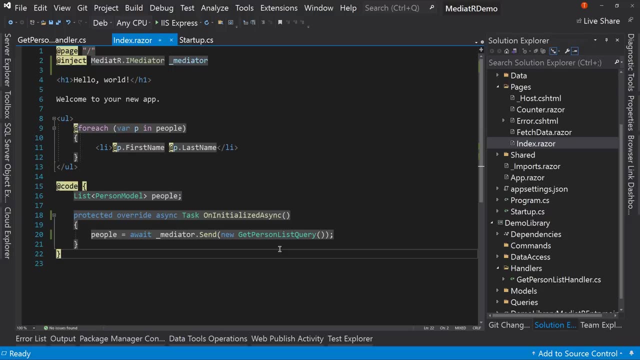 And, by the way, it returns list of person model, So you can know what it's returning, and it says, okay, call the handle method, do that work, return the values and boom, you're done. So when it comes to our actual index page, or whatever page we are in blazer, 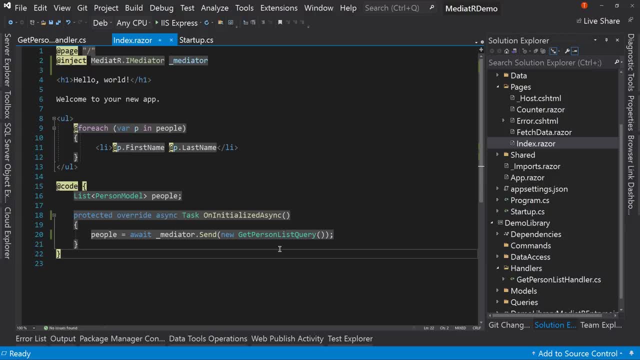 we're going to have a list of people that we've asked for a get person list query. So it says, okay, you've asked for a get person list query. The call to get data is that? right there, That's it. Now, our handler is quite small. 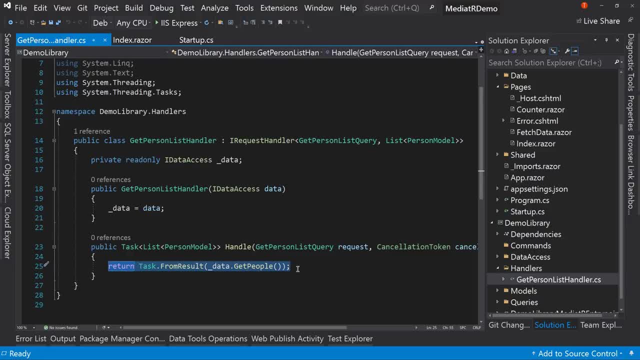 It's only doing that right there, when fact it could be doing a lot more than that. but let's just say it is. you know five, 10,, 15 lines of logic. We just have one line in our actual UI that just says: 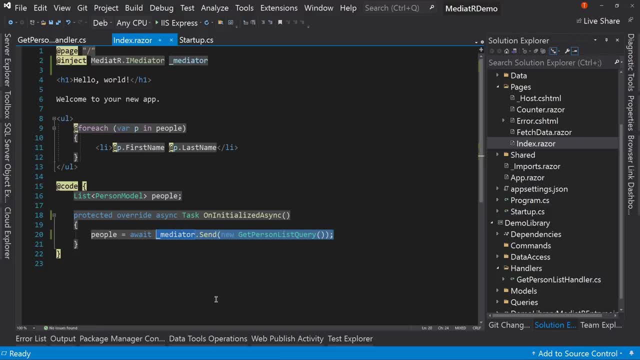 Hey, handle that. We've moved the complexity. We haven't gotten rid of it entirely. In fact, we've added some complexity, but we have moved it out of our user interface. What are the benefits of having this set up like this? 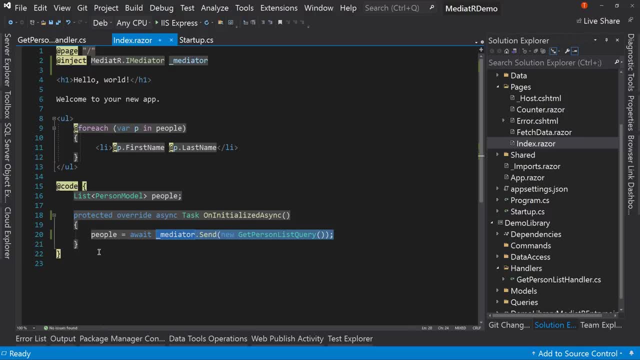 Well, our page. here there's no real logic. The logic is just do something, go do it and then display the values. If we get values office page, we just say: go use those. That would be all we would do. 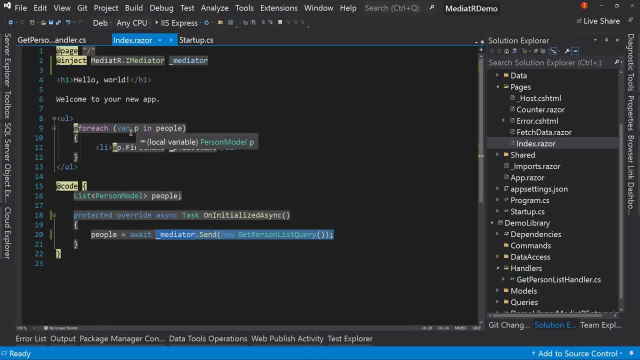 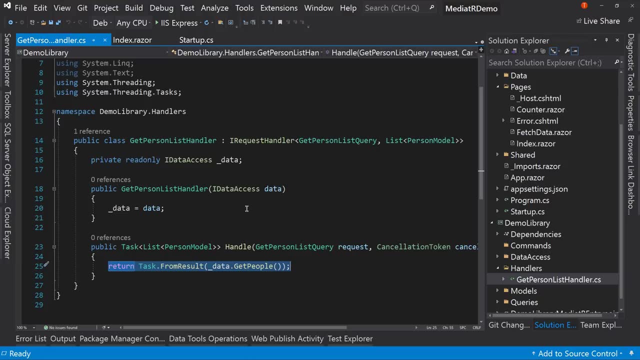 So there's not a lot of work going on here. Instead, the work happens in the handlers. but notice, the handlers are just simple methods that we could pass in, We could call. we can instantiate this class without mediator, which is the point. 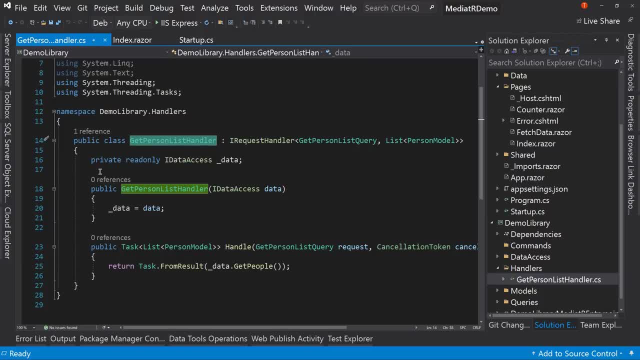 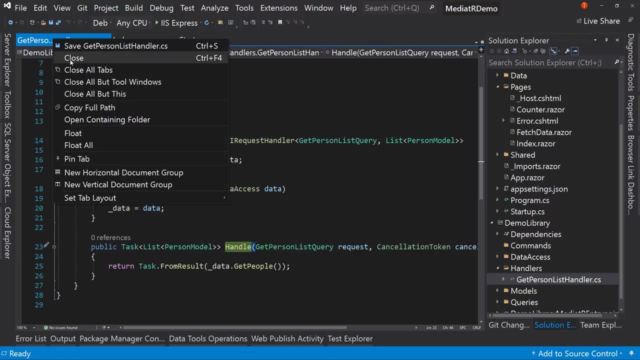 because now we can use unit testing to test this handle method. We can inject ID to access and we can test just the handle method for this, And it's very simple. Let's make this even more obvious how this can be helpful. Let's close all the tabs here. 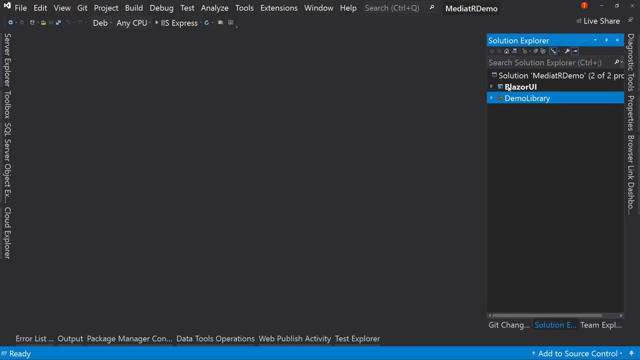 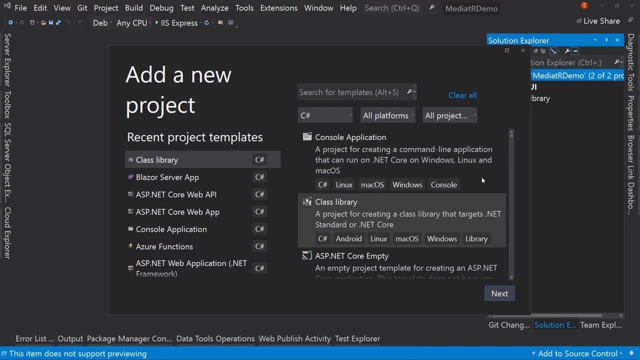 I am going to minimize everything here. I'm going to right click on solution and say add- we're going to add a new project type. Let's create an API project, So let's search API. We have ASP net core web API. 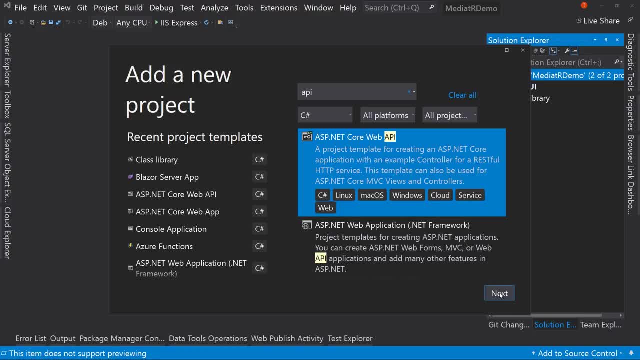 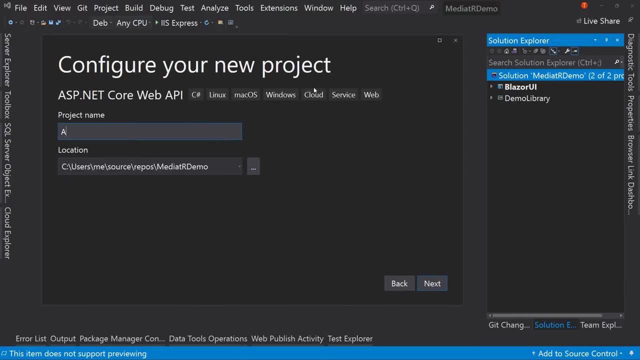 That's the only want, not framework core. Hit next and we'll call this our. we have Blazor UI, So let's call this our API or call it demo API. There we go. Demo API, Our naming conventions all over the place. 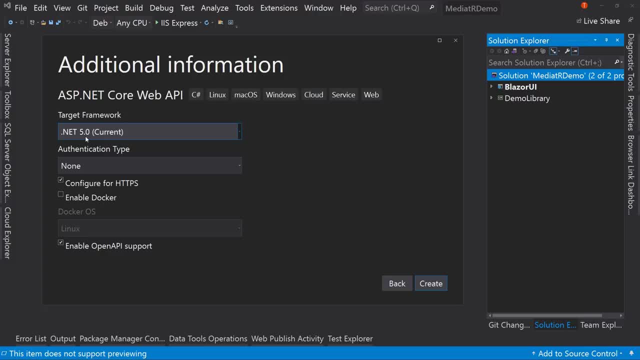 It's okay, It's a demo. Dot net five: Yes, No authentication. Yes, Configuration for HTTPS. Yes, No Docker and yes, to open API support. That'll give us swagger, which is very helpful for for this demo. 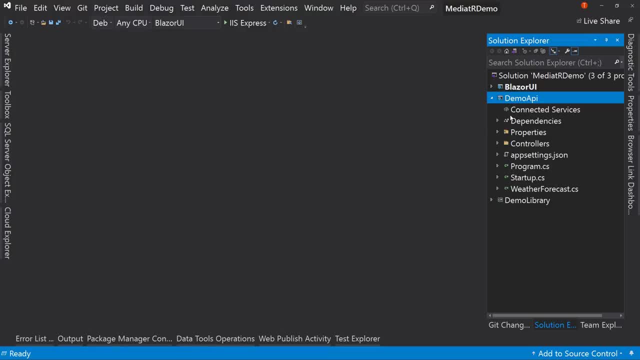 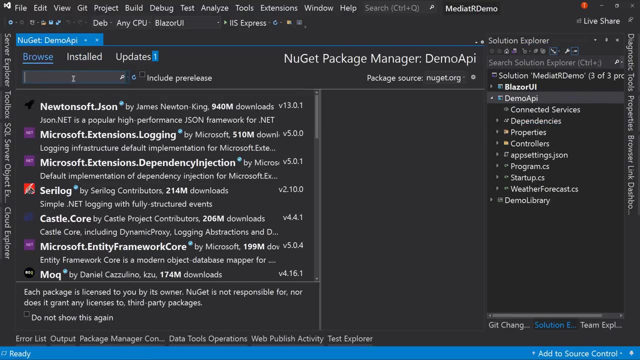 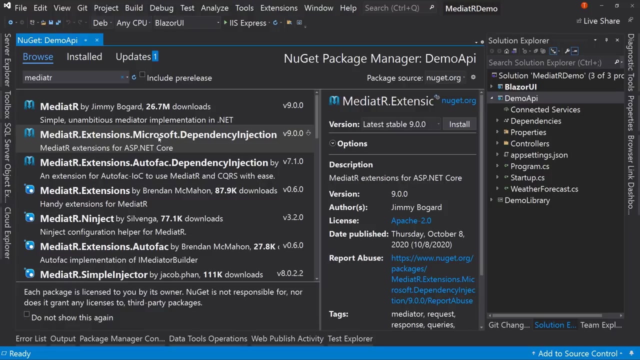 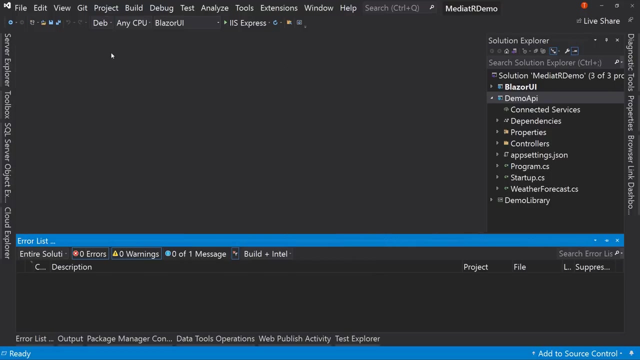 So basically all the defaults. it closes down right Clicking dependencies and say: manage NuGet packages, browse for mediator. install the mediator dot extensions, dot. Microsoft dot dependency injection that I accept And now we have mediator installed in our API. 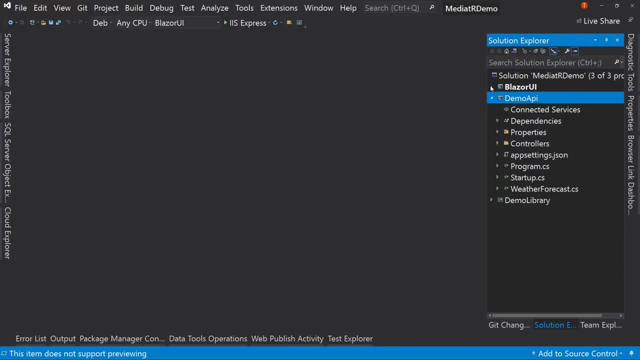 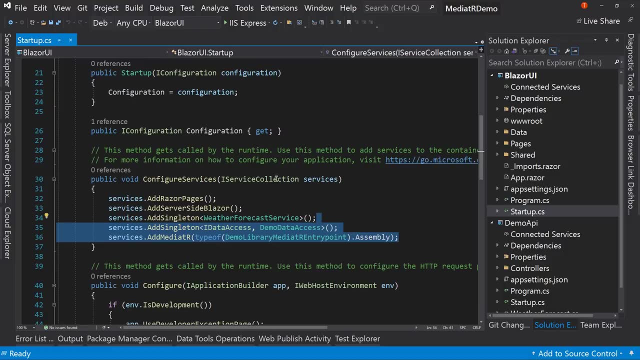 Now we're going to do is in our. let's go back to our Blazor UI and go to startup. I want to grab these two lines, just instead of cop, instead of retyping them, I grab them and go to our startup. and after the swagger gen. 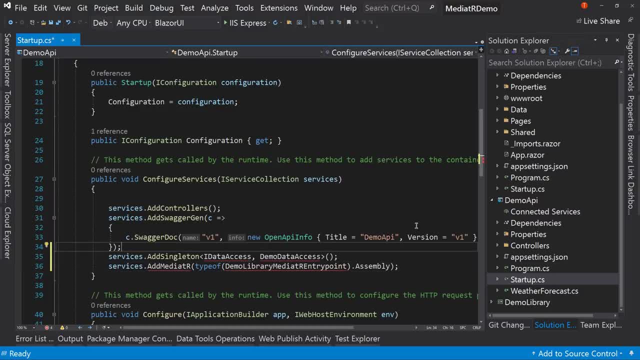 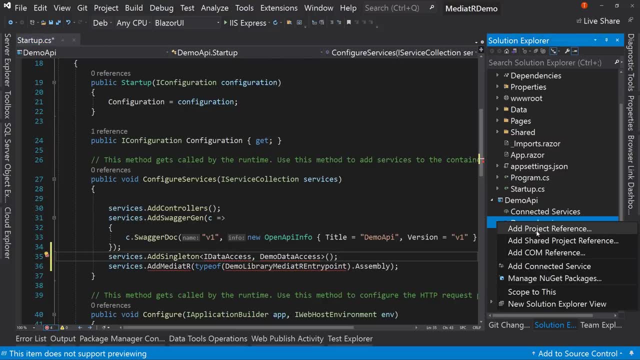 I'll paste those two lines. I have to add a. let's add the dependency. So right click on dependencies and say a product reference reference, the library, demo library, not the UI. And now we can say control dots to add the using statements here that we need. 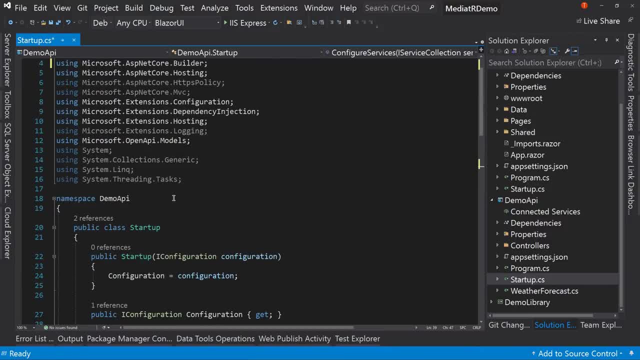 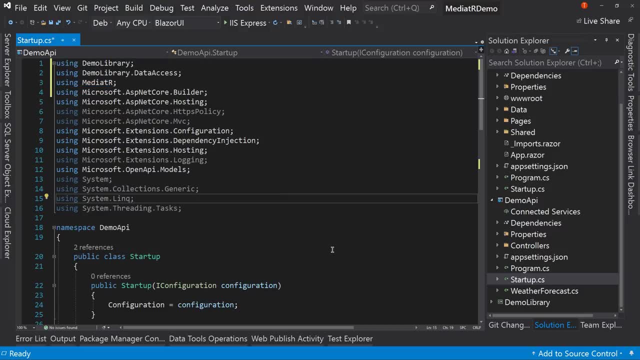 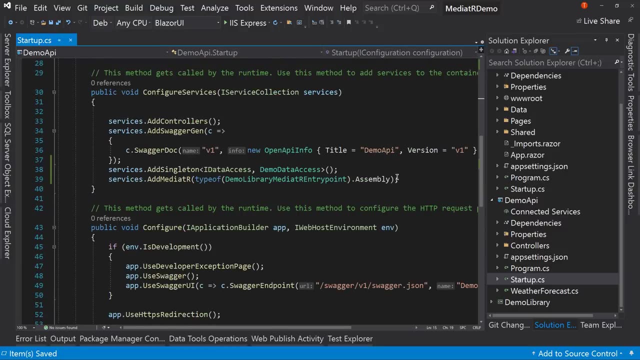 And that adds our various using statements. If you look up here, there's our new using statements for demo library, demo library, dot. data access and mediator. Save those We now have. we now have a full mediator implemented in this API, just with these two lines and the NuGet package. 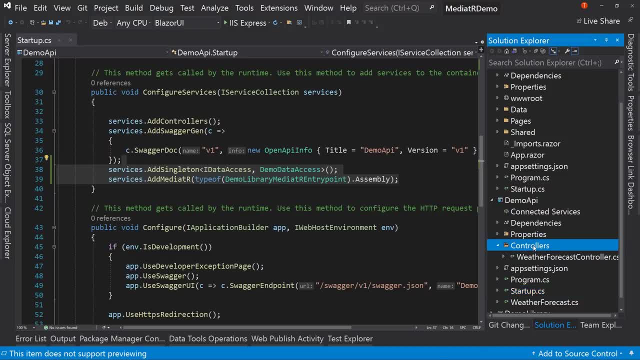 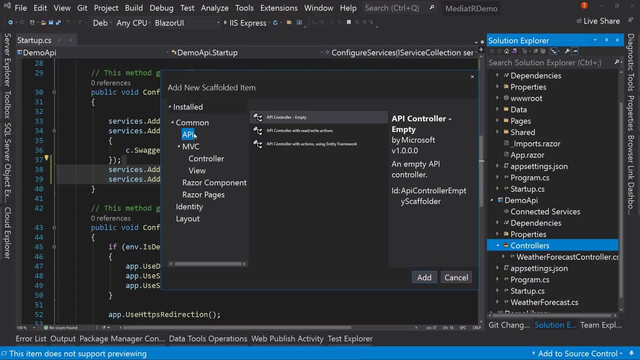 Now let's go to controllers. We can right click on controllers and say add new controller and we're going to choose an API controller. Sorry, it's a little small. I'm not sure why they're that small. We're going to choose API controller with read. 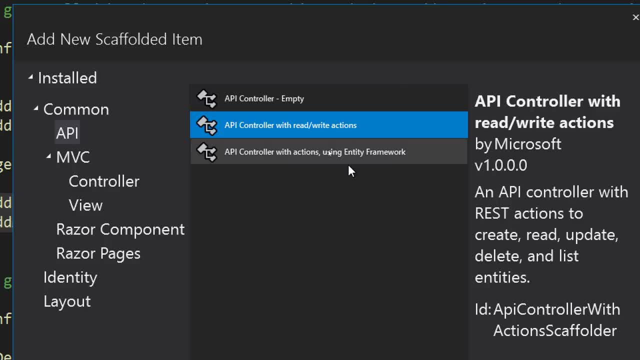 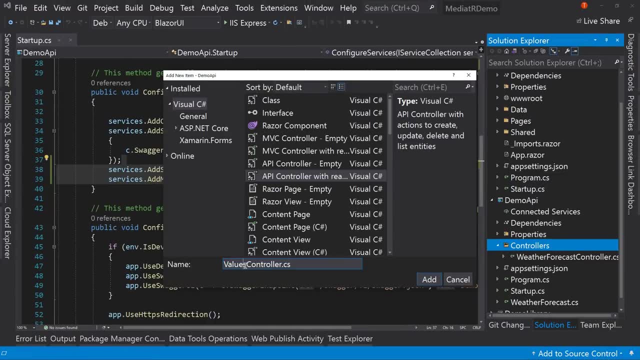 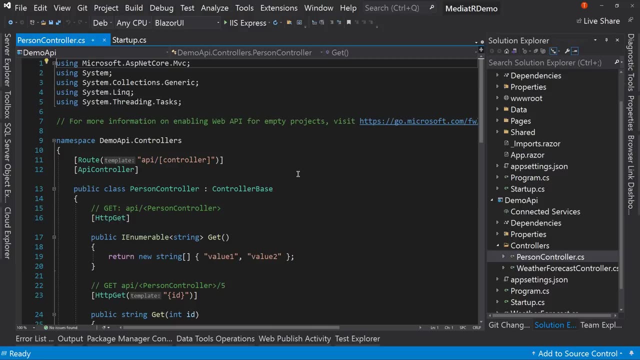 write actions. Now it's going to give us a demo to work from, which is just easier, in my opinion. Add, And we're going to call this the person controller, Okay, And it's going to scaffold out for us a number of commands. 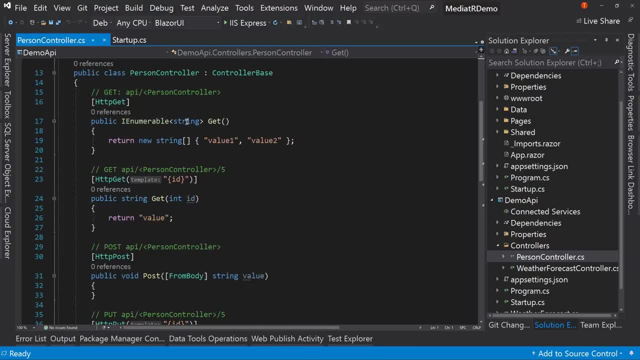 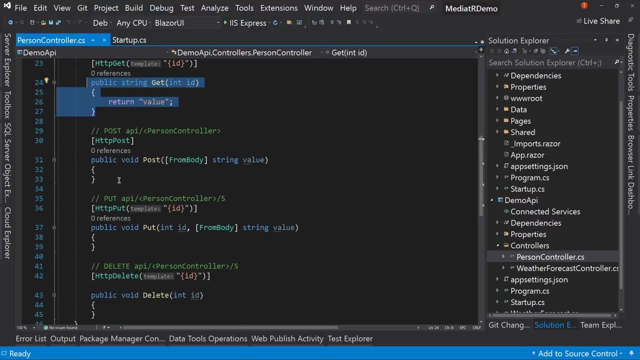 In fact all the the general ones. So we have our get, which is usually a list. We have our get by ID, which is usually one item. We have our post, which is kind of like an insert. We have our put. 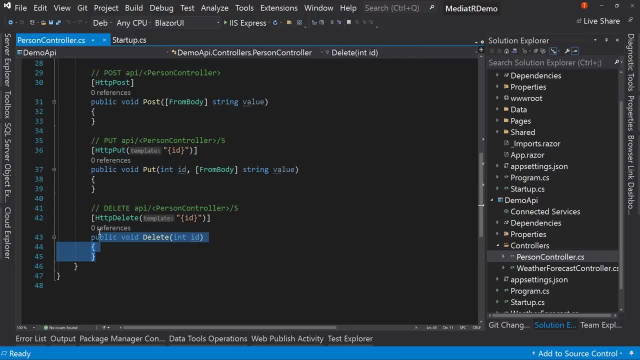 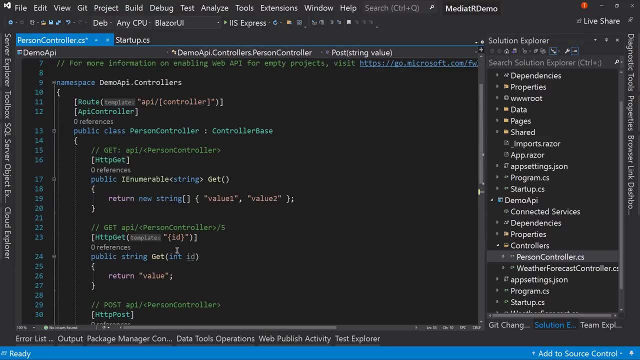 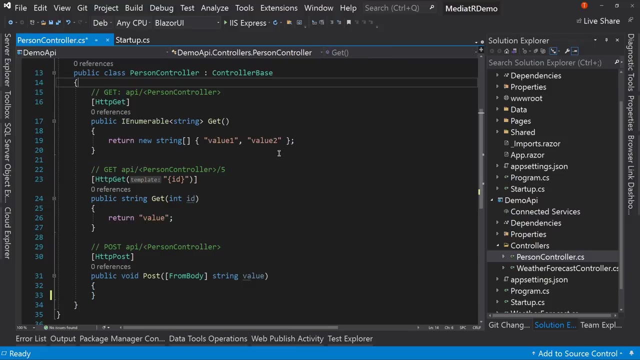 which is an update, And then we have our delete. Let's get rid of the put and delete and just have our our get, our get by ID and our post or insert. So let's talk about bringing in mediator. Well, CTOR to create constructor. 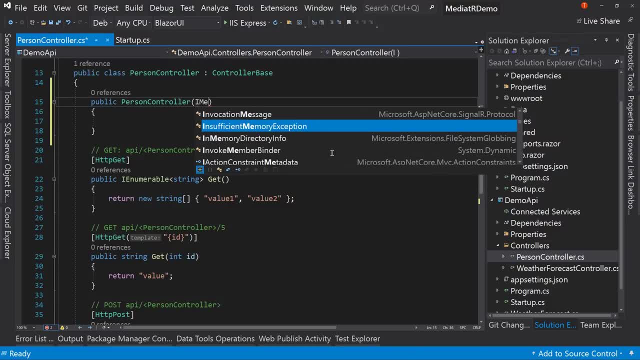 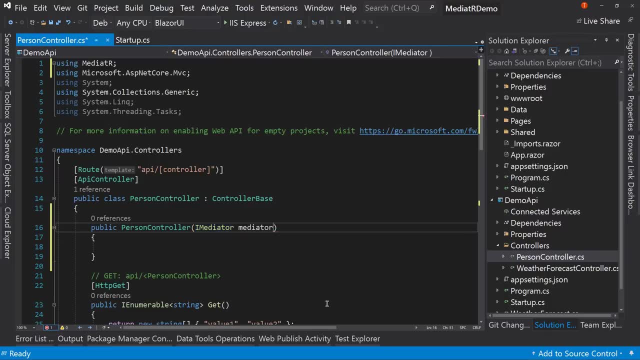 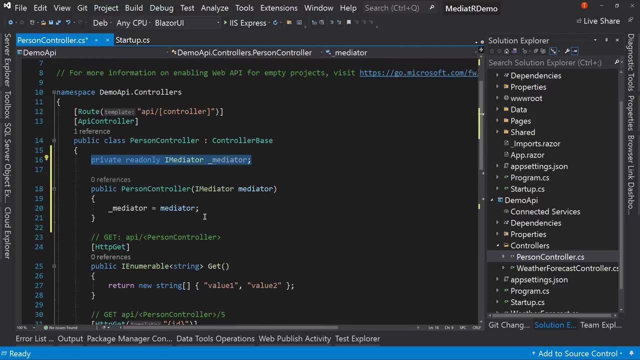 We're going to say we want the I mediator. It's going to add the using statement for mediator up at the top And we'll say mediator control dot. to create and assign the field for mediator, which adds that right there and that right there. 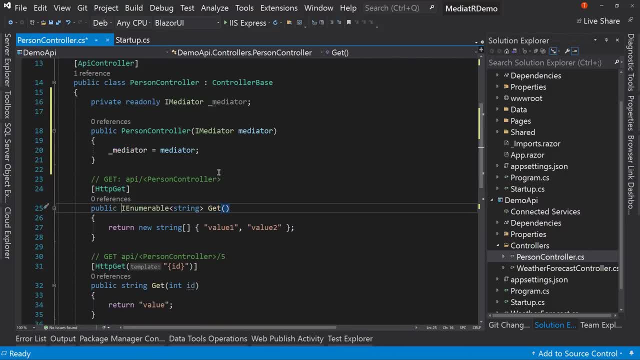 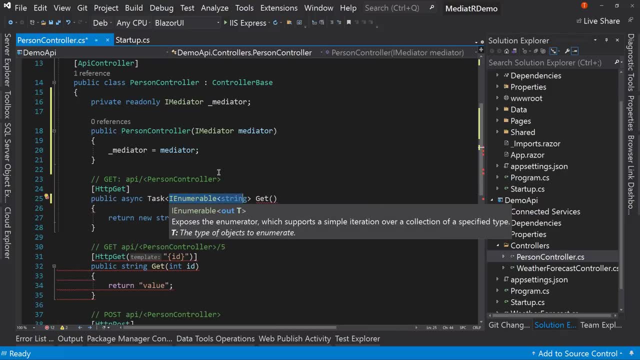 And now in our get command we can say: this is a async task of type, list of person model. They'll add the using payment we need. So it's an async task of person model. And in here we're going to say: 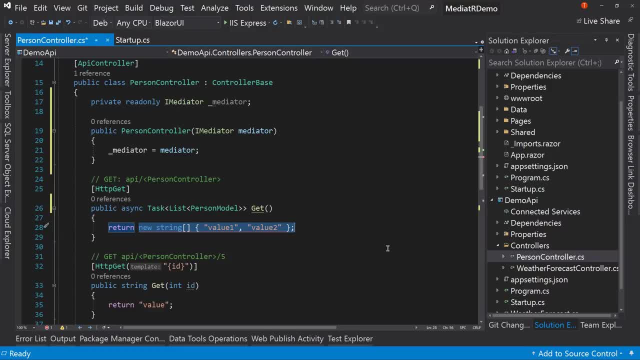 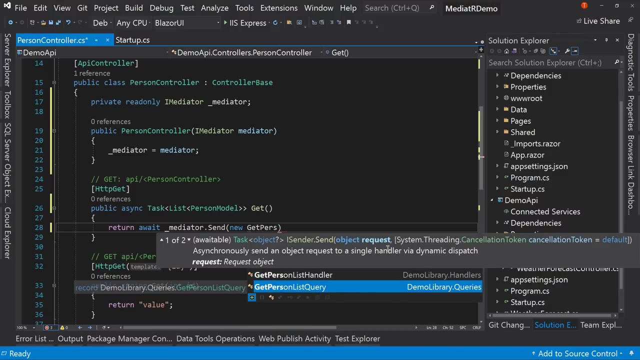 just like in our blazer app, we can say underscore: mediator dot send. Oops, we need to await this. Await: mediator dot send. We can pass in here a new get person list query. Okay, that's it. So now there's a few lines. 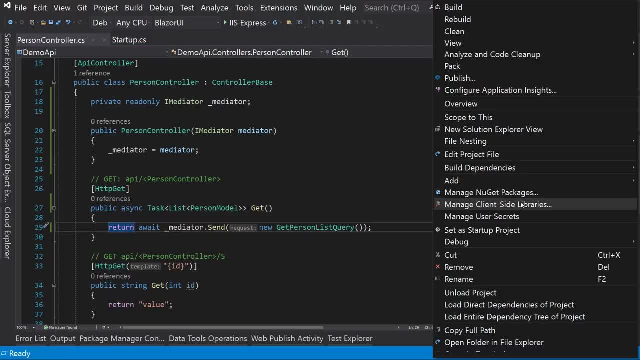 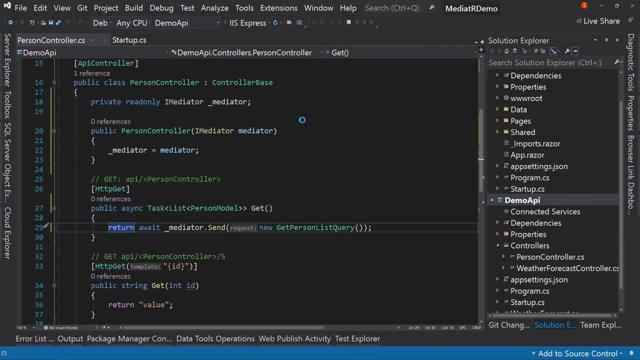 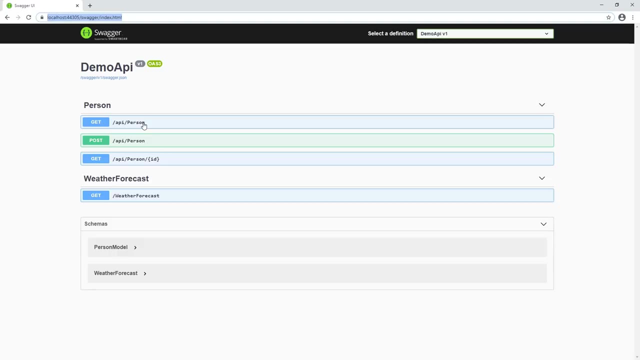 a few lines of code. If we switch over to this API as the startup project, So right click on it and say set as startup project, We run this. This will start our API, which will start swagger, which is really helpful. He's not going to say under the get for person. 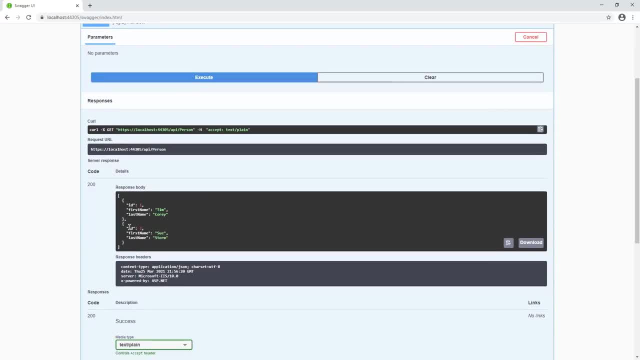 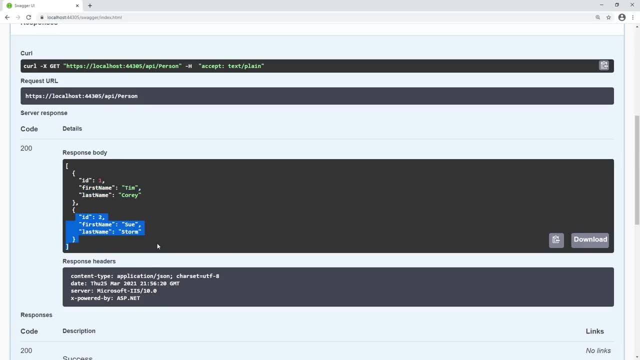 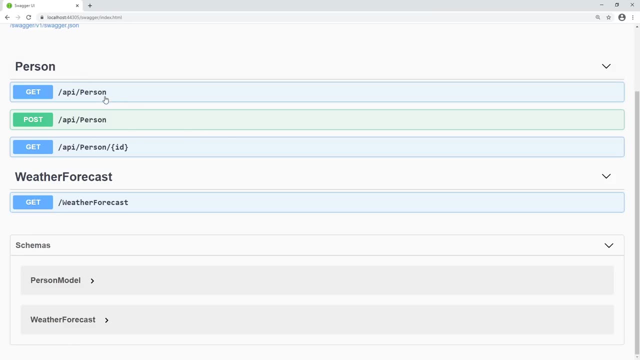 try it out, execute And you'll see here that we have under the body the response, Tim Corey and Sue storm Ids number one and two. so we are working. We have a a get command working in the API the same way we. 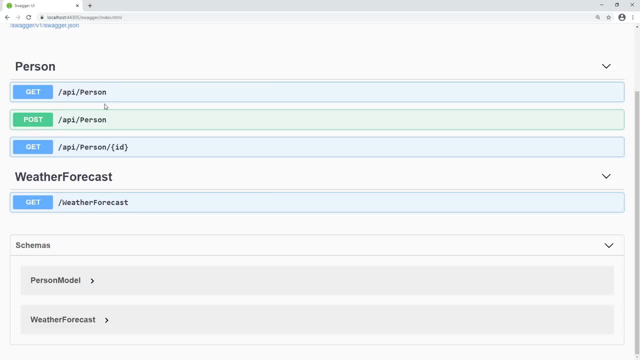 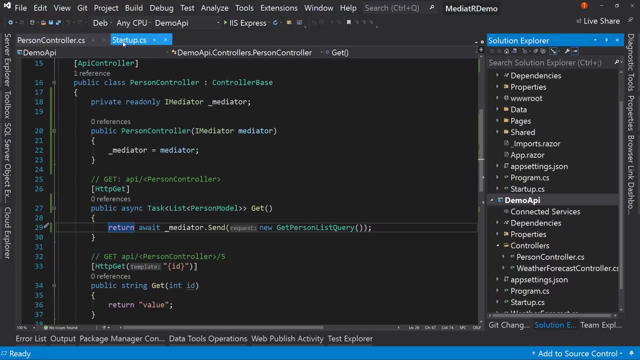 have it working in blazer with just a couple of lines of code And that's kind of the the. the awesomeness here is that because we're using mediator to load that entire assembly And because we are just saying Hey, 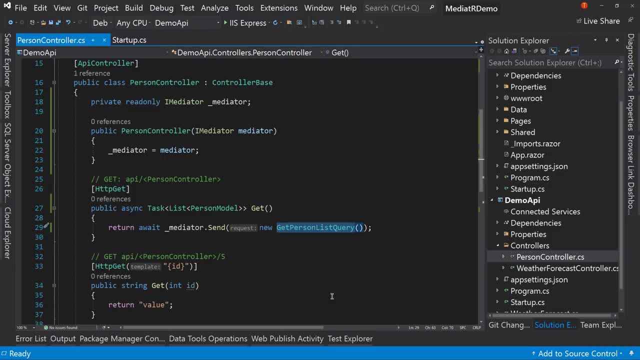 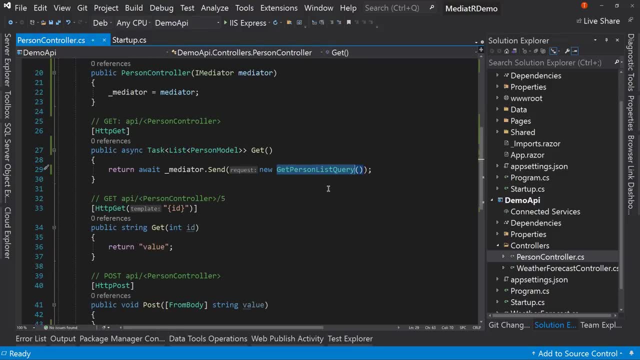 call that query, We don't have to think about the implement, We don't have to think about the implementation details in our user interface. And so when you talk about really thin API controllers- the idea that are tiny, they do practically nothing. 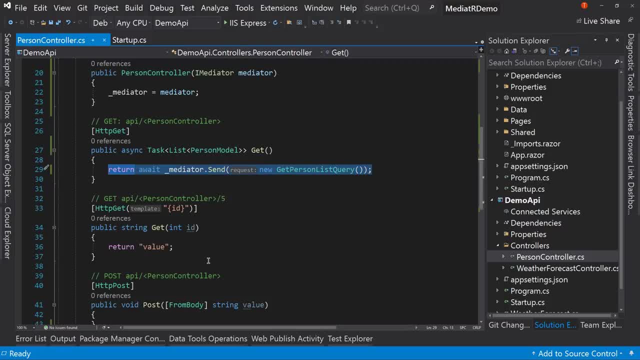 This right here is the definition of practically nothing. It's saying: I don't do anything, I just tell somebody else to do something, That's it. So let's kind of flesh this out: We'll, we'll do it on the API side. 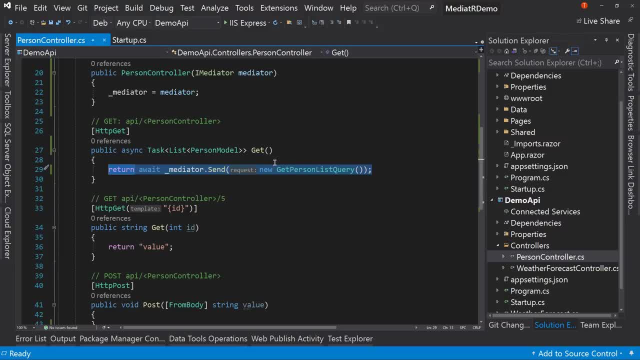 It's a little easier, a little faster than trying to do it on blazer side, Cause I don't want to go into how to create edit forms and all the rest in blazer. Let's just do it right in the API, because it's fairly simple. 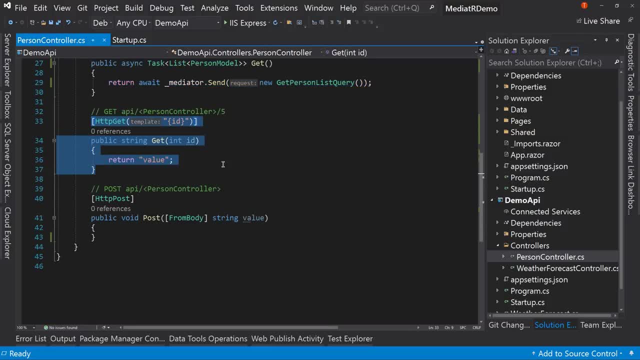 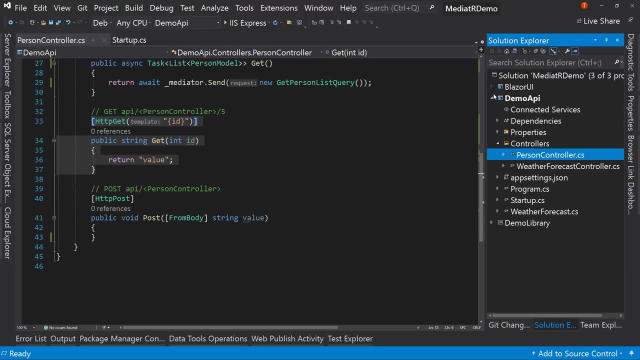 So let's implement this right here, which is just get one, and we'll base it upon the ID. So what do we need for that? Well, let's go back to our, let's go to our demo library. Let's close all tabs. 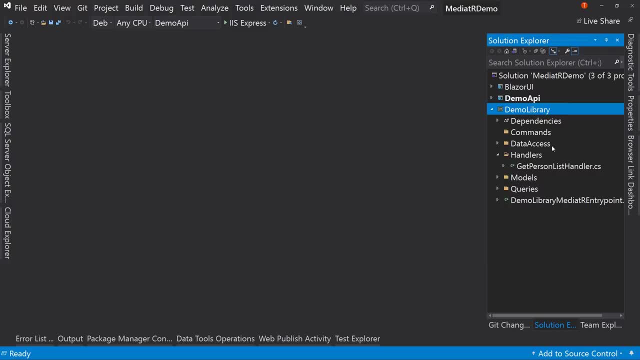 Otherwise it will open back up if I select one of those tabs. So let's go. Let's go to our queries. Is this a query? We're just asking for data. A query should not modify data. Okay, That's the. 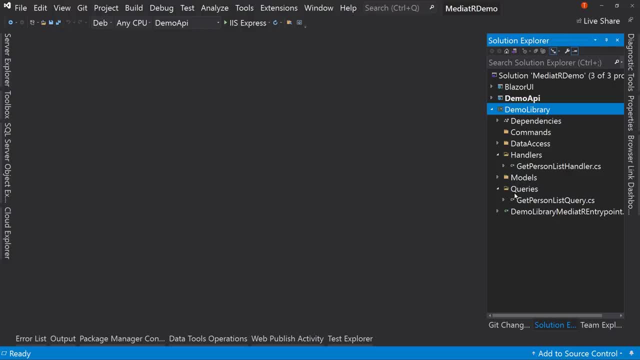 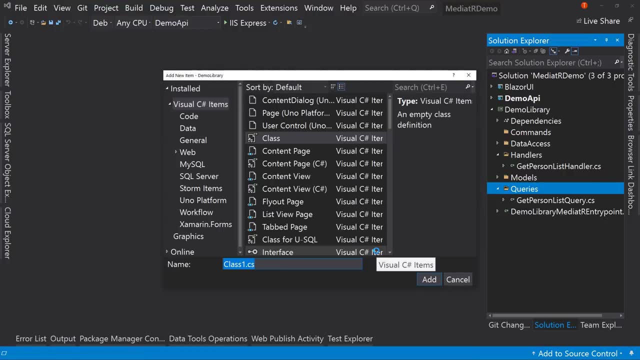 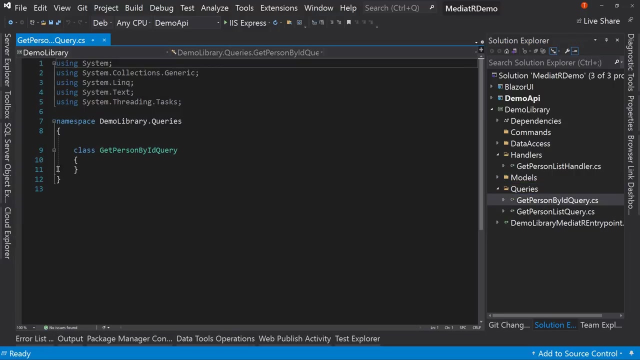 it's a read action, In fact it can be read only. So let's go to queries and we'll say add new class and we'll call this the get person by ID query And again we'll make this into a. I'm going to make this public. 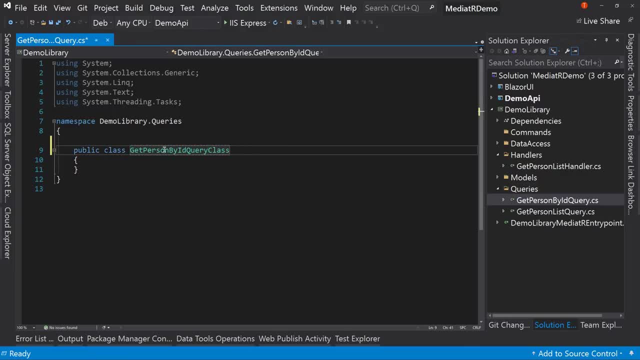 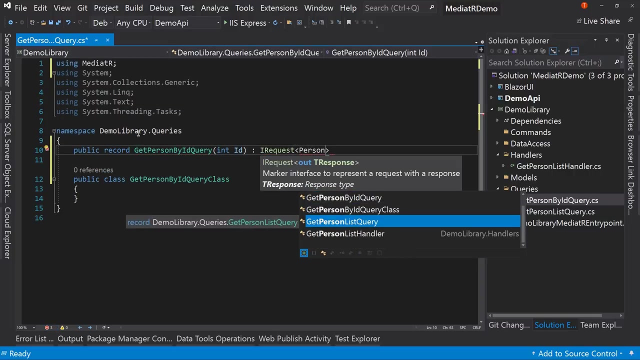 I'll say this will be our demo, just as comparison. but I'm going to do the public record, get person by ID query which takes in an ID and we'll say: I request at the return person model. So that's our entire query, right there. 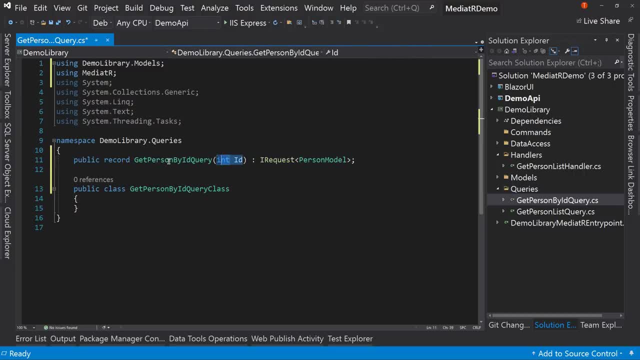 We're just saying the we have an ID in this person by ID query. Now, the class equivalent of this would be to have a property like so and maybe even to create a constructor that required it. So let me say that you know. 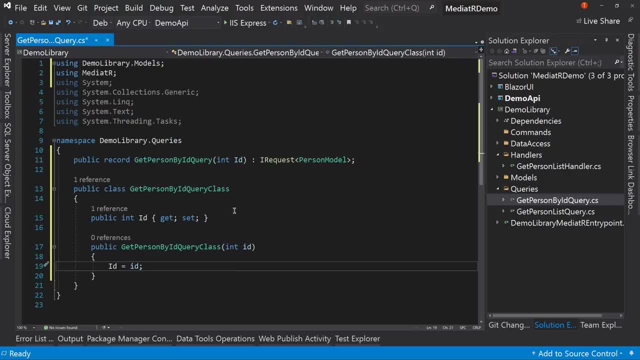 ID equals ID, like so, and then we'd also implement the I request: Okay, So that's the equivalent right there. but why write, you know, whatever the eight lines of code when you can write one really clean one? I'm not big for just shrinking down code to shrink down code. 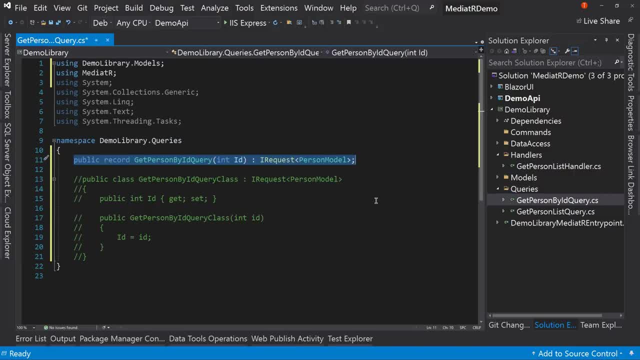 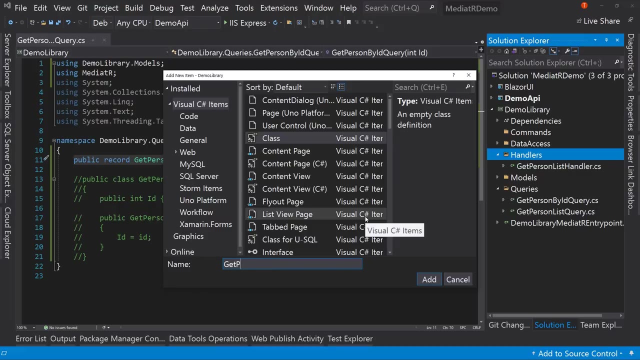 but this right here is just so clean. So there's our record. So we have our query. Now let's create our handler. We right click, we say add class and we're going to say this is the get person by ID handler. 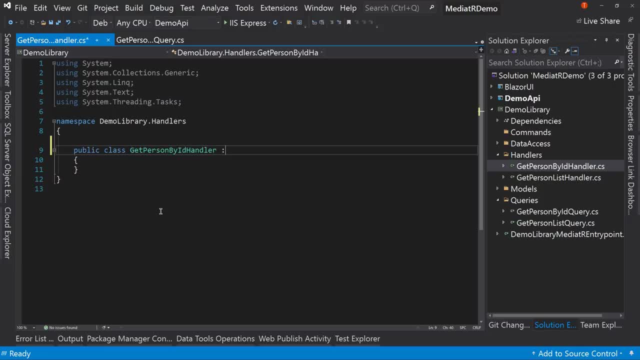 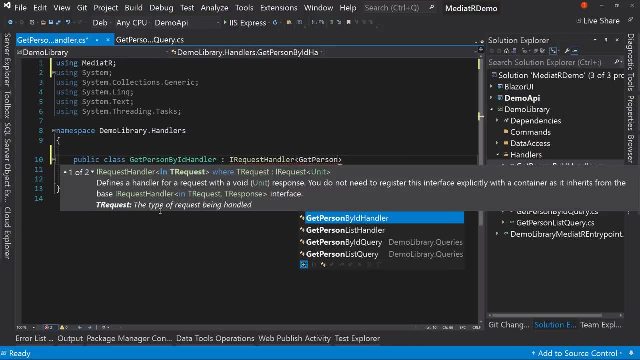 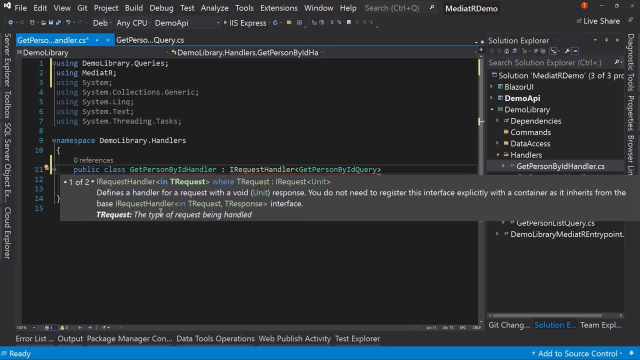 public And this is going to be an I request handler of type get person by ID query. This is where you can get tripped up a little bit. So if I said, um, get person by ID handler, then it's going to let you put that in there. 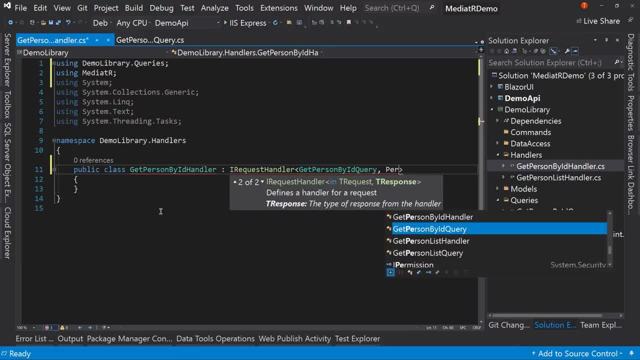 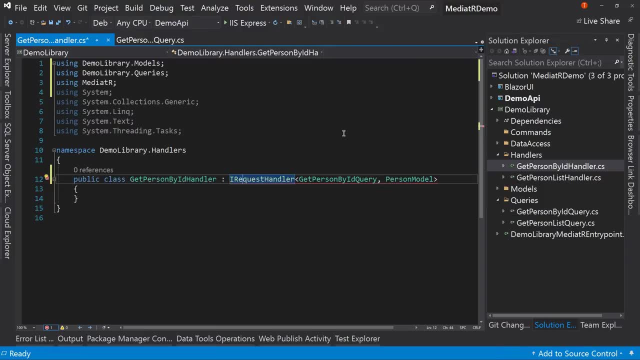 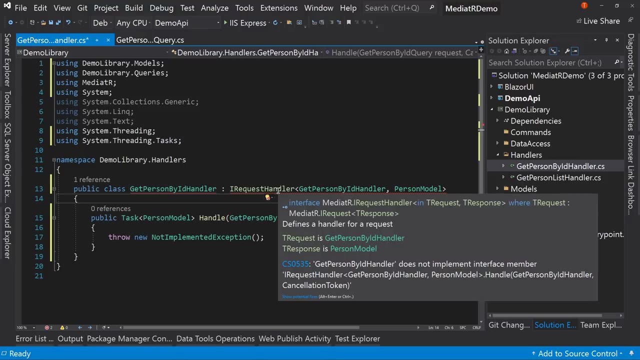 but it's going to yell at me. So, and then person model: All right, And I have to implement this. now control dot to implement the interface. So just to go back to this, if I put this here, instead, it's going to yell at me and say that the get person by ID handler does not implement interface. member. 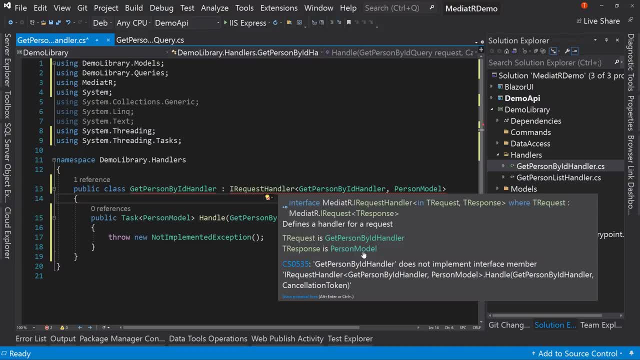 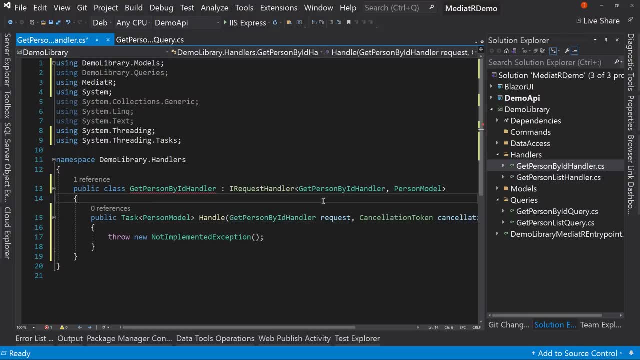 I request handler. You're saying: wait, wait, wait, what? what's going on here? This is kind of a a looping thing. Well, actually, sorry, there you go. That's what it create. But this right here is where it says: cannot be used as a type parameter. 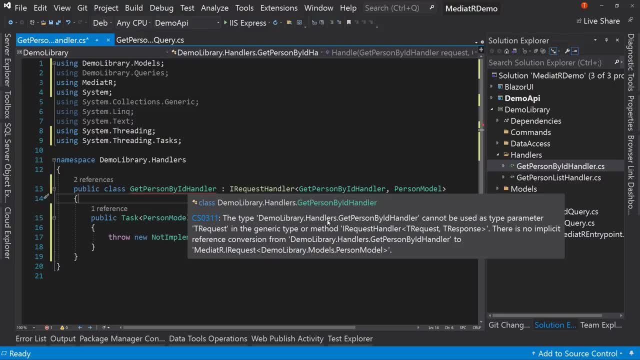 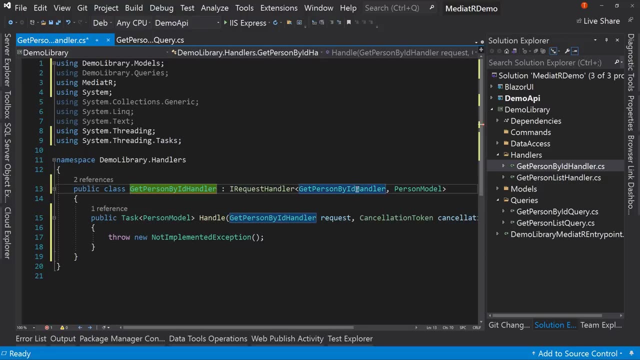 All right, So that's we go. what's going on? Why is it yelling like this? And there is no implicit reference conversion from get person by ID handler to person model, for I request. So that's because we're using handler here. 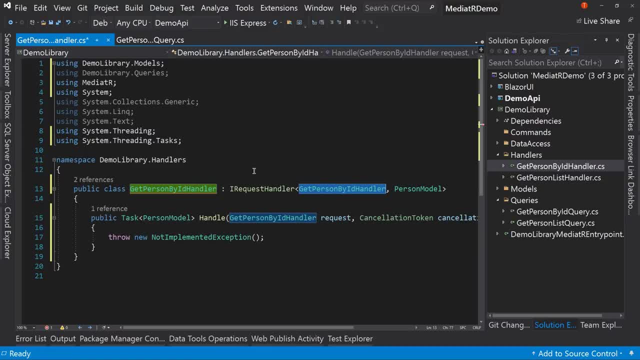 Which is right here. We're trying to implement it and also use it as a parameter. So just note that needs to be a query or a command, So check that. if you have an error, So we'll do the. the undo is here. 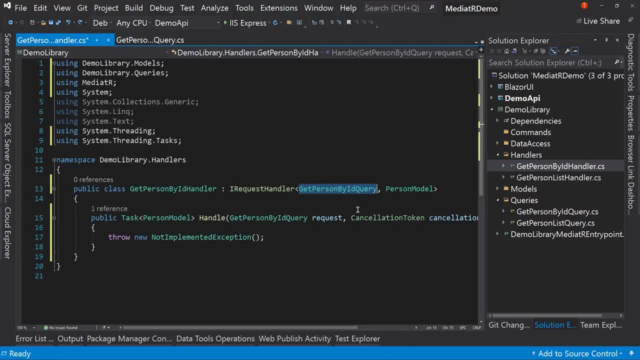 Oops, there we go. So it needed a query or a command in this spot, not a handler. If you have an error, check that first. Now in here I could do a separate call For my data access, except for the fact that my data access doesn't have a lookup. that gives me just an ID. 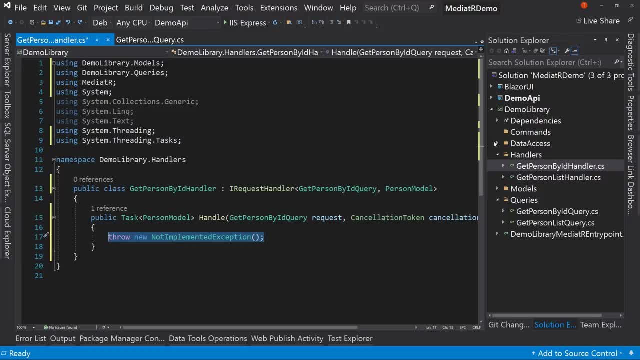 But I do know that I have another mediator object that can give me a whole list And then I can query that list for just one ID. Now, if you have a database and you have a, give me an entire list- and you have another command that's going to give you a record by ID. 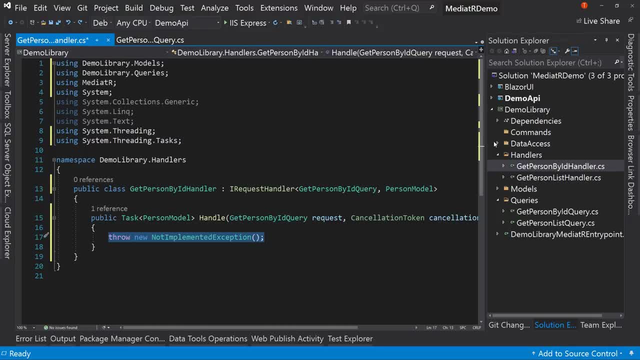 probably you want to go back to the database. The database is more efficient than your, your lookup for everything and then just filtering by one item. But in our case I want to show you the concept of a mediator item, a handler calling another mediator. 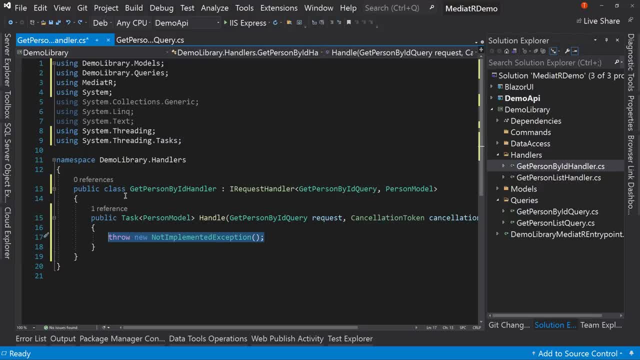 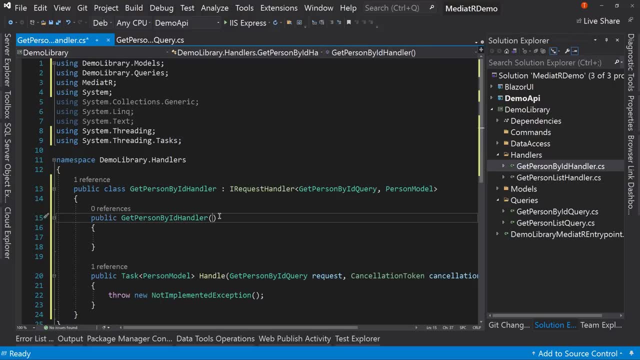 So let's do this. Let's bring in first our mediator, So CTOR constructor, And then in here we'll say: I mediator, which is going to add the using statement, doesn't have it already? I think we already have it for mediator. 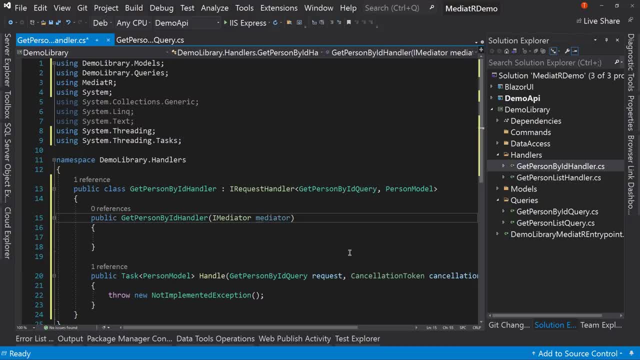 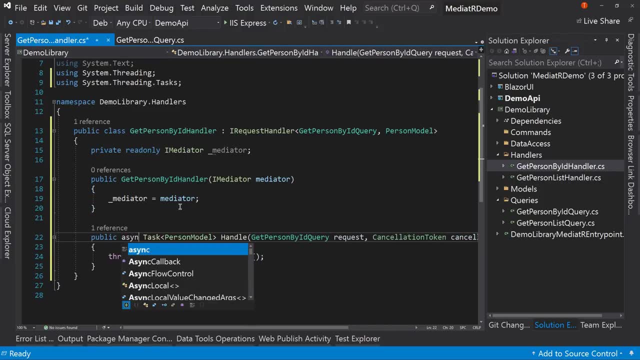 So I mediator- call it mediator- control dot- to create, assign that field. And now down in here let's make this async And we'll say: I want to say var results equal to await underscore. we can type it right: mediator dot. send New. 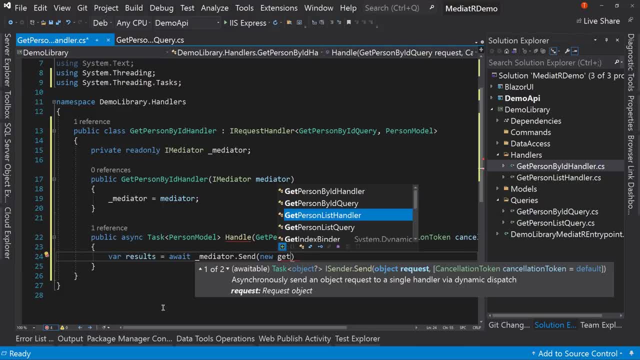 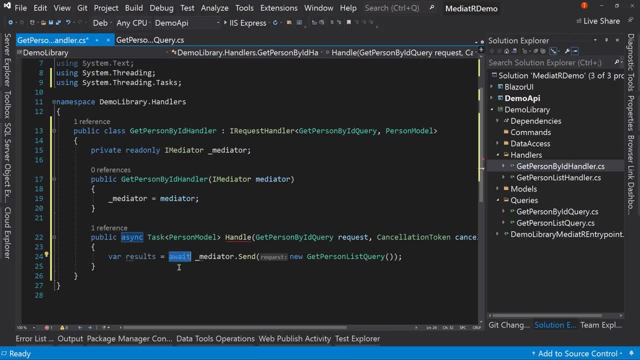 get person list query, So give me all the people that's I want. I'm going to await that, so that the results will be a list of person model And now I can say: var output equals results dot first or default for X arrow X dot ID equals. 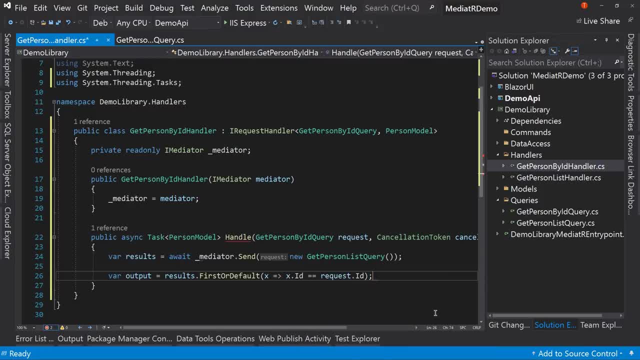 request Now where that request ID come from. that comes from right here where you passed in that data. So you've queried it and said this is the ID I want And I say, okay, find the first or default and the entire list by the first or default. 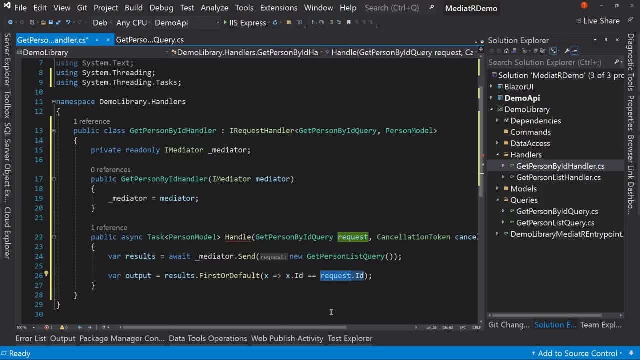 where the ID matches the ID you've passed in. So if you pass in a one or a two, it's going to find the corresponding value, either Tim or Sue. he passed in a three is going to say or default, Which is a null. 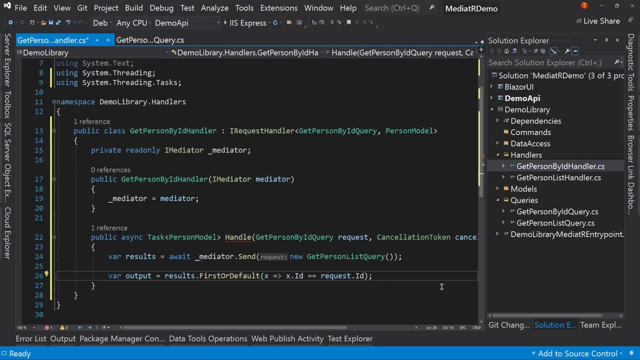 maybe a null in here And then we can say: return output which is the resulting value, either a null or a person model. Now we're not going to get into error handling in this demo Again. we're keeping it really tight to just mediator stuff. 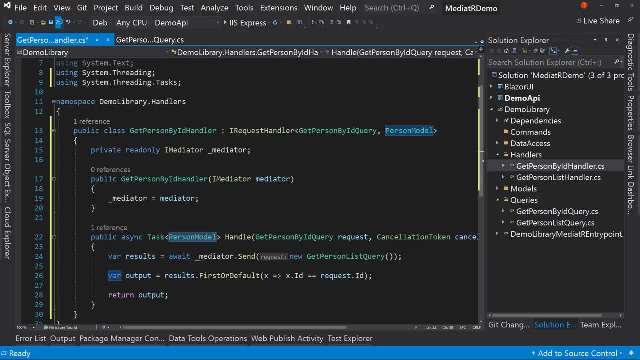 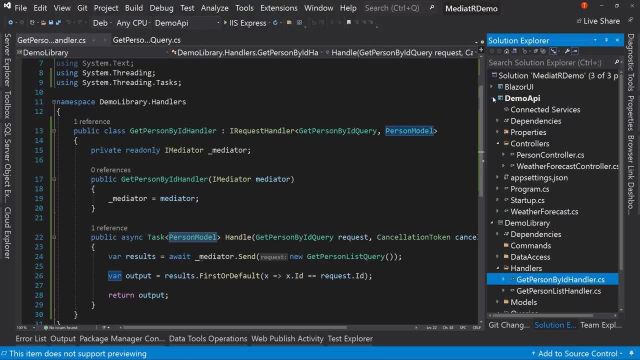 But now I just wrote another handler. This one is going to be for handling, looking up just one, two, one element. Let's go back to our API, changing nothing else. Go person controller. Let's scroll down here to get by ID. 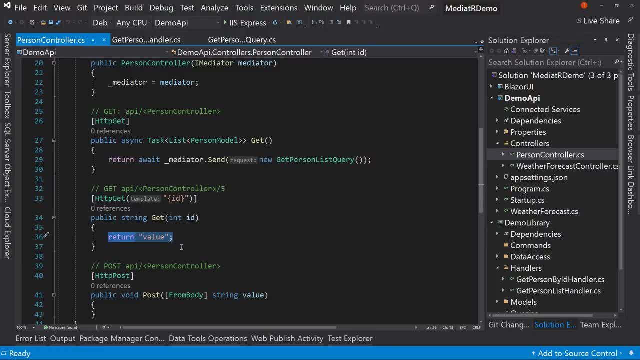 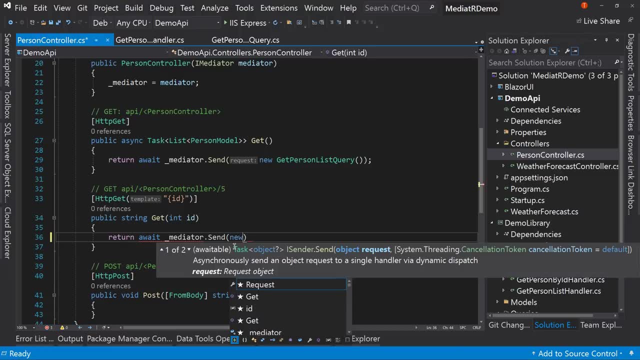 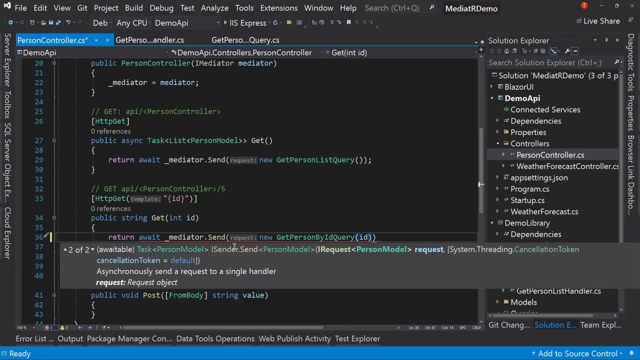 And this is going to look practically the same as line 29.. We're going to return a wait. underscore mediator dot. send new get person by ID query. This time we'll pass in our ID and I'm tempted to put a default value there for some reason. 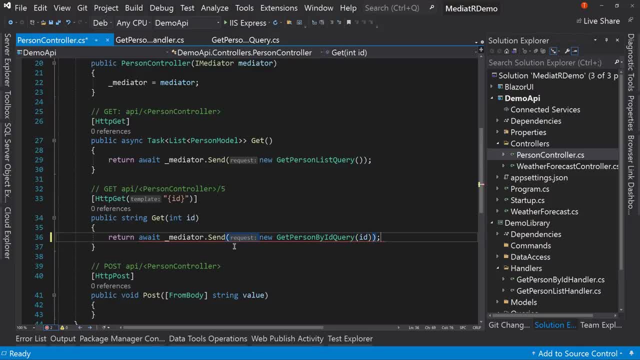 I'm not sure why that's it. So the ID that you pass in for your, your lookup, we're going to pass that into the get person by ID query. We're going to send that out to mediator and say, Hey, give us the handler or call the handler. 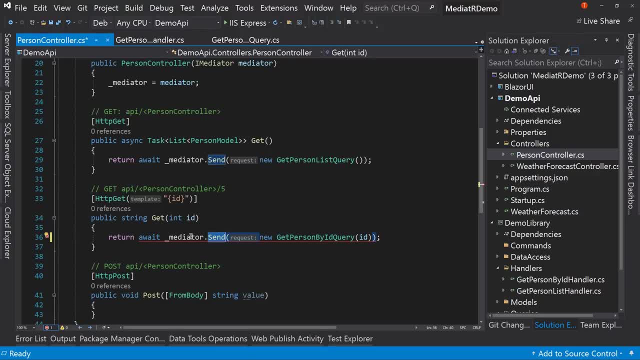 Give us the results The handler gets and return that We're going to wait for that. Now it's yelling at me because this should be not string, It should be a sync sync task of type person model. That's our, our lookup. 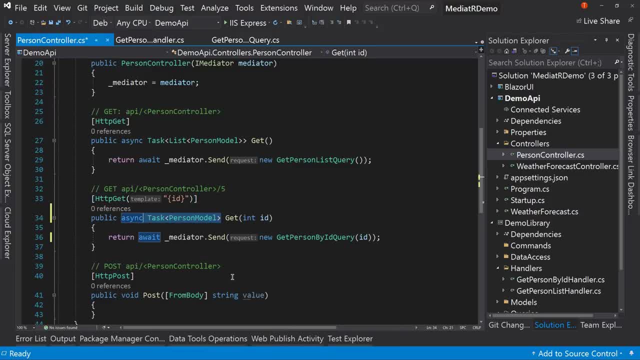 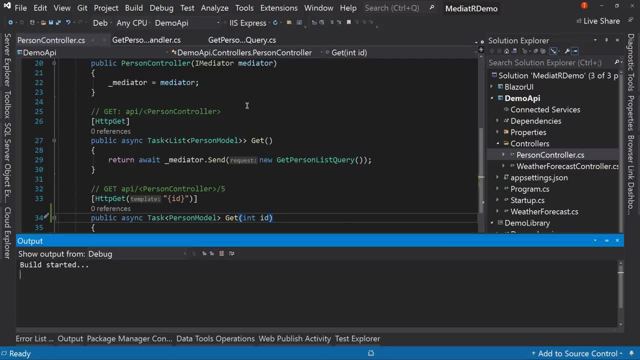 All right, So that's what's going to turn as a task of person model. We're going to wait that. So now, with this in place, we can run this again, and this time we'll be able to do a lookup based upon our 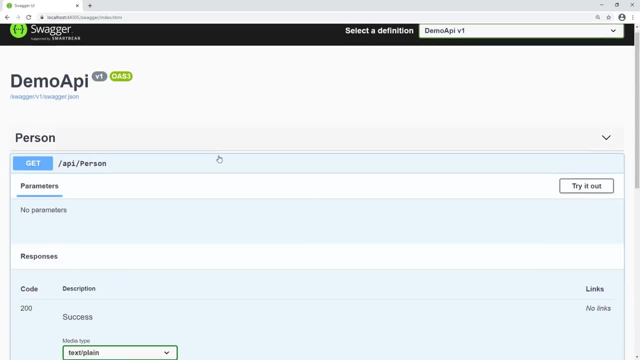 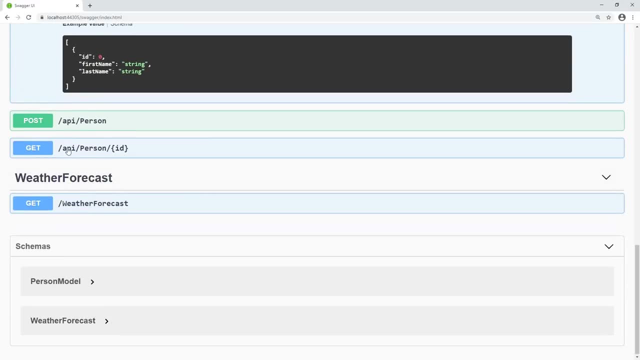 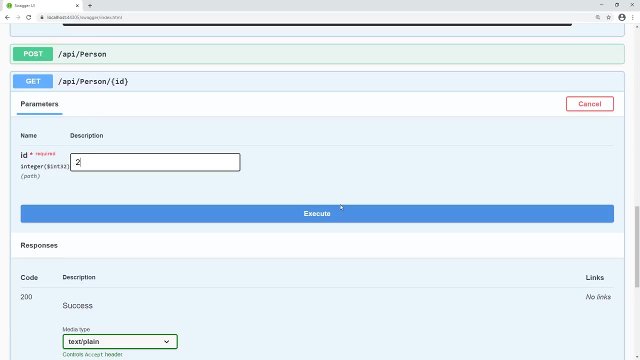 ID. So we have the person, we can do the tried out execute and we get the two results to him in suit. Then down here we have get person by ID. We can say try it out. We change this to be to execute. 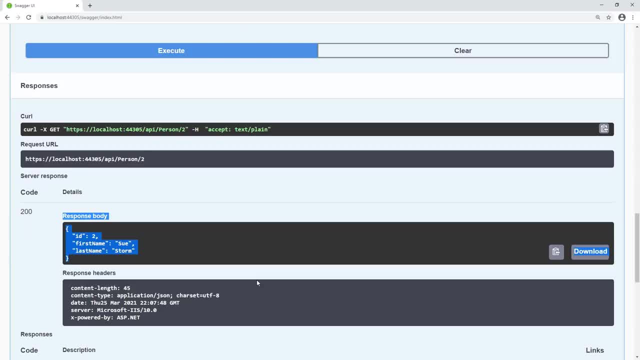 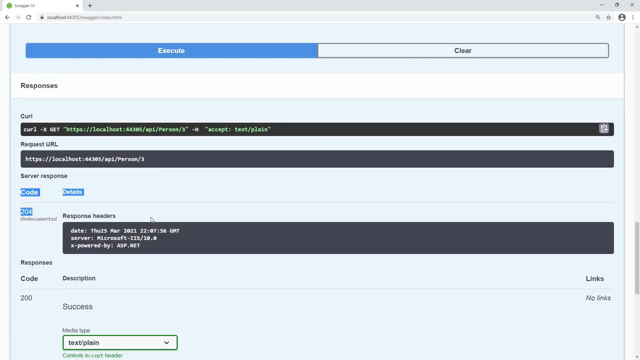 And the result is we get back Sue storm. Now, if we say three here and execute, we'll get back a two, Oh, four, basically a um, a null, Okay, So we haven't gotten any, any data back for that. 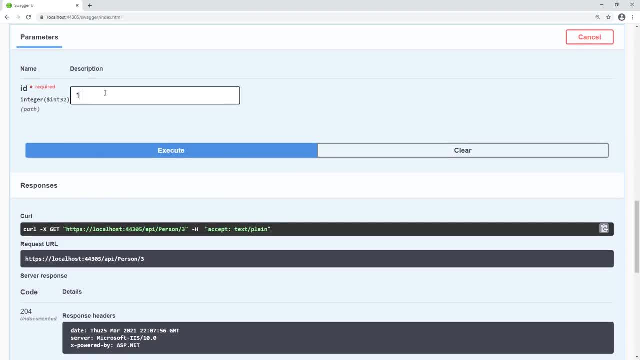 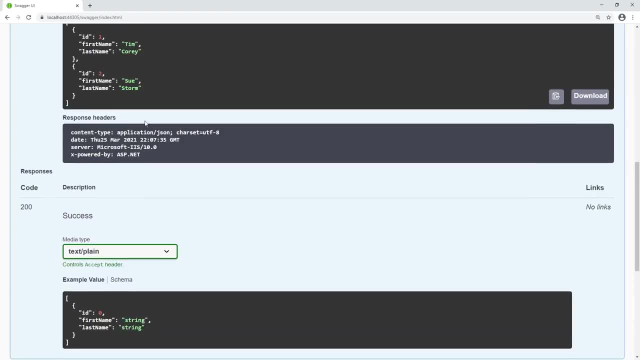 We could have handled that. We're not going to um pass into one here and get back Tim court, Okay, So now we've got these two wired up. We've got the get person and the get person by ID. ignore where their forecast. 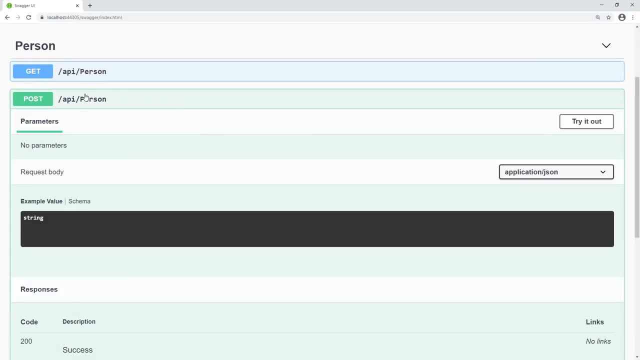 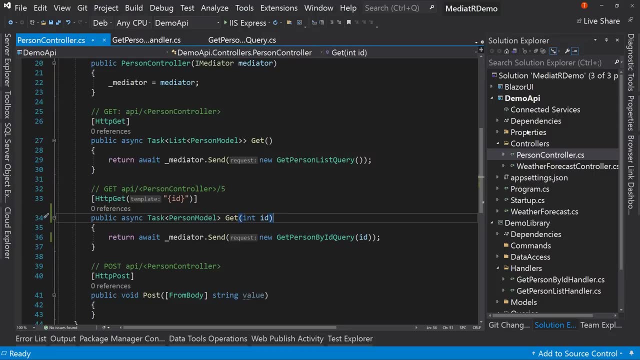 Um, let's do the post Now. let's set this up so we can send in data. So let's close this out, Let's go back to our demo library. but we're not. we're not going to create a query because, remember, a query is for reads. 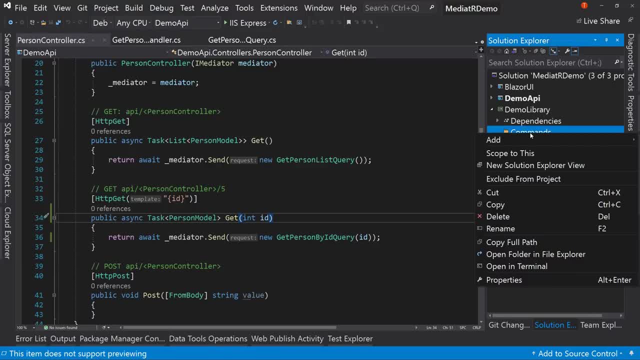 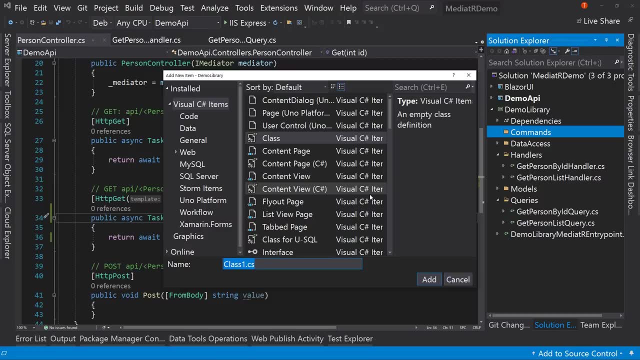 We want to create a command, So right click add. This is going to do an insert into our database, which in this case is just a, a static list. So let's call this insert person command, which I'm going to create, that again. 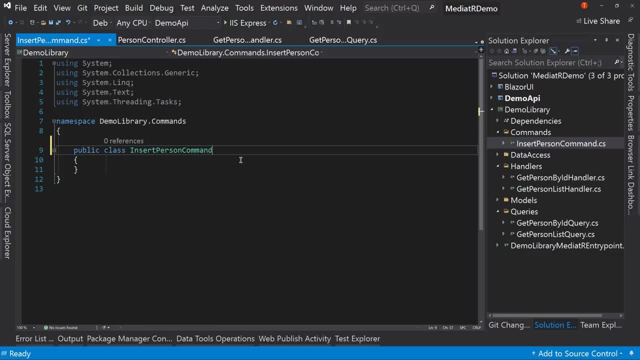 that demo for you. Uh, public class with class at the end, And we're going to say that we have a string first name, string last name, and we'll create a constructor as well. Um that we pass in those values. 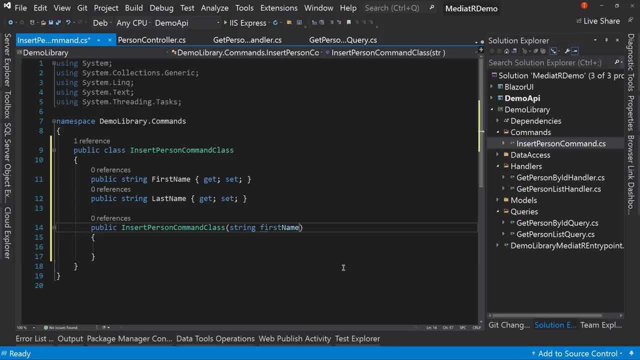 So string first name, string last name and then say that first name equals first name and last name equals last name. Okay, That's essentially what we're going to do: and implement the I request and it's going to return back a person model. 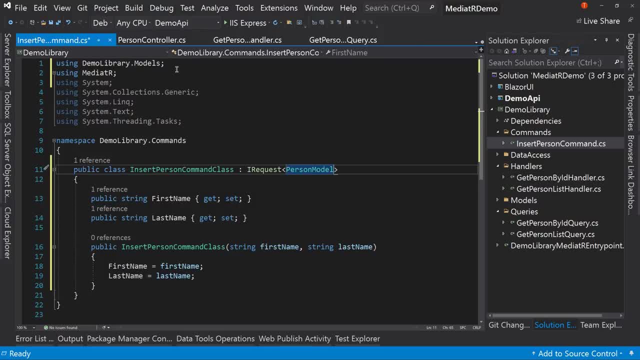 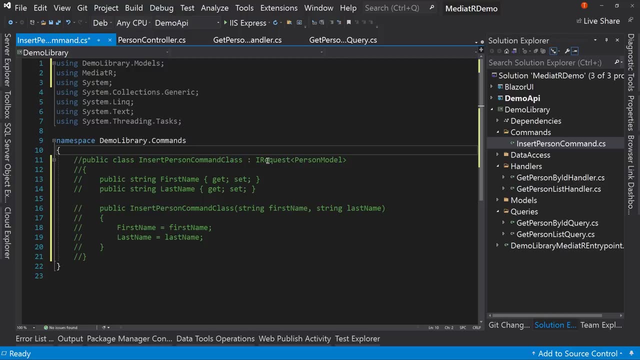 Okay, So I add a using statement for that as well. So there's a two usings that have been added. So that's that's the code we could create If we create a class. but let's comment this out. We do want to comment it out, because we would otherwise have another. 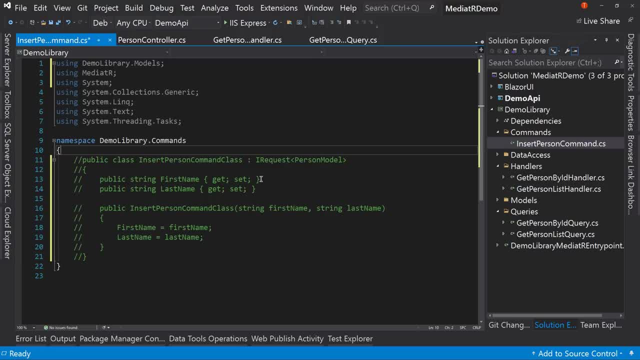 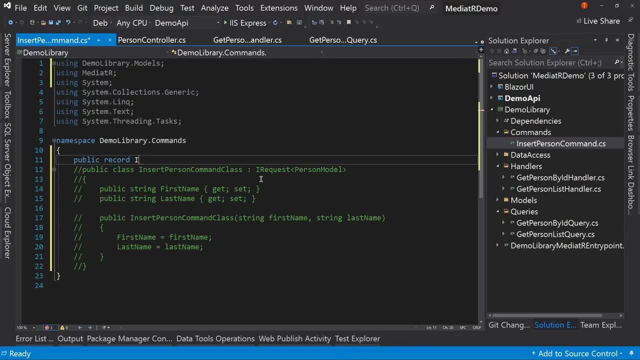 uh command, but this time it would be have no handler. So you do want to comment that public record insert person command that takes in a string first name, string last name. And if you're not familiar with, let's do I. 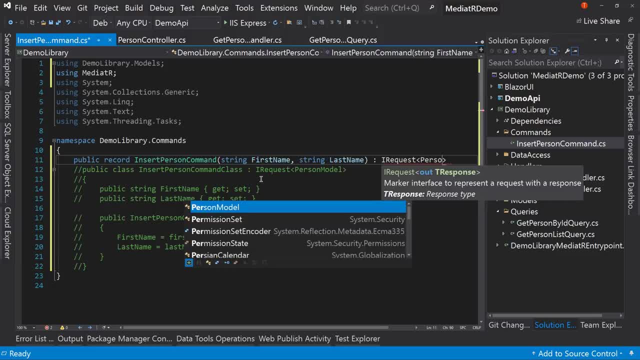 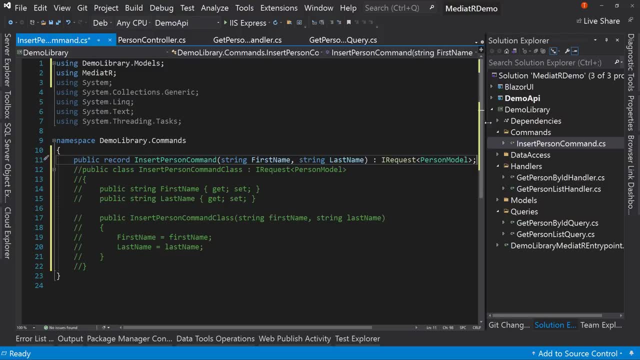 let's do. let's do this first. I request person model and notice how it's in a semi-colon Notice, how it even kind of reads like a um a command, where it says: okay, here's the command. I request a person model. 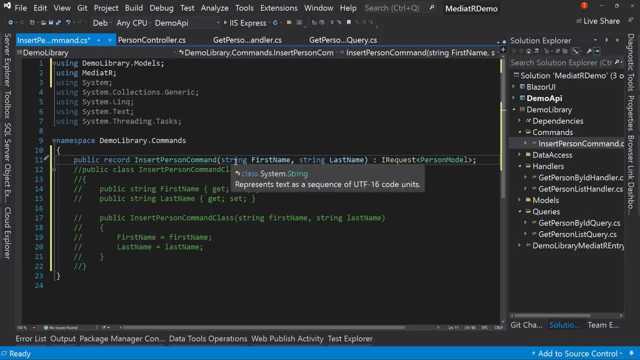 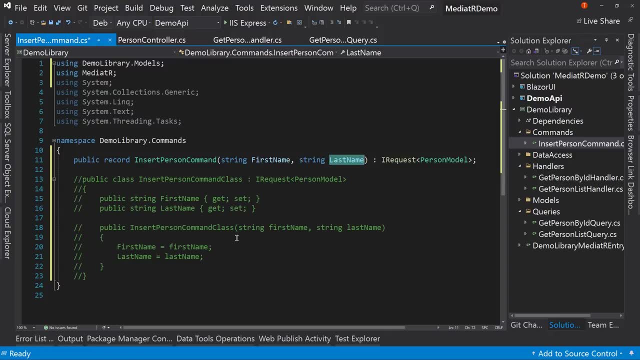 That's why I want to return. So if you're not familiar with records, the the fact that we are capitalizing first name and last name may seem a bit odd, because down here we have a lowercase first name and last name, because that's what a parameter typically is. 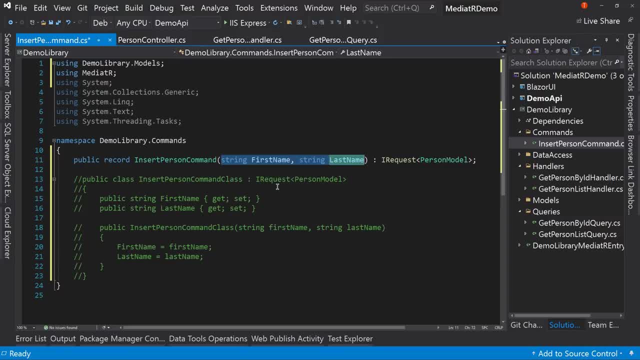 These aren't traditional parameters. They're actually going to create properties based upon these names. So therefore we capitalize them because the properties should be a Pascal case, not a camel case. So again, watch my records video if you want more in depth on that. 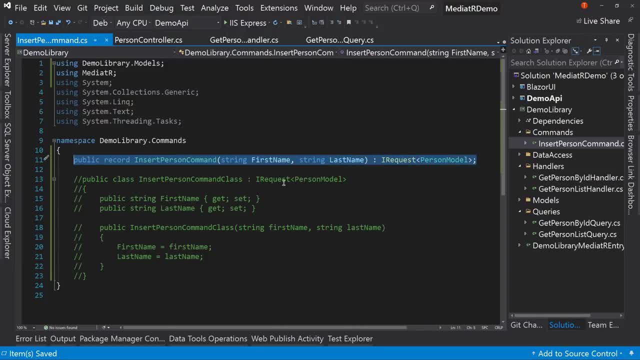 So again, that one line is our command. So we're going to pass in a first name and last name. We're gonna get back a whole person model. that want to get that whole personal model back. So I can see, see what was inserted in the database. 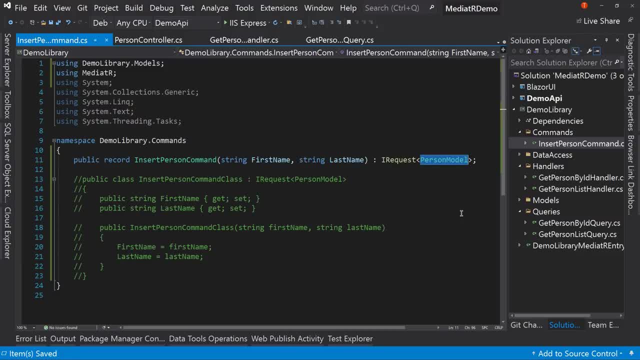 including the new ID. So let's talk about creating a handler for it. Now handlers are all going to same spot, So whether they're commands or whether they're queries, they all have this one handler spot. So we add a class for handler and let's call this handler. 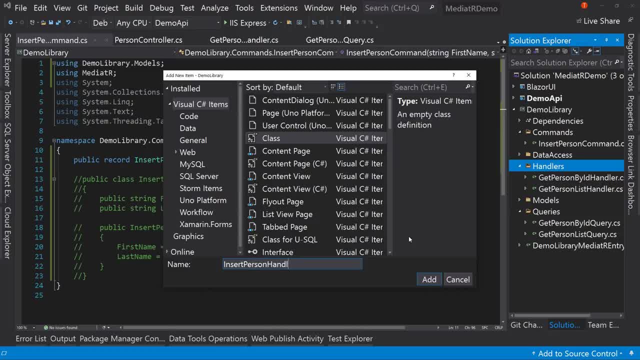 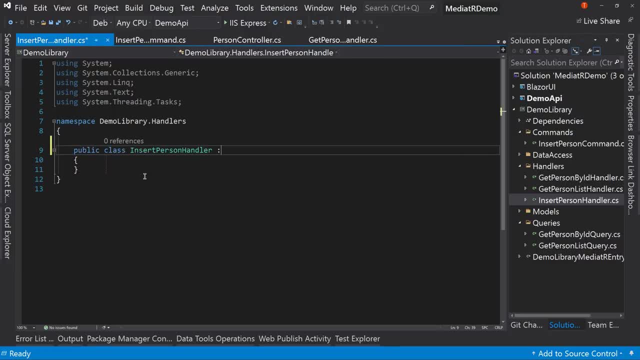 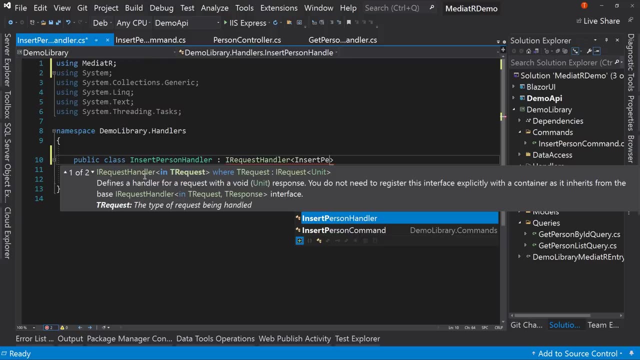 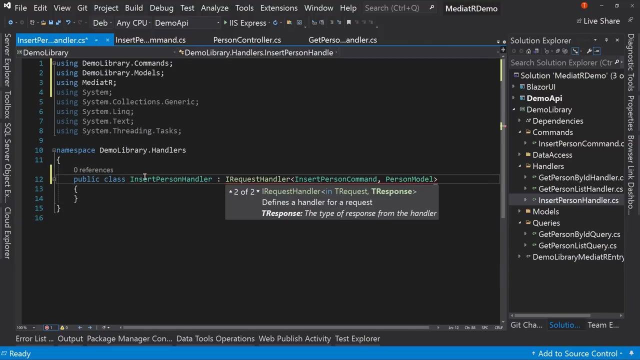 the insert person handler and I'll make this public And at the end this will say: I request handler insert person command and the return is going to be person model and again it's adding using statements for both of those. 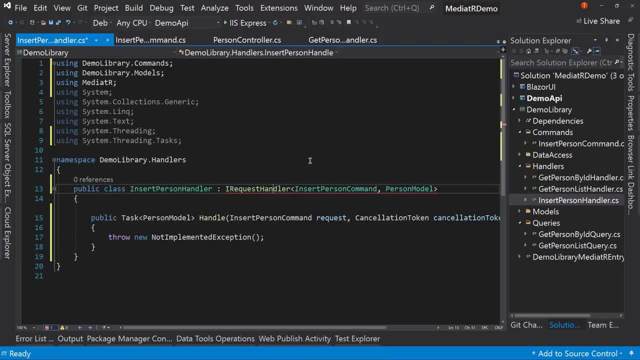 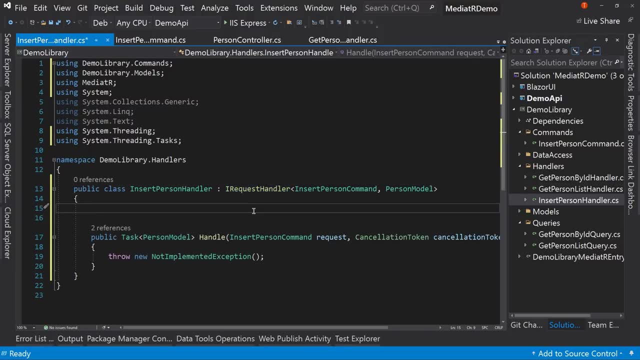 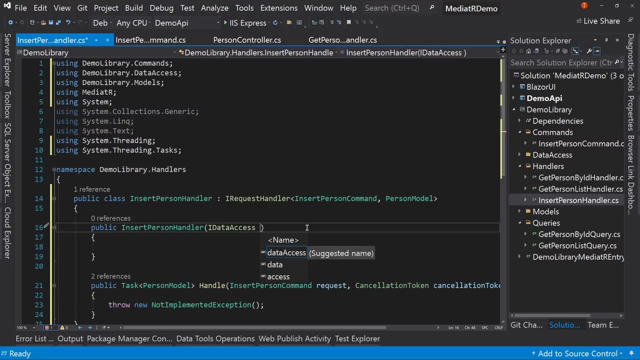 Now we can do the control dot to implement that interface And we do have to bring in data access here because we are going to be calling that directly. So C T O R, where we ask for the IDataAccess, call it data control dot to create and assign that field. 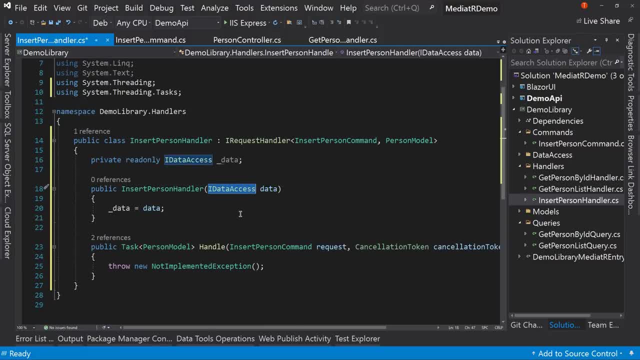 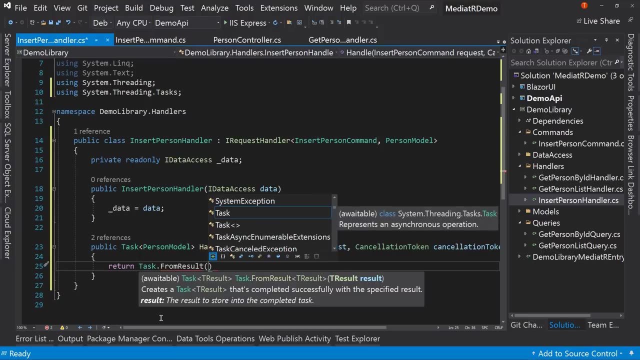 And now we've talked to our dependency injection, got our data access and down here we can do our code to call data access, which is pretty simple. We're gonna return taskfromResult- Again, that's kind of that cheat. We're gonna say data dot insertPerson. 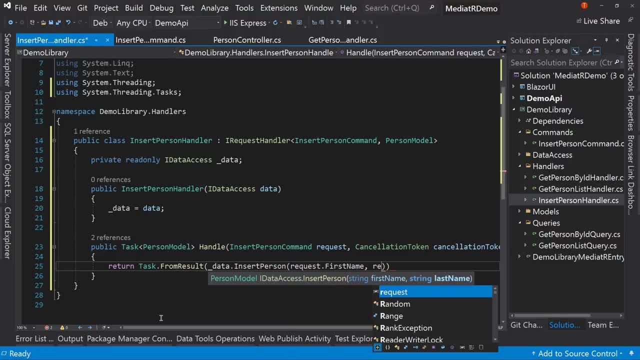 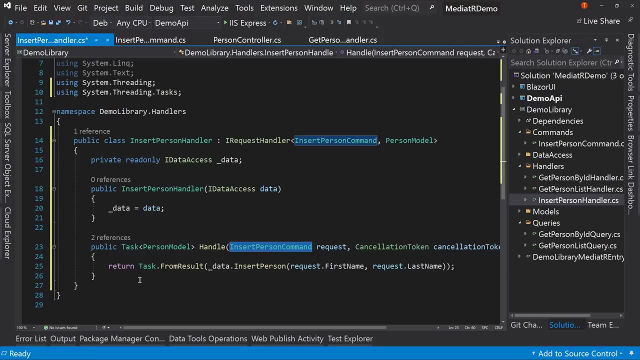 request dot firstName. request dot lastName. So I'm doing insertPerson, I'm pulling the first name and last name from that command because that command has those two values. That's it right, Because I'm returning that, because insertPerson returns the full person model. 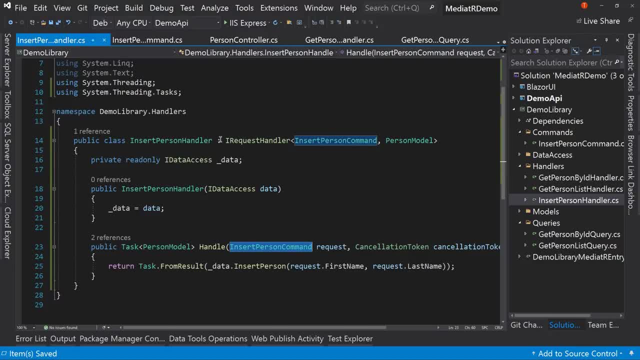 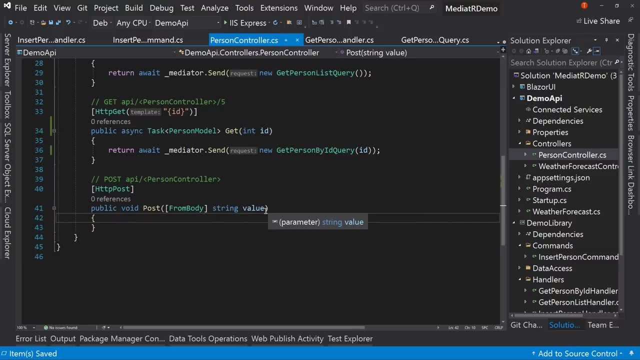 Handler is done. So let's go back over to our controller, Our controller. we have this post here, which right now we're from by we're getting the string value. Let's just get the, for simplicity sake. we'll say person model and we'll say value. 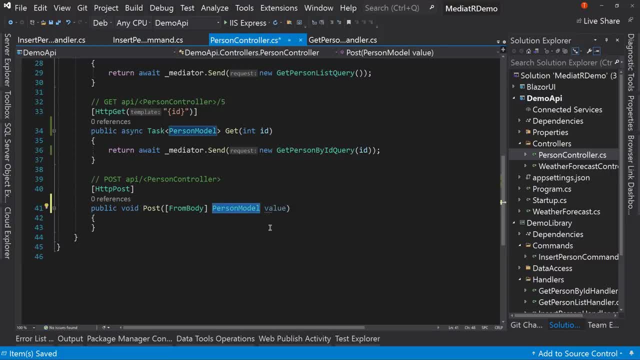 So yes, you probably have a separate model for this that had just the first name and last name, not the ID as well. We'll just leave the ID blank and we'll say: var model equals new insertPerson command where we pass in value dot firstName. 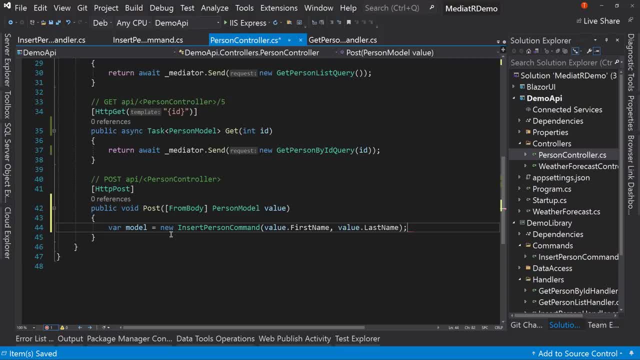 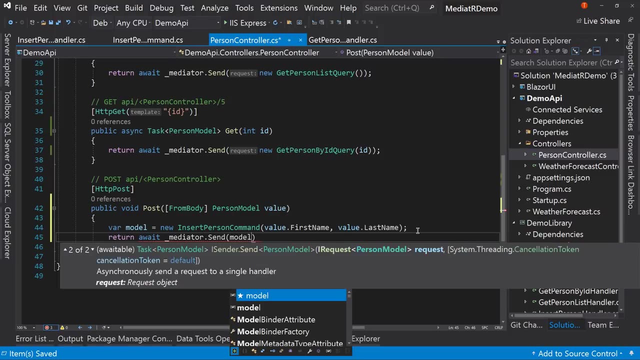 and value dot lastName. So those two values are gonna pass into our model. That's our insertPerson command. Now we can say return await mediator dot. send our model, Because our model is that insertPerson command. I just didn't One line do it. 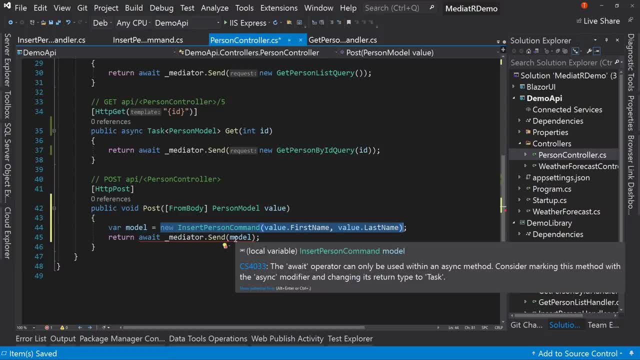 I could have said this right here, put that in our send and do it in one line, You know. so let's just I'll show you. I copy this, I paste it in here, I can comment that out, and now it's in one line. 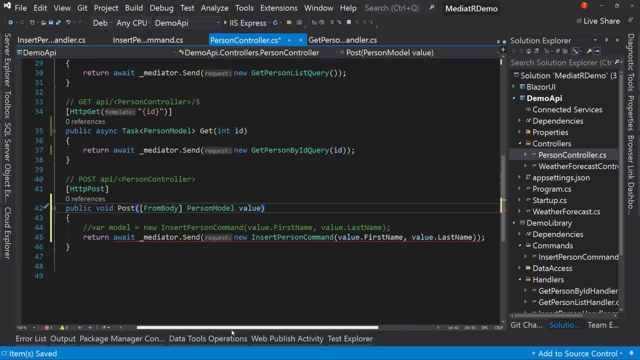 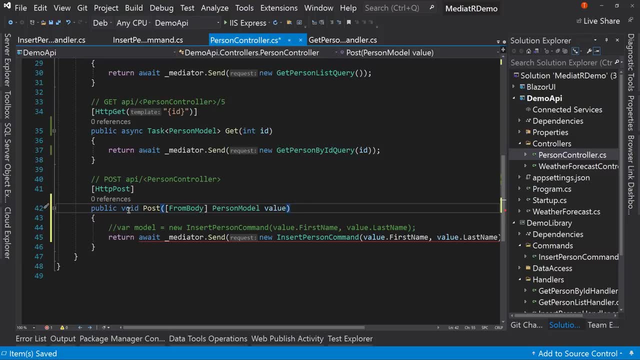 And yeah, it's yelling me. Why is it yelling me? Probably put an extra semicolon or something. Oh no, it's yelling me because I have a return await, which this is a void. So task of type person model, there we go. 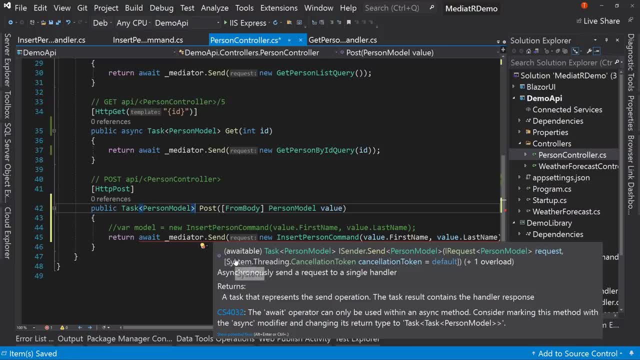 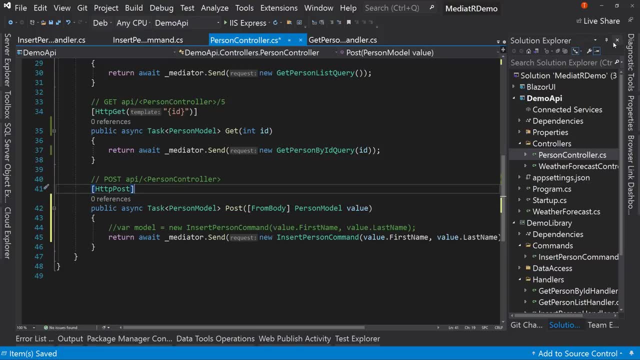 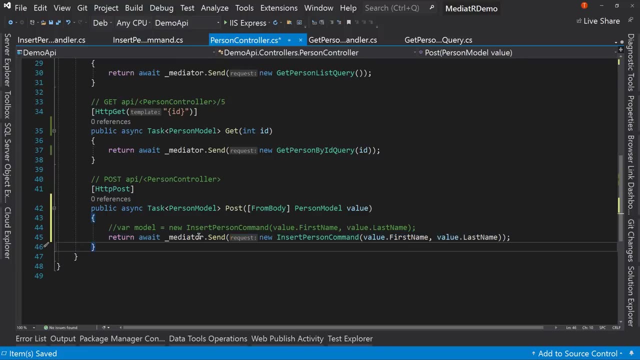 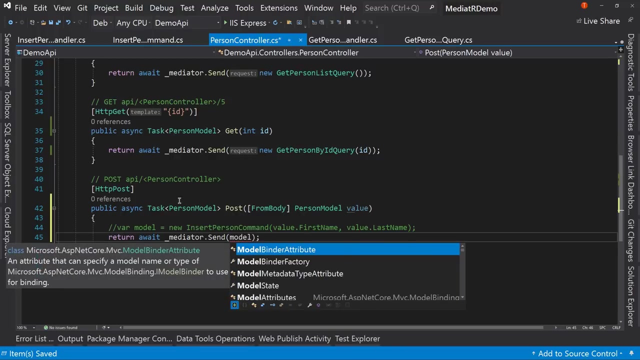 That should, oh, async task of type person model. There we go. So we have either one liner value, which can get you know a little bit long, or you could replace the send value right here with model And then do it in two lines. 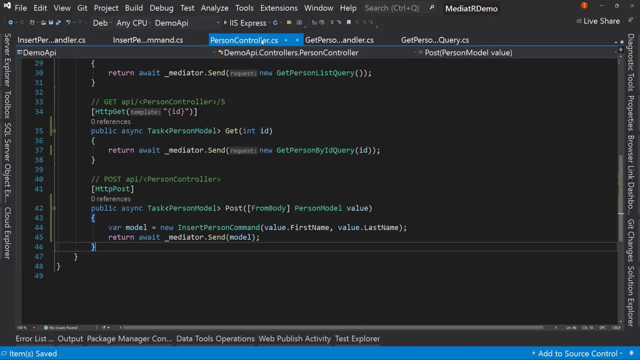 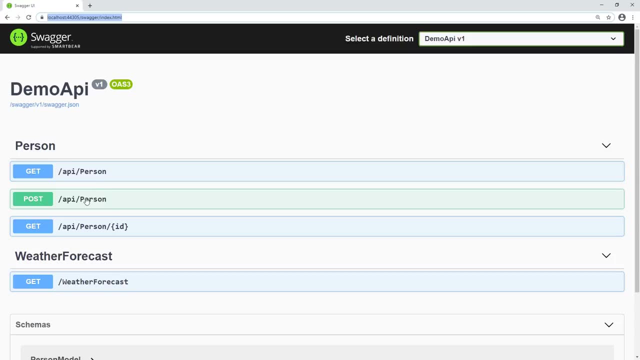 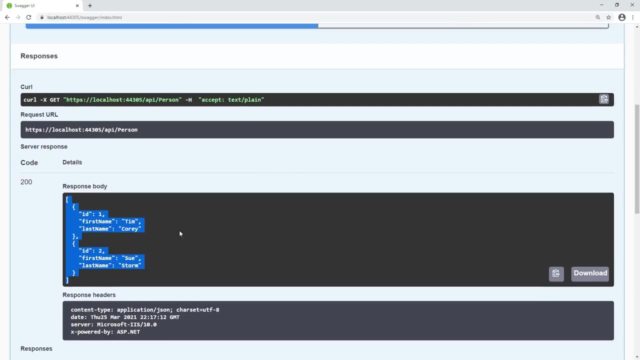 It's up to you. But with that we run this one more time And now we have our let's just get the list people. So you have it, try it out, execute, And we have our short off one and two: Tim and Sue. 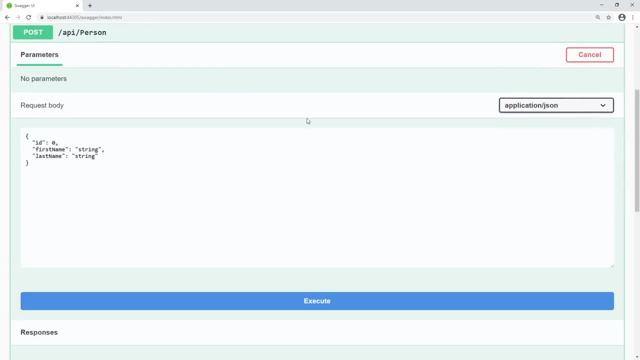 Go to post, try it out And we have this little JSON byte. Again, ID is there, but we can ignore it, leave it alone And let's just say Bob Smith execute. The result is ID of three, Bob Smith. 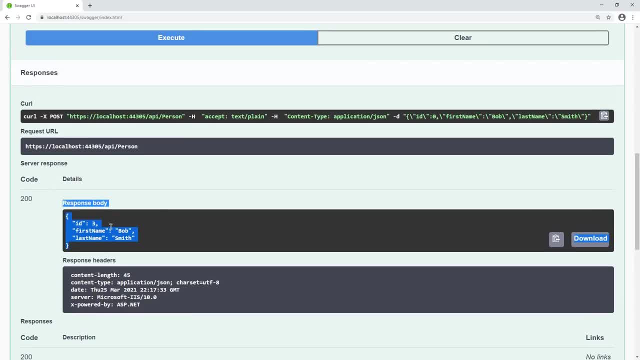 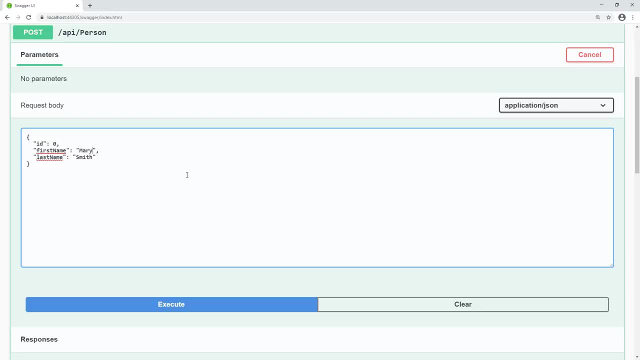 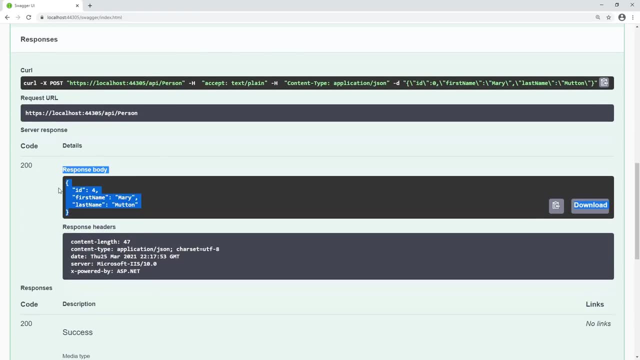 That's what was returned, because that's what we inserted was Bob Smith. The ID that got generated was three. Now if we said marry mutton and execute ID is four and marry mutton, Let's go back up to the get person, get the whole list. 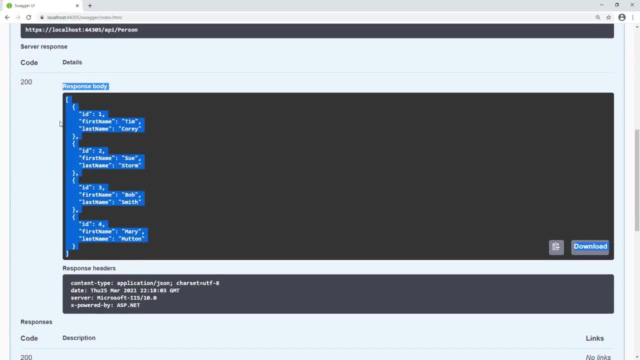 execute this. You'll see. now we have four entries in our quote unquote database. We have Tim, Sue, Bob and Mary, And that's because we're using that singleton to kind of game the system into remembering, between calls, all the data that we've changed. 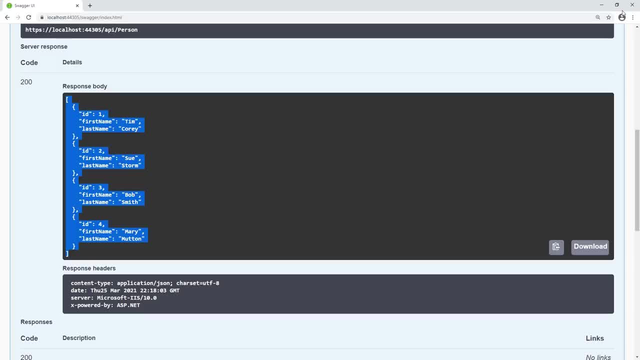 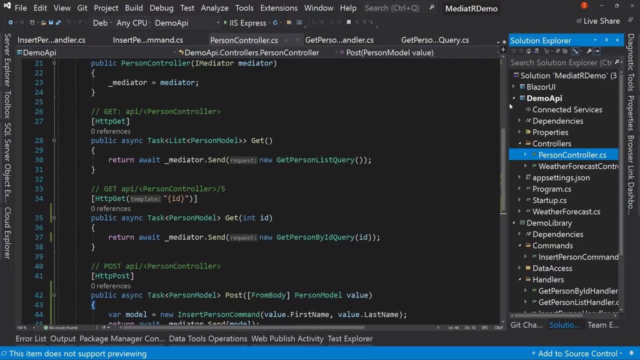 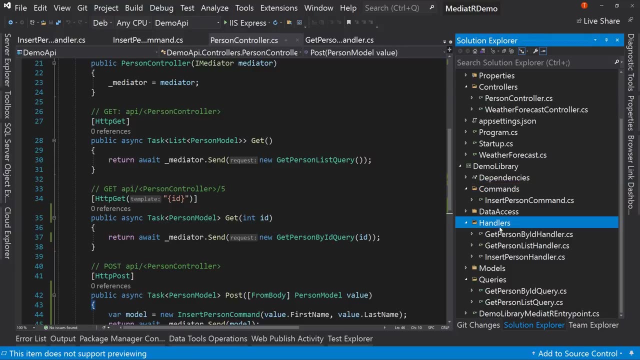 And that's using mediator. So let's kind of go over what we've seen here. The kind of broad picture context here is that in mediator itself, the tool, we have the concepts of commands, handlers and queries. Now we haven't talked about that kind of the more. 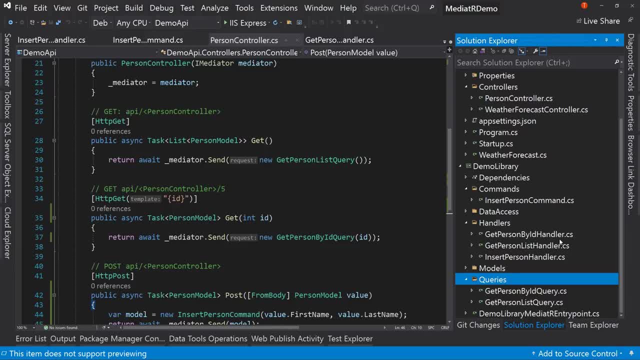 of the eventing style of system. We'll probably cover that in another video. But for this pattern that we're using the CQRS, we have our commands, handlers and queries. A query is just the data that you're sending in. 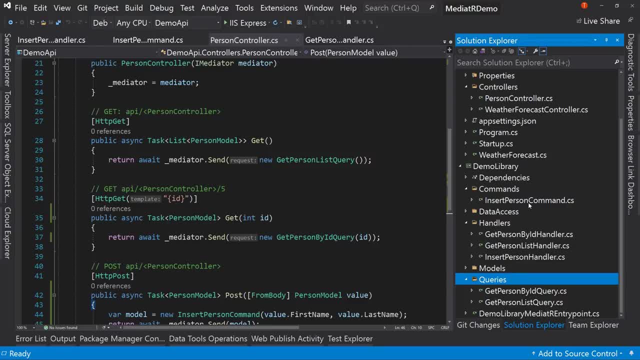 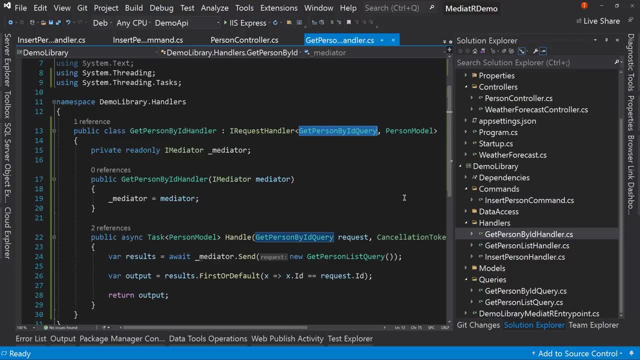 And the same with the command. It's just the data you're sending in And the handler says: I'll handle one of those queries And this one is handling the get person by ID query, And so it does one job: It handles one query or one command. 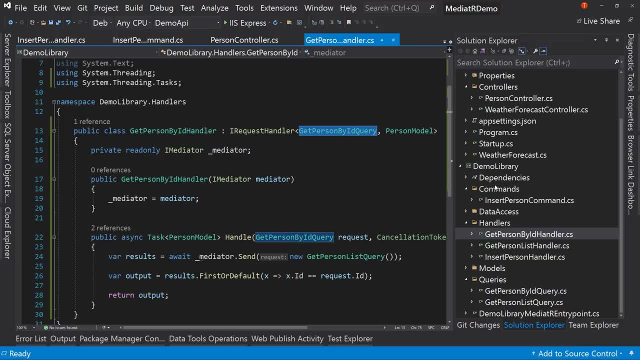 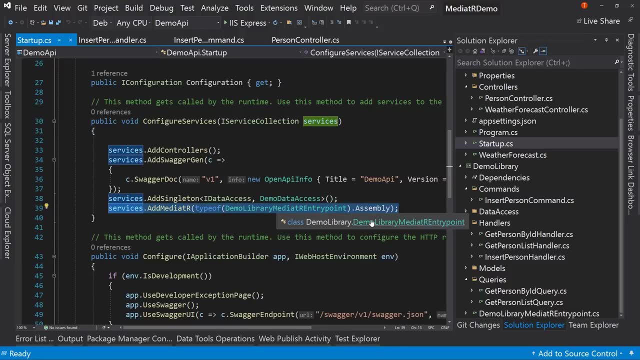 That's all there is to mediator, because then mediator will scan your system, Your assembly, for all of the entries that say I request handler or I request Now. scan all of those and put them into the registration system. And it happens once at the beginning. 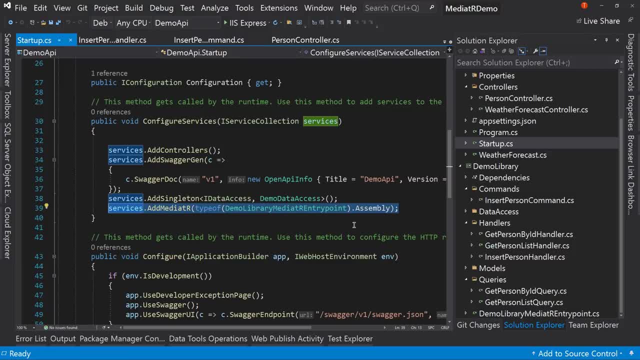 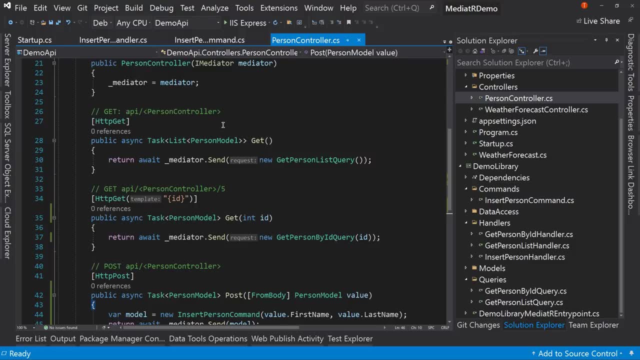 It's very quick And then from then on, whenever you want to make a call, instead of asking for all these different dependencies you might need, you have just one dependency. It's on imediator, And then from there you just say send. 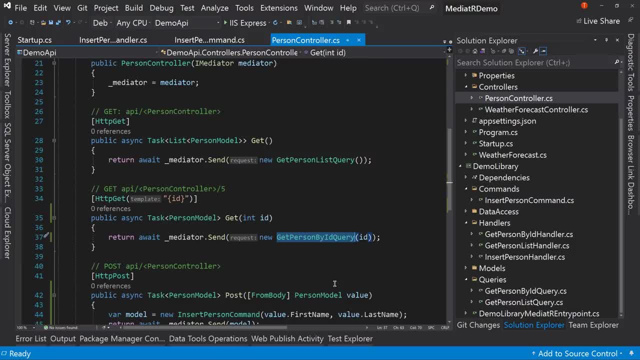 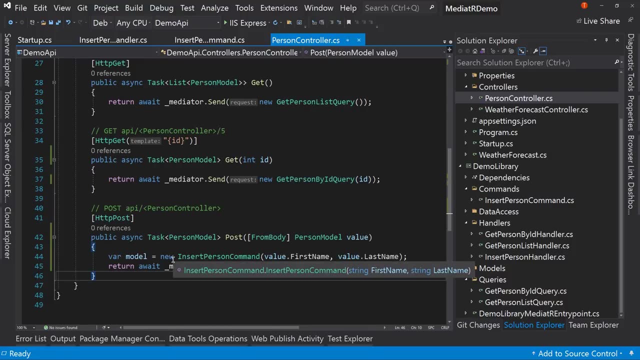 and give it which query or command you want, That gets executed and your data gets returned. So, if you notice, I have a fairly complete API controller right here And yet really the actual lines of code for calling all the database and getting the data. 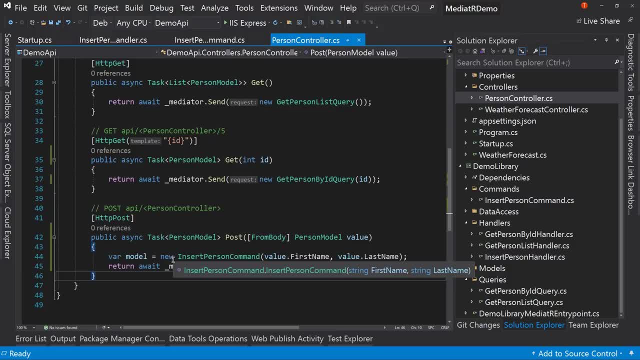 searching through it for the ID lookup and returning the data, Returning back the values after creating a new ID, and all that kind of stuff. All that work is in this line, this line And, in this case, these two lines, because I didn't want to make it into a one liner. 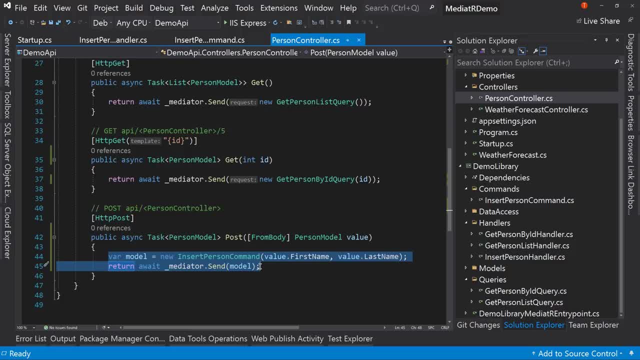 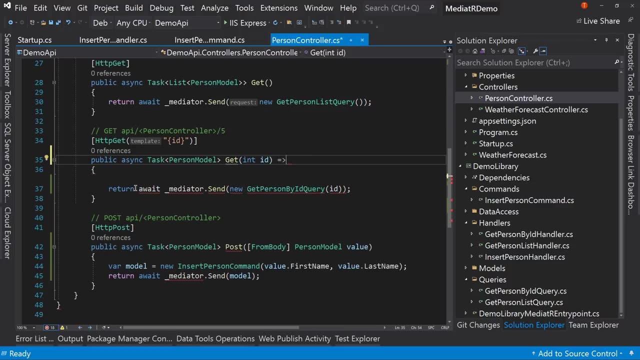 That's it. So our controller is tiny. It's very, very small. In fact, this can be shrunk down even further into an arrow function, something like this, where we say, oh, I'm gonna do this, And then just have our, our weight, like so. 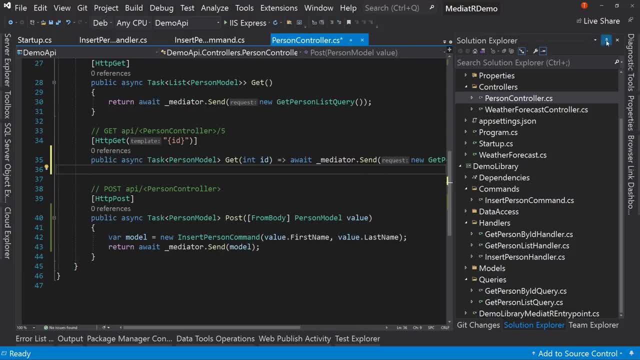 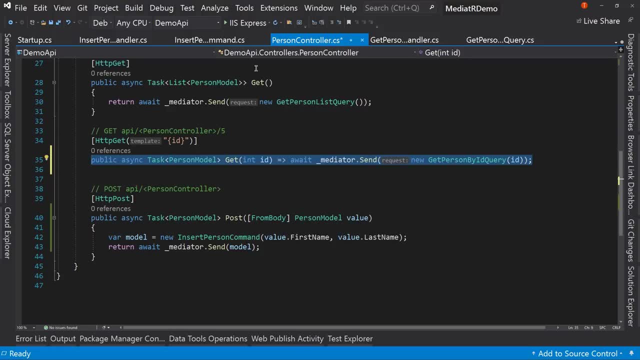 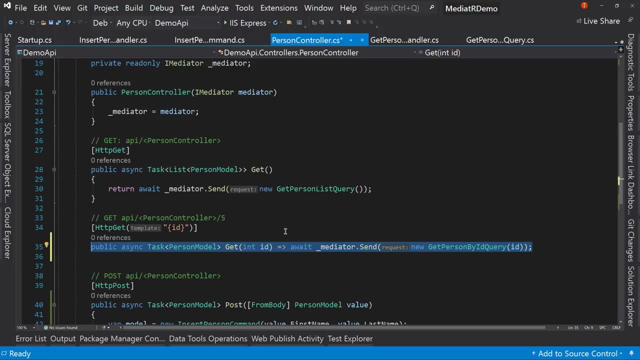 And that'd be it. Okay, So that could be one endpoint, The insert or get by ID. We have a same thing for all of these, where it is one line, one line, one line for each of our, our gets posts, puts, deletes, patches. 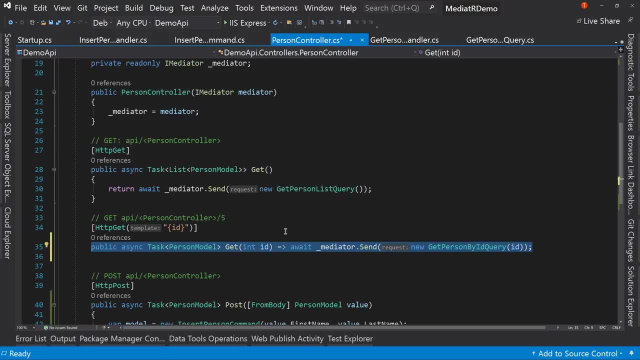 All of those things Can be done with one line, because the work is not being done in the controller. This means the controller, in a lot of ways, doesn't need to be even tested, And you can argue with that if you want. But what happens instead is you can test those handlers. 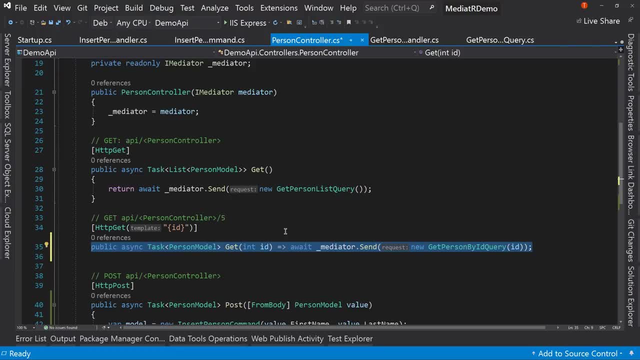 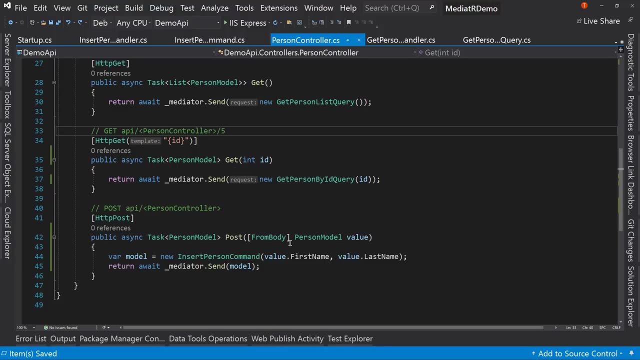 That's where the actual work is being done, So I'll undo that Just doesn't confuse you. Actually, I don't know how far it went, So let's there we go. So that's all you need to do in order to keep your controllers very tiny. 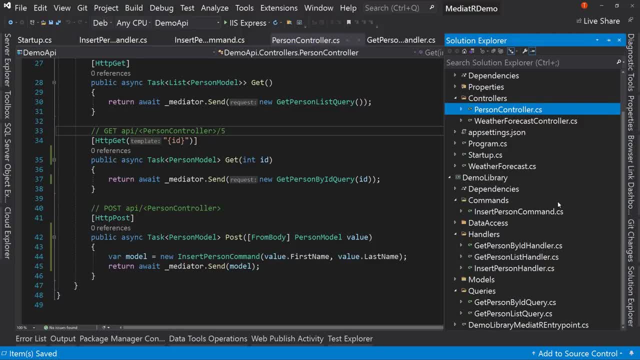 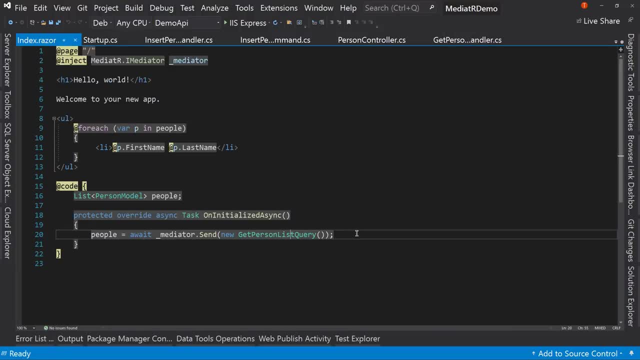 But at the same time, if we look over in our blazer, it's no different, Because in our blazer and our pages, when we said, hey, I need a list of people, I have this one line and I can start using it. 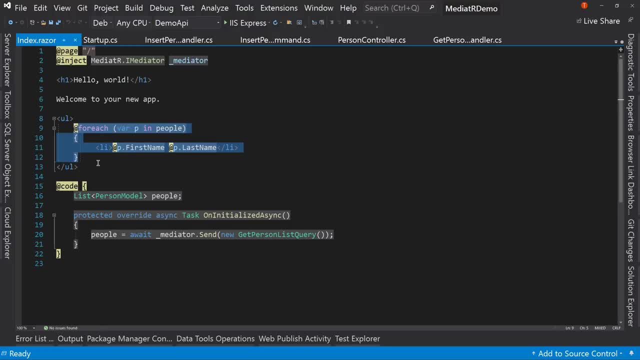 If we had an edit form here, the code for the result of the edit form is: just pass this data in. That'd be it. So a lot of stuff you can do is shift your responsibilities out of your user interface and down into a more testable location. 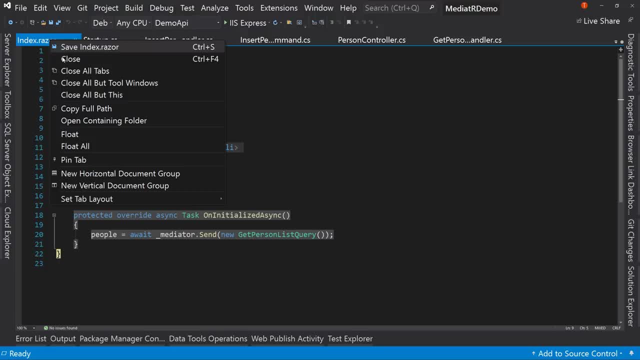 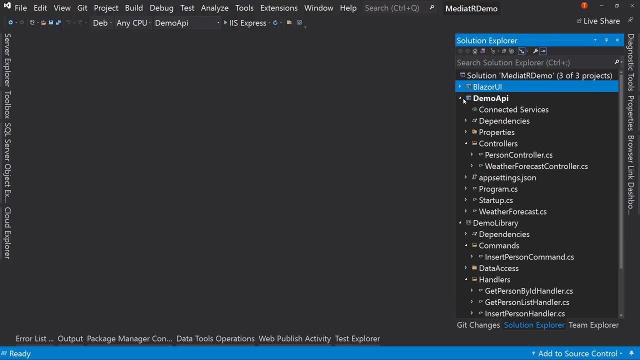 that is also then portable. If you notice, I swapped over from blazer to our API and didn't really have any changes. I just pulled my library, That's it. I said: hey, come along with me, Let's bring your handlers, your commands, your queries. 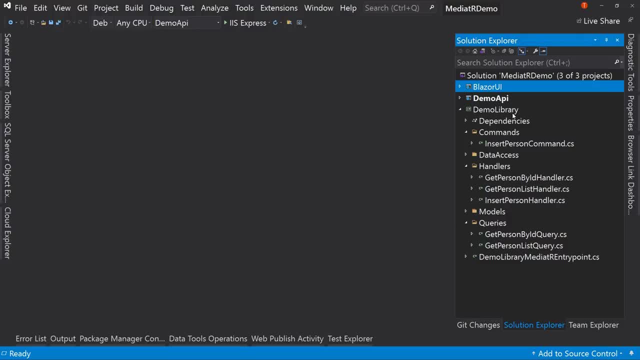 And now I can use it in a different user interface. So some pretty powerful stuff here, but at the same time, notice that even for this little demo, I've got a lot of stuff in my class library. So again, this is where. 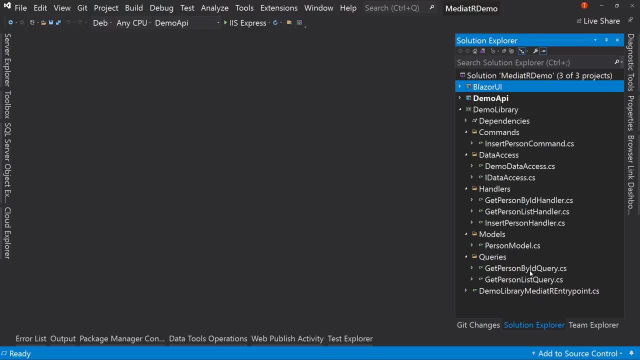 if you're doing a hello world project, do not use mediator. Where the tipping point is is gonna be based upon how big and complex your application is getting. As it starts to add complexity, that's when mediator will start to um have more benefit than drawback. 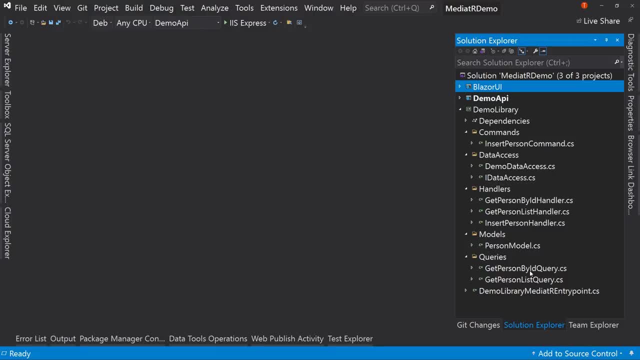 And that's kind of that balance, that balance you wanna hit on the teeter totter of you know how big and complex your application's getting, versus how much these patterns will help you. Now, note also, I just did one folder for commands. 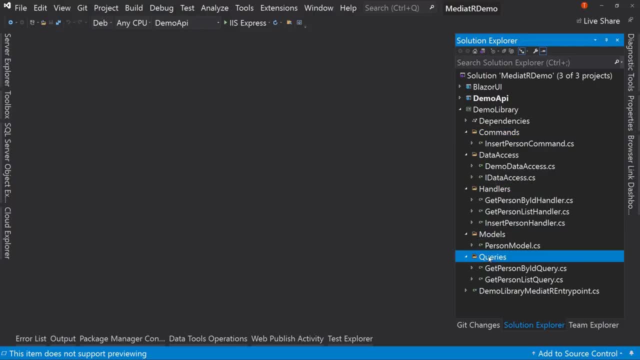 one for handlers and one for queries and even one for model. So for commands, handlers and queries, I might even break it down even further And say: well, for person, for people, I have commands, handlers and queries. 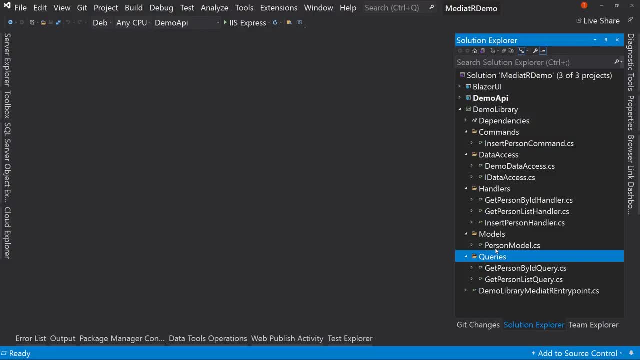 And then a different one for another- uh, roughly a table of data, you know, and so we have multiple of these sets of commands, queries and handlers. Again. that's as your com, your application, grows in complexity. that's when you need to start thinking about how to best keep things together. 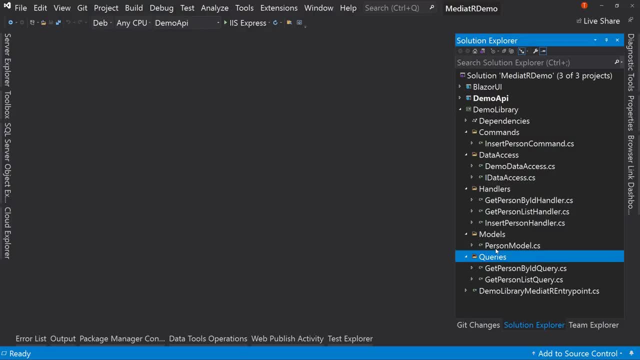 in a way that's. that's logical, so you're not hunting all over the system for implementations but at the same time, is not overwhelming with a number of uh folders you have to look into for your various things. Okay, So that's the mediator pattern. 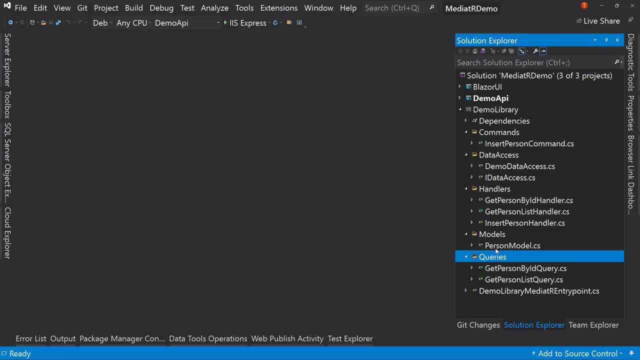 I would encourage you in a lot of ways not to use it until you grow a certain size. Don't just use this on every application you build. It's a shotgun for what sometimes is a tiny little problem you're. it's just way too big a solution. 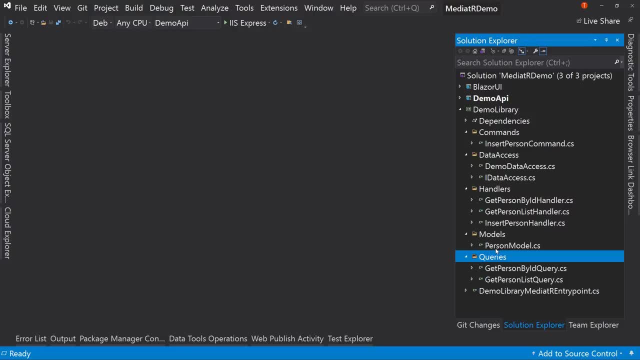 But for when you get bigger, this is a great solution to help you make things more testable, help you disconnect things that have it more loosely coupled. It even helps with um the idea that your depends injection is injecting so many things. 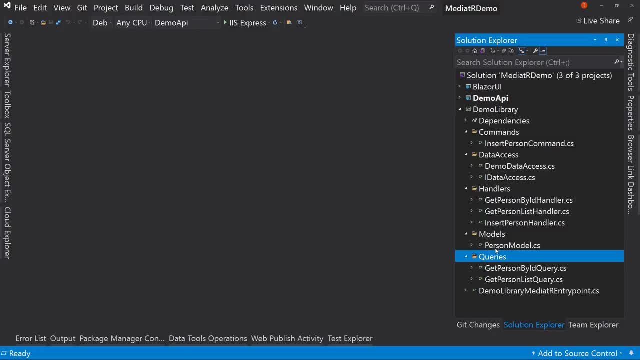 It has your classes have to know about so many different things. It reduces or eliminates that by just allowing you to depend on mediator and having your handlers do all that. Do all the rest. Okay, So that is the mediator uh system, which uses CQRS pattern and also the mediator pattern. 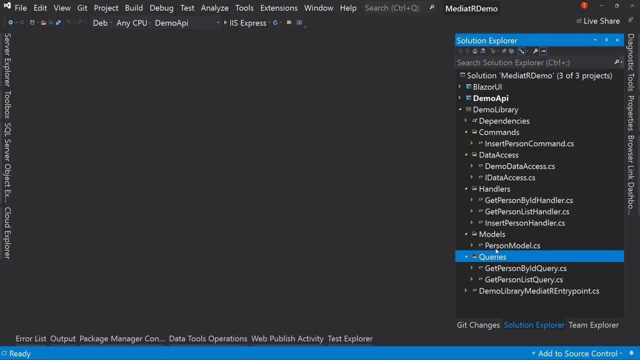 Uh, I hope you've enjoyed it. If you have questions, let me know down in the comments. I'm sure there's a lot more we can go into with this. There's a lot more complexity you can dive into, but I try to keep this as high level- as entry level- as possible for this intro.